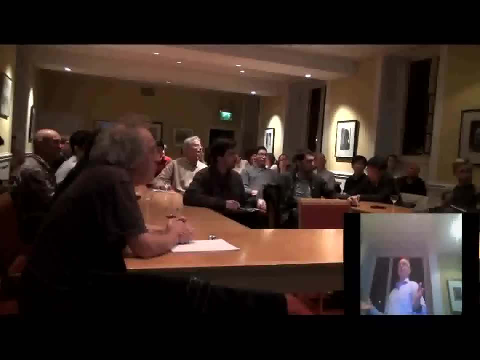 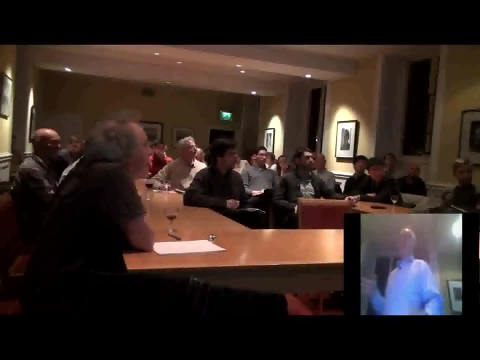 thanks for the invitation, and it's one thing I like that we can do. when there's disagreements within the non-Orthodox crowd- dare I call them neoclassical, non-neoclassical- we actually talk to each other about it, which is one of the pleasant things about our side. 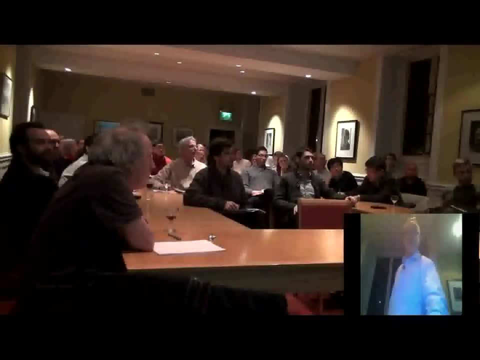 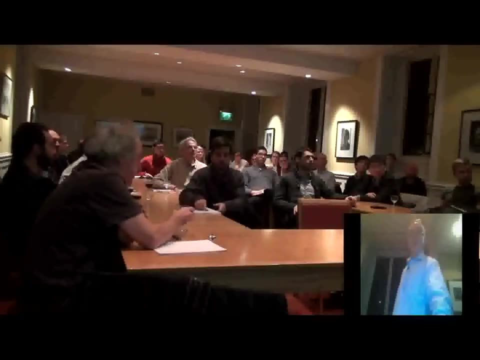 of the debate. It's not a case of wanting homogeneity all the way through. So I'm going to be defending mathematical modelling, but what I'm going to be saying is mathematical modelling in economics is a means of criticism, is a tool of logic, and is what I think it. 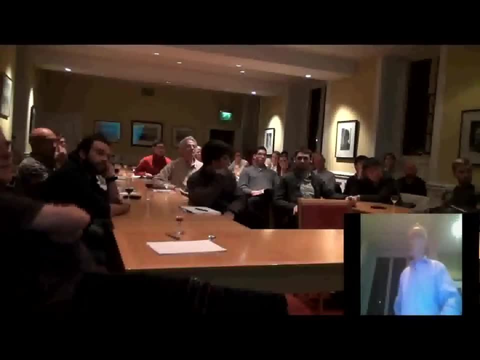 should be and why I think it's necessary, even for people who oppose it. It's unavoidable, which is a conversation I had earlier today with a lot of people in the audience. and I think it's necessary. even for people who oppose it, it's unavoidable, which is a conversation 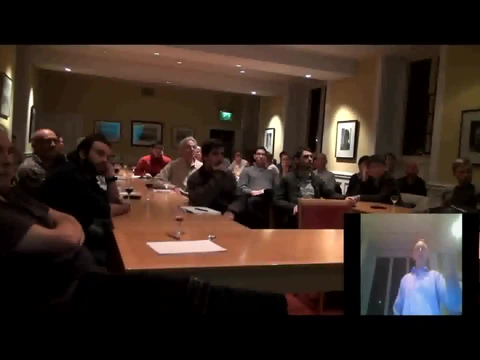 I had earlier today, and I think it's necessary, even for people who oppose it, and I think what I'm not defending is the modelling that's been done by—and I'm going to use the word neoclassical. it's fine Tony being here. that was because he is here—mathematical. 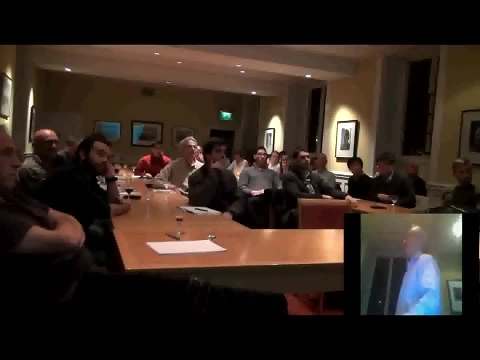 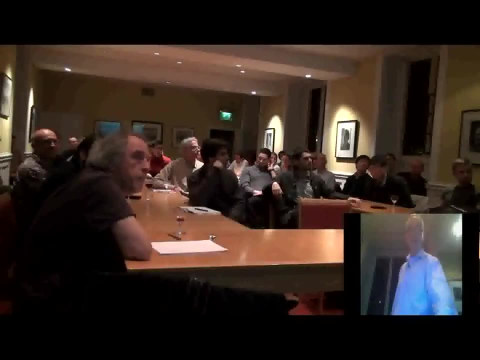 modelling by neoclassical economists in the main, and this is what it has been and I think why it's damaged economics, that a very different perspective on why that mathematics and in the hands of neoclassical economists has done damage. 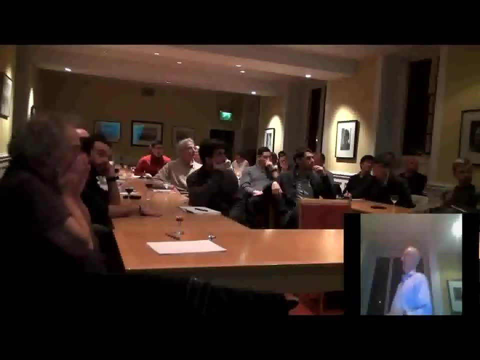 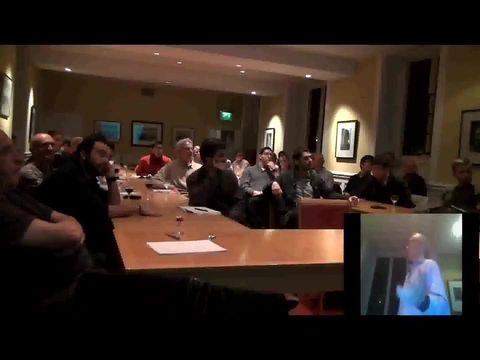 And, in a nutshell, one of the chapters in my Debunking Economics of type. it's titled: don't shoot me, I'm on the piano. That means people are like like who knows where? reference for that. or who doesn't know the song? reference for that. okay, Elton. 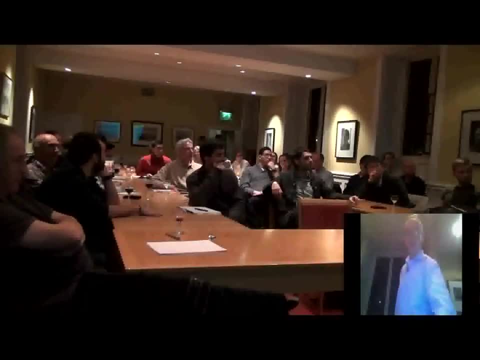 John, one of the one of the songs, one of his famous albums. don't shoot me. I'm on the piano player and my argument is: well, mathematics is the piano and when you get lousy tunes out of it, you should actually shoot the piano player, don't. 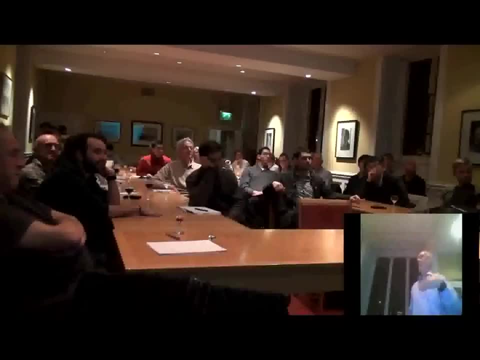 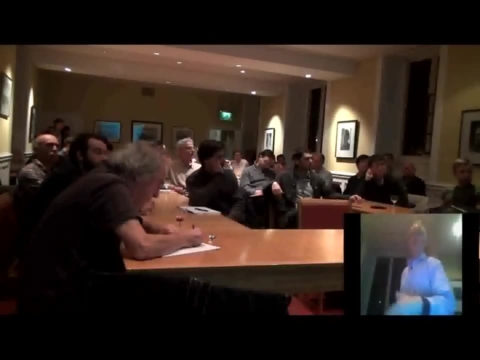 shoot the piano. so, as a means of criticism, if you look through the literature- and this is something I had to do after I did my undergraduate degree, of course, because you didn't get this stuff covered in their normal textbooks- but you can find an enormous number of fundamental critiques of 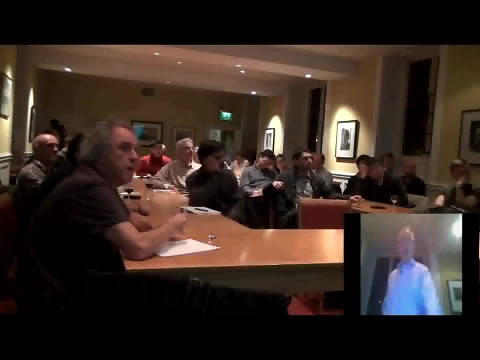 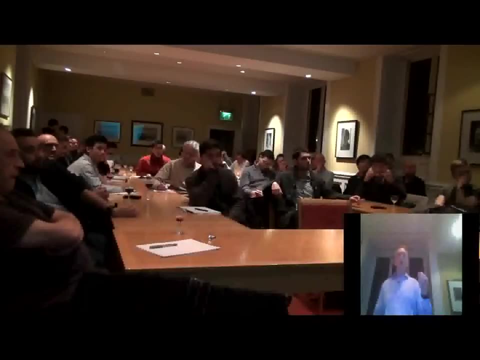 neoclassical theory, all of which use mathematical logics as an essential part of their critique. so Shraffa was probably the first, one of the first really advanced technical critique of neoclassical economics, and what he argued was that if you look at how the marginal productivity theory of income 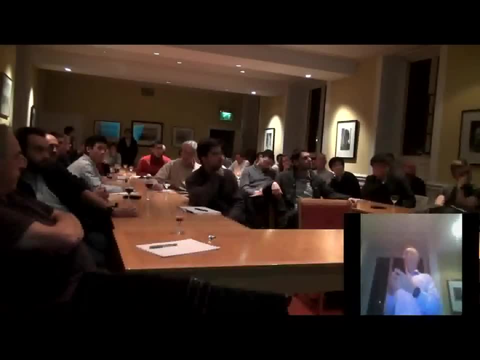 distribution, which is essential part of neoclassical theory if it, since the days of JB Clarke, argued that the return to wages, the labor, was a return for the marginal product of labor and the return to capital was the marginal product of capital, in both cases arguing an increasing amount of the. 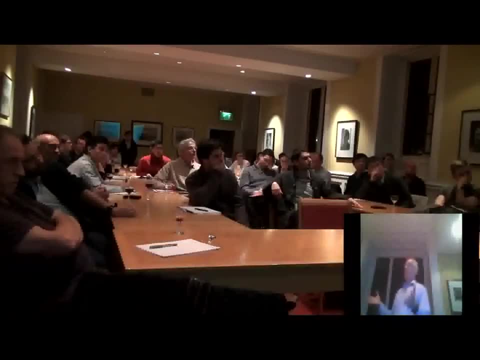 input would mean a lower rate of return. now that mean you have to measure it accurately. and Shraffa argued: yes, you can measure labor within reasonable bounds. you can measure unskilled labor. you can use multiples for skilled versus unskilled. that's not difficult. but when you add up capital, how do you do that? 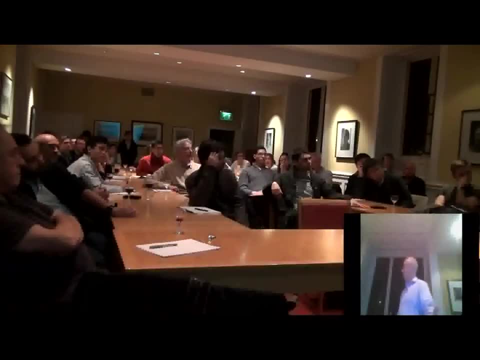 how do you add- speaking of my technology here- a portable recorder to a laptop computer? how do you add them together? together? well, neoclassical say: no problem, they ignored the ontology. let's just add up the numbers, we get in the statisticians and then still use that as 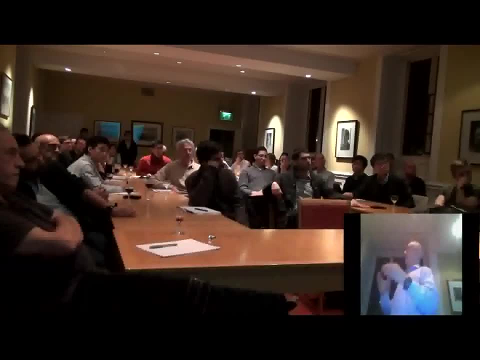 an argument for the marginal productivity theory. Shraffa said no to really add up heterogeneous capital. the best method is to reduce that capital to day-to-day labor. so you say today's capital is yesterday's machinery. plus the work that was done to make it into the machine it is today and vice and so. 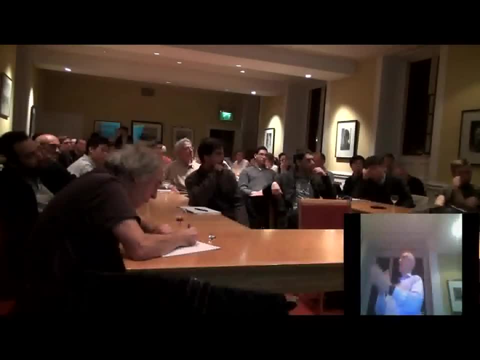 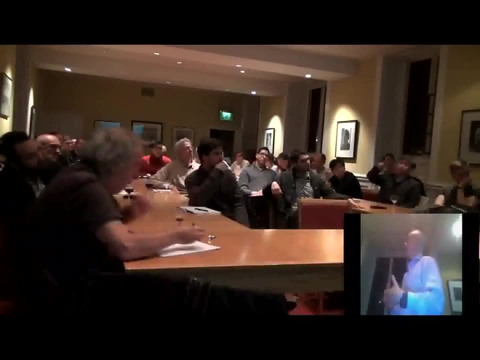 on. you keep them going back in time and reduce them as much as you can. the capital component, to have a series of terms in dated labor, when the labor was applied to producing something, and then you get a measure and when you do that you've got a very complicated expression for the amount of capital you measured which depended upon the rate of profit, a highly nonlinear function and that meant that, rather than the rate of return of capital- depending on how much capital there you measured, that you had the measure you had the amount of capital actually depended upon. 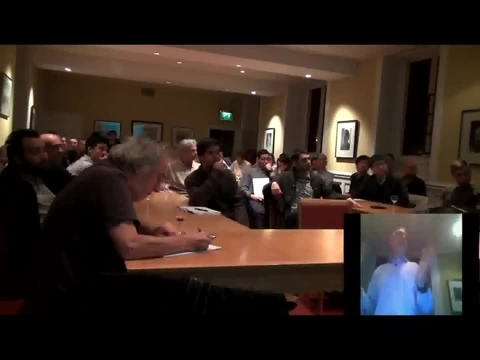 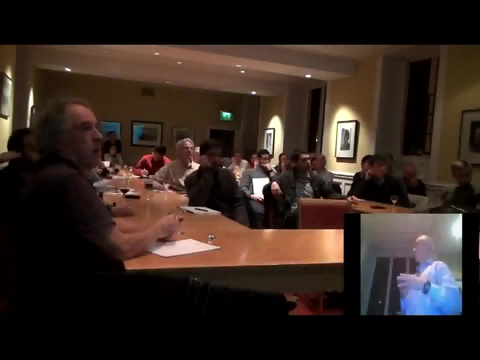 the rate of profit in a way you simply couldn't reduce to the the same, relatively simple adding together of workers to work out labor input. so that is a major mathematical critique of neoclassical economics. one you might not have heard of is what's called the dual stability theorem. when 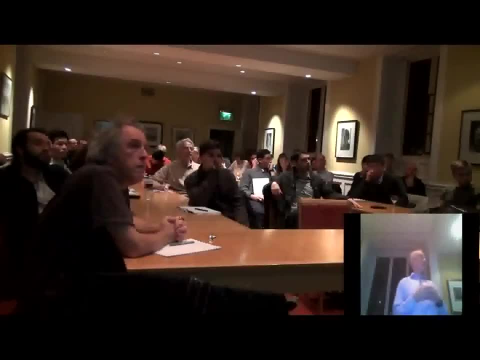 you look in the literature, it's actually the dual instability theorem. and these three- the two names- are the ones that are most associated with the Jorgensen and McManus. I think Black does a far better job of explaining it and pointing out its importance in his neglected but, I think, extremely important book. 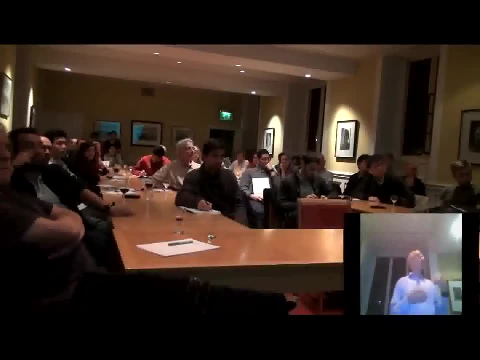 economic economic systems of post Keynesian approach, written by a professor of applied mathematics and that's took a look at the stability of general equilibrium. and if you take a look, if you, if you reduce any production function to its various components, the one that determines the stability is the. 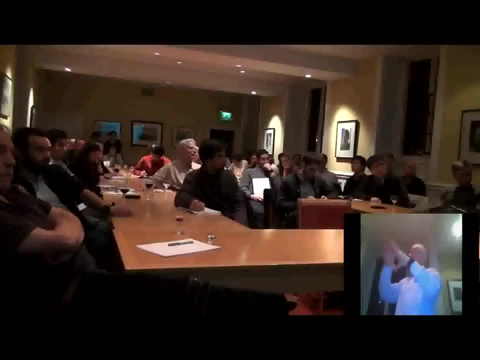 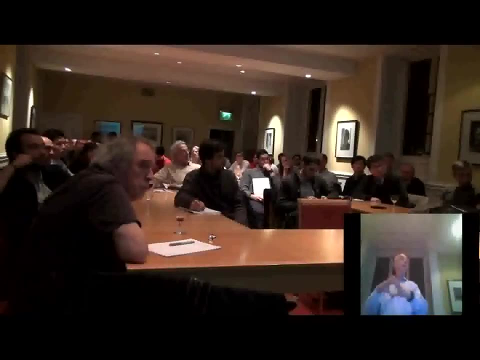 linear component and that's what gives you a input-output matrix as your very first measure of the structure of any production function. and when you have multiple commodities being used to produce multiple commodities, you get a square matrix where all the terms are either zero or greater than zero and, according to the Throne-Trobenius theorem, the what's 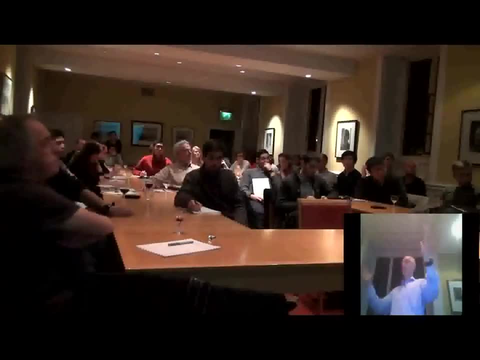 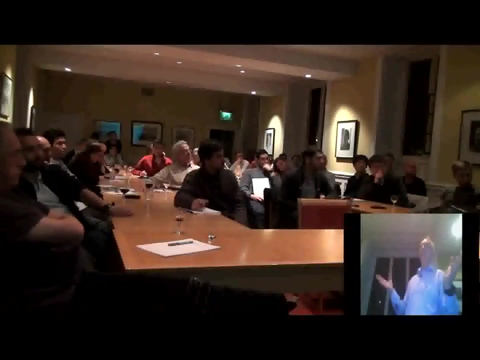 called the dominant eigenvalue, the term which tells you whether the matrix as a whole expands space away from equilibrium or contracts it towards the dominant eigenvalue, is greater than zero, which means that, well, that has a dilemma for neoclassical economics, because when you work out general equilibrium, as they 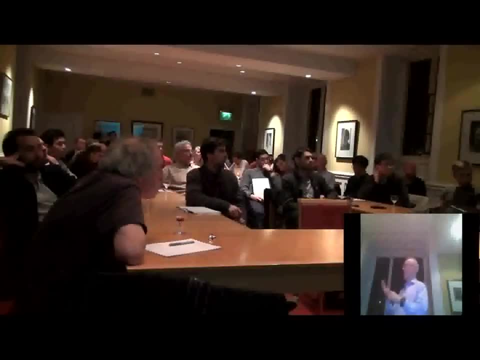 used to call general equilibrium, which is multiple commodities producing multiple outputs and trying to reach an equilibrium price vector, which would therefore mean no change in relative prices, and an equilibrium level of quantities of output, which mean quantities all grow smoothly through time. you need that. if you done, either you're here those cases applying and not 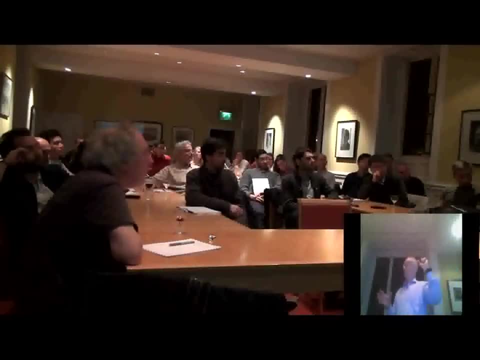 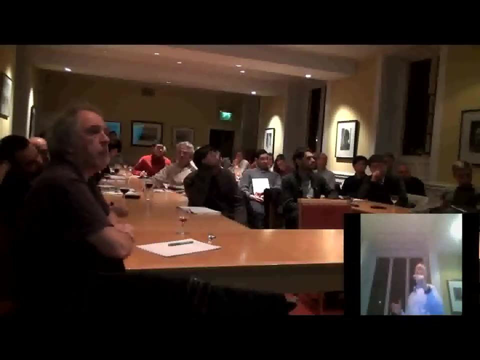 in general equilibrium. the matrix determined the dominant eigenvalue for production, so the vector of quantities. but the inverse of that matrix determines the dominant eigenvalue for prices. now simple thing about matrices: in their inverts, aji o, that matrix determines the dominat eigen value for prices. now, simple thing about. 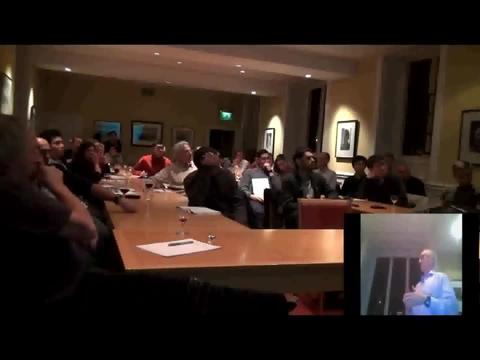 matrices, in the inverse or quantity they're going to take, the proportion that larger or more vaporiousат versus if the dominant eigenvalue of 1 happens to be 0.01 and the dominant eigenvalue of the other is 100.. That means that even if you're working in discrete time where the 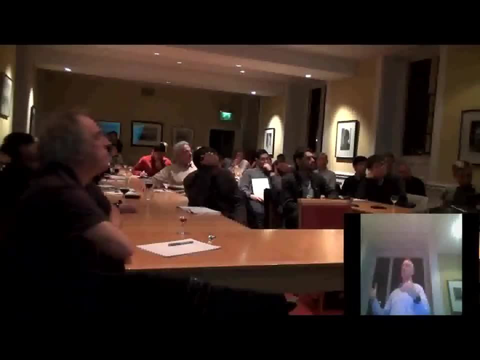 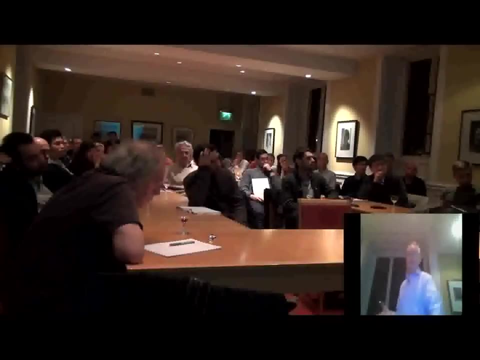 important value for that eigenvalue is 1, one of them is going to be massively greater than 1.. So necessarily either the quantity vector or the price vector will be unstable. But they call it the dual stability problem. It's actually a dual instability problem. 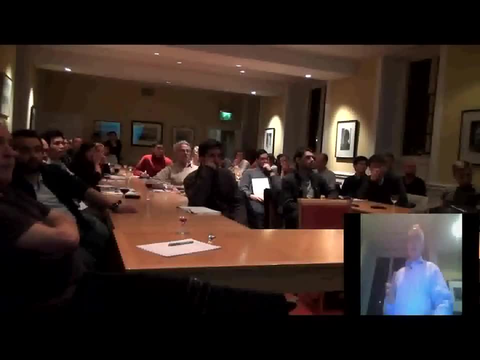 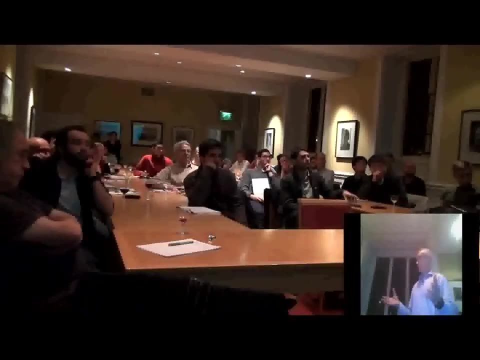 And that meant that general equilibrium can't be created. That classic sense of seeing a way of reaching an equilibrium price vector and an equilibrium set of quantities, which was Walranz's overall aim, was impossible. It couldn't happen. You couldn't have an equilibrium. 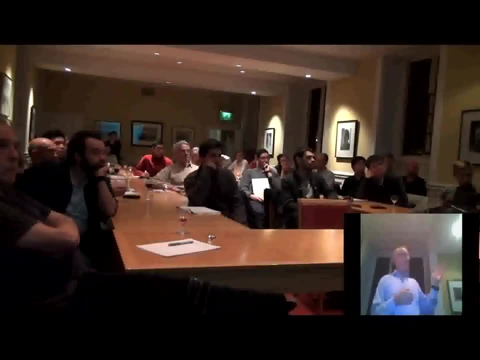 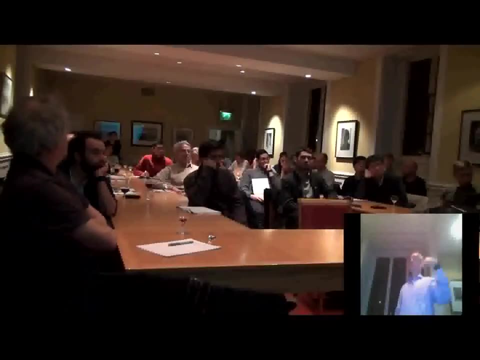 vector of prices and an equilibrium vector of quantities in the same system. The one that I think is most important, and one you may know, is Sonnenschein-Mantor-Lebreu. That says: let's imagine or let's pretend you have an entire unit of the equilibrium. 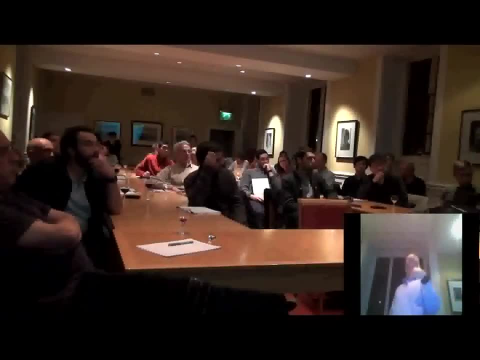 universe populated by individuals, all of whom have the classic neoclassical downward sloping demand curve. They've all got Hitchin compensated downward sloping demand curves. What happens when you add them up? Do you get a downward sloping market demand curve? 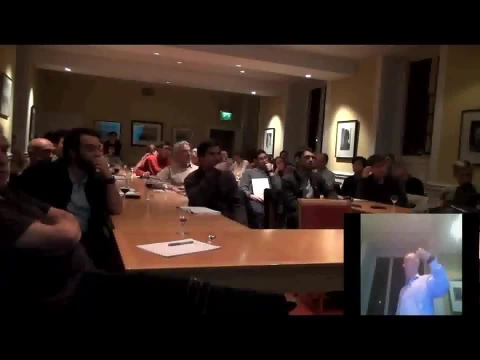 The answer was no. The market demand curve formed by adding up the demands of perfectly neoclassically rational Hitchin compensated demand curve. individuals can have any polynomial shape at all. So that says even market supply and demand analysis can be done is not justified. So those are three incredibly powerful critiques of 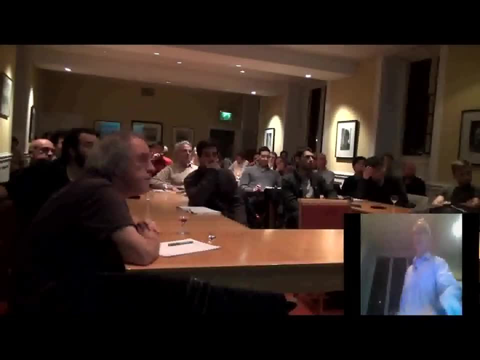 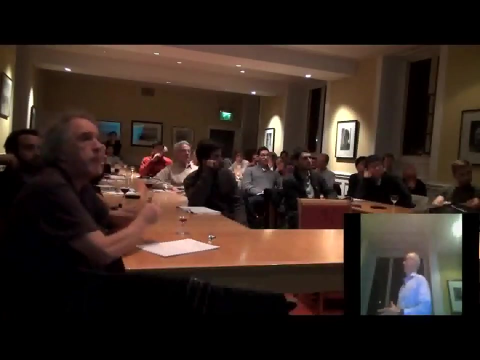 conventional theory and if there was genuinely a mathematical discipline. the reaction to those three discoveries would first of all be: well, you can't have a master of productivity theory of income distribution, because that depends on being able to accurately measure capital and have a nice simple relationship between the amount of capital and the rate of profit. So profit. 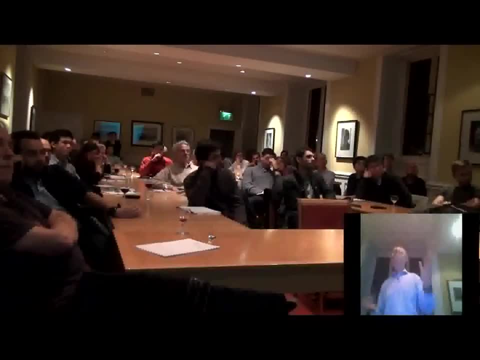 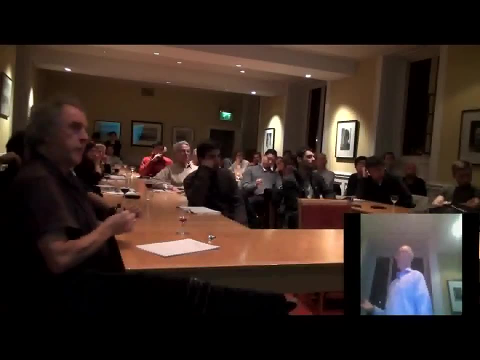 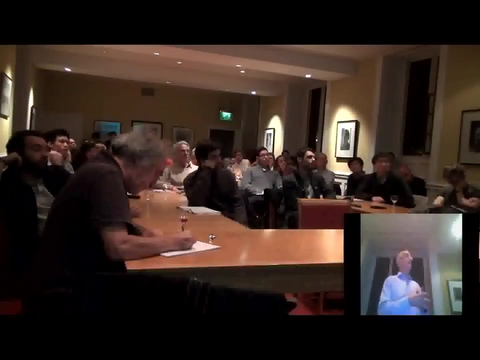 has to be a surplus. You might be able to have wages in some sense reflecting some contribution, maybe, but profits got to be a surplus, which is what the classical theory argued before them. You then have to also abandon methodological individualism, because if you can't reach equilibrium in a well-specified model of 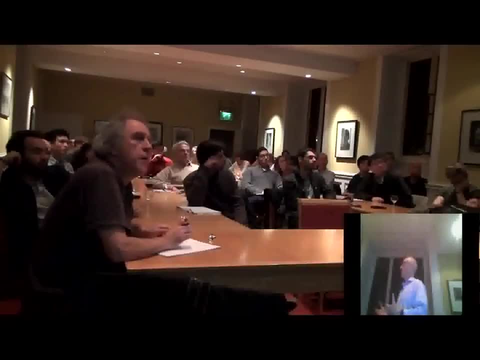 production, then prices and quantities have to be set in a non-equilibrium way. so there goes equilibrium and you have to also abandon methodological individualism, because if you can't even get the market demand curve out of individuals who have all got that downward sloping individual demand curves, then you can't even do supply and 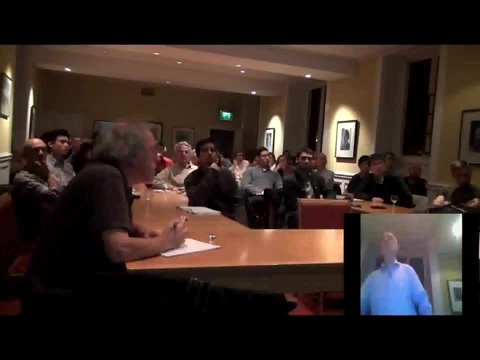 demand analysis. Now, those are very, very strong results. May I ask a question? Yeah, sure, yeah. What do you mean by a mathematical reaction? You mean the reaction that doesn't abandon the mathematical. If a mathematician had derived those results, the reaction would have been: well, that theory can't work. You've got to find a. 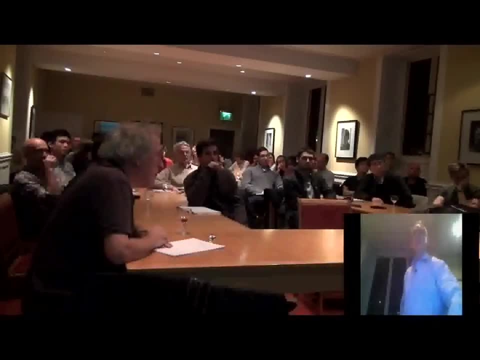 replacement theory In mathematics. In mathematics, That's a mathematical reaction. Yeah, Okay, Can I ask you what you mean by a new classical? It's derived from the util, the Volra, Jevons and Marshall tradition, which sees methodological individualism as an essential part of how you proceed, which sees 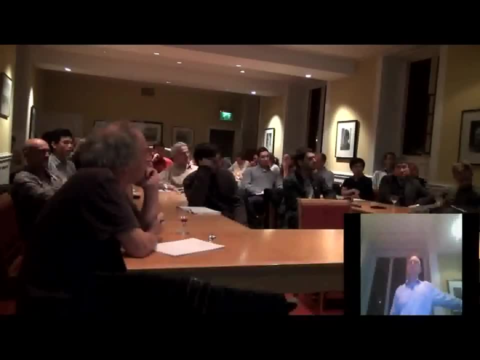 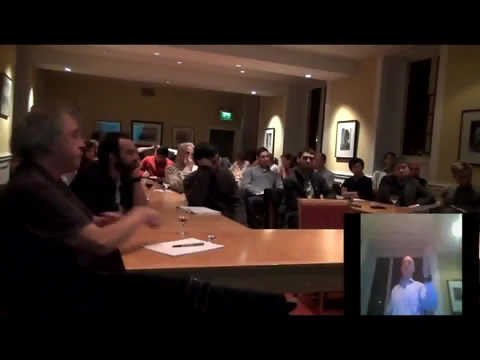 individual consumers as being utility maximising, individuals firms being profit maximising and the belief that you can reach an equilibrium system of prices and quantities out of that system. So I see, really it's the Marshall, Volra and Jevons tradition which has been transformed numerically. 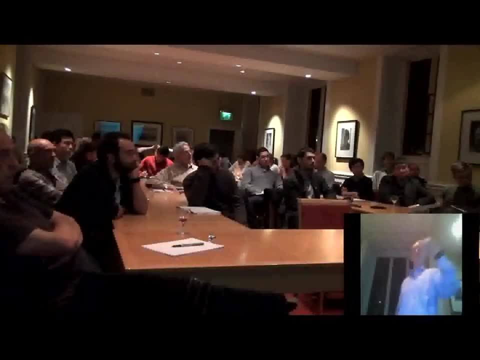 numerous times, but in this case I agree with Giannis Varoufakis- those elements: if you don't have individual methodological individualism, if you don't have methodological equilibrium, and if you don't have a meritocratic income distribution story as well, then you don't. 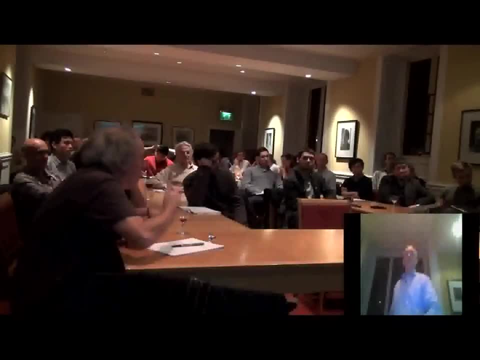 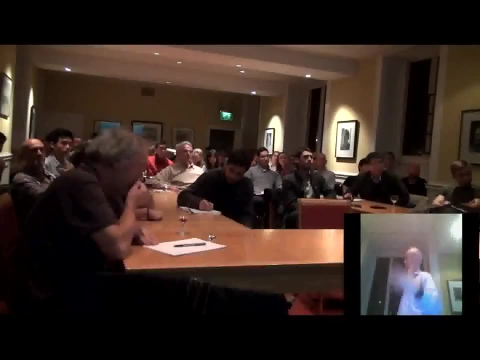 have neoclassical economics anymore. Okay, I mean I'm happy to come back. but Yeah, come back to that. Now what's the actual reaction of neoclassicals being ignored a lot? They still have the Marshall productivity theorem in how they explain, certainly in undergraduate. 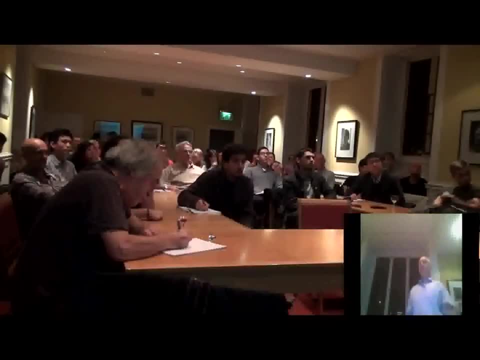 and also how they explain, Yeah, how they think at the level of so-called advanced theory. They still assume equilibrium, though the nature of equilibrium keeps on changing radically. DSG equilibrium is completely different to what was the norm for the computable general equilibrium fad of 30 or 40 years. 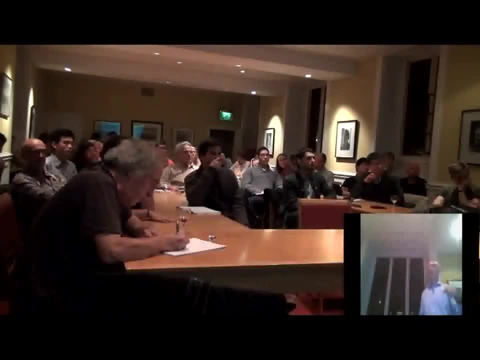 ago, but it's still equilibrium. It went from CGE to DSGE. We didn't go from CGE to DSDD for dynamics. They're still stuck with the equilibrium belief of how about? one must do the work. but where did that go and how did they improve the rates of? 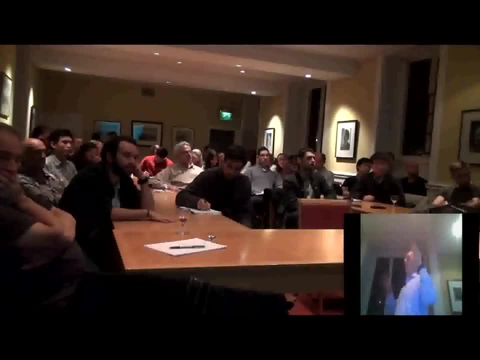 And so you get at the level of the. So you've got- And that was a really really good explanation for the A little bit more detailed explanation of what you said there. you know Right, exactly, yes, You've got a. 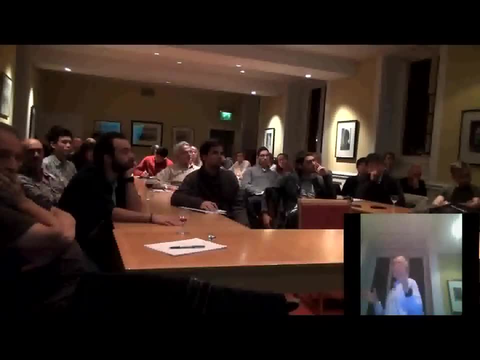 Well, I So the For Universal equilibrium. I guess the idea, Yeah, is that you've got a, Yes, that there's a, There's a widest clinical probability on that matter, and that the number of people. 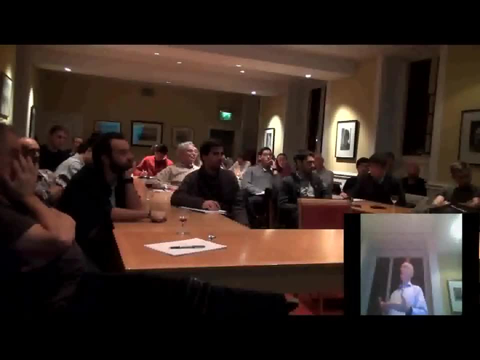 who do You know? you've got a. I've got a lot of- I mean I was thinking a little bit about that just a minute ago- about I mean actually, I'd actually say you know, for example, people Yeah. 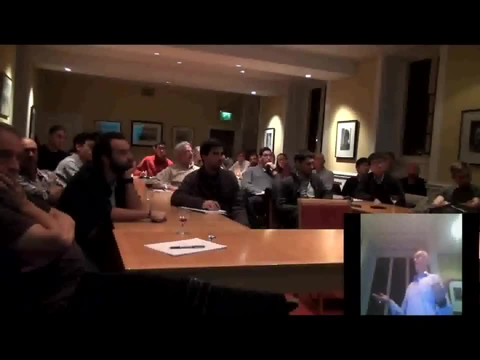 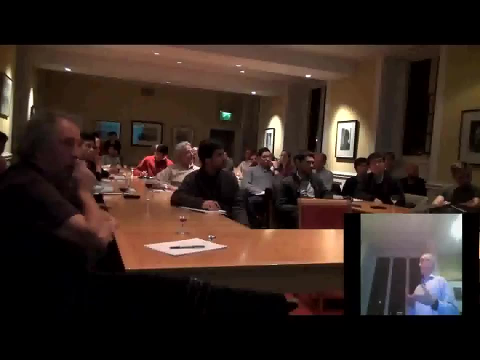 Instead, we have to work at the level of social groups that have some coherent behavior, which is social classes. In other words, I think the neoclassical agenda, when you look at it seriously, has proven the classicals were right. 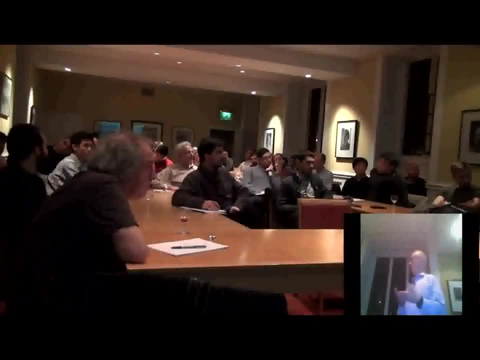 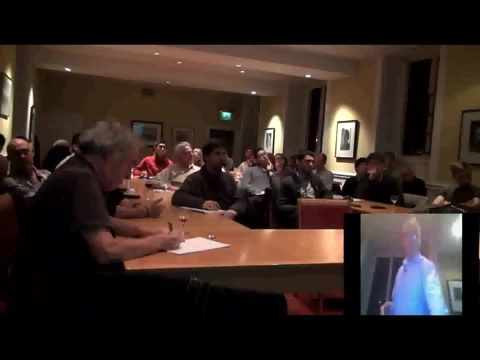 You have to have social classes, you have to have capital as a profit, as a surplus, and you have to have dynamics. That's what the proper reaction should be. It's the opposite of what they've done. So I see them as fundamentally anti-mathematical. 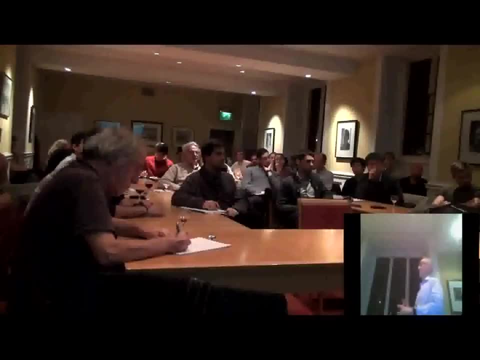 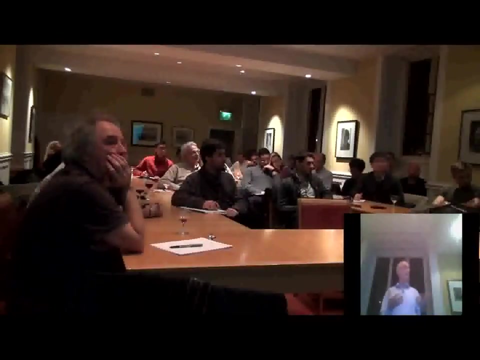 And what's driving them isn't mathematical logic, it's a set of conclusions they wish to reach. They want to prove that a system of isolated markets can reach equilibrium without any overall coordination. They want to prove that we live in the Pareto best of all possible worlds, where merit rules. 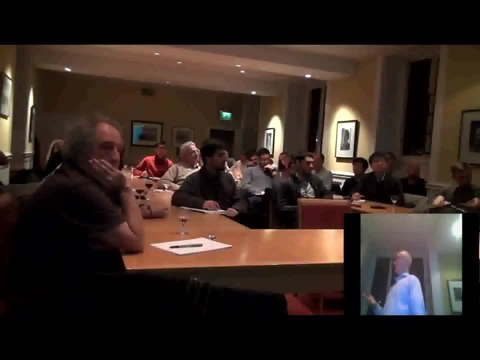 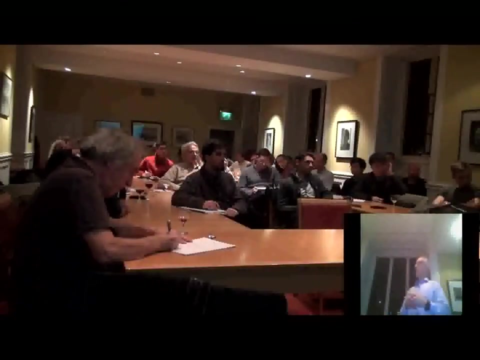 income distribution. They want to prove stability And rather than finding that out, they actually disproved all that. Sometimes own goals- The Seinenschein-Mantel-De Broglie theorem is a classic own goal- But the other thought by critics, as in the case of Schraffer and also Blatt. 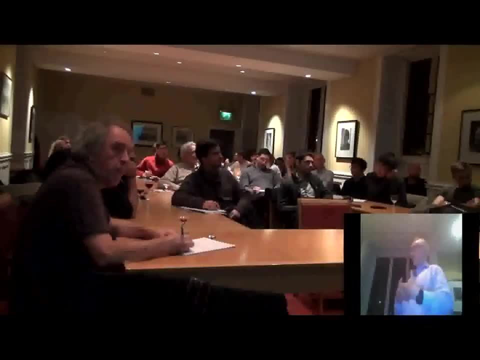 So, rather than reflecting upon those findings and changing the nature of economics to suit, they've stuck with those theological beliefs and ignored the results they don't like. So I see it as an anti-mathematical discipline, not as a mathematical one at all in the genuine. 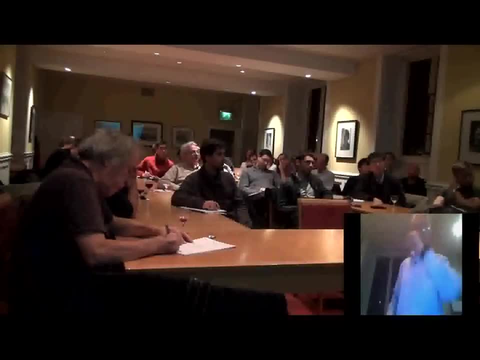 sense. Now, just giving you an example of that, I'm going to go through one of my contributions which is much simpler than any of the other theorems, And that relates to the model of competition, which is still taught in all first-year textbooks. 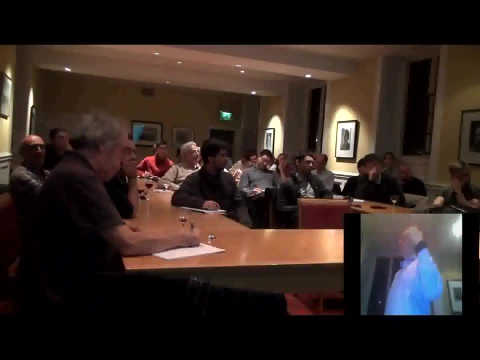 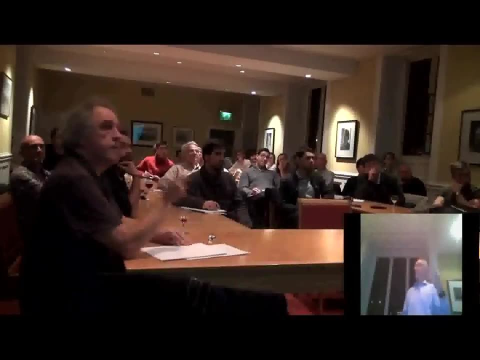 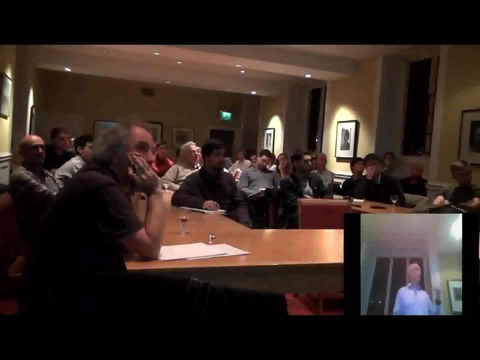 And unless we succeed in overthrowing it or continue being taught for the next century, the model they teach in first-year courses is mathematically false. That's the Marshallian model, Not Cournot and Nash's mathematically consistent. There's no errors in the Cournot-Nash proof of perfect competition. 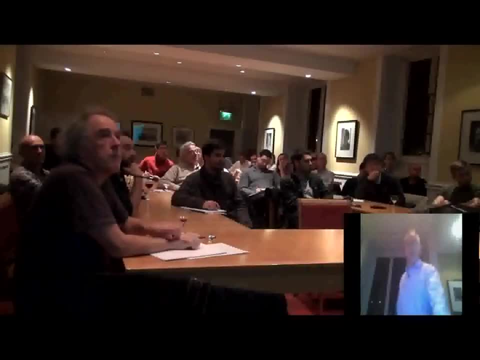 It doesn't generalise. That's the problem And it's too complicated for them to teach as well. But the standard textbook model starts off with a model of competition. It starts off by saying you have a downward-sloping market demand curve, which is already known. 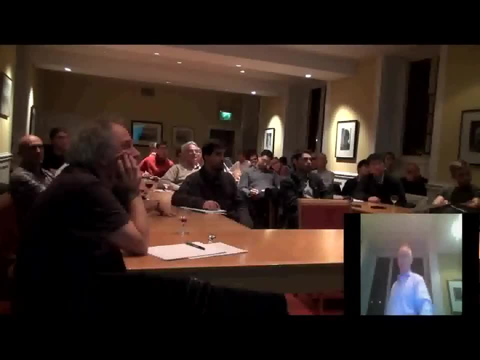 to be false, But let's start with that particular assumption. So you have the slope of the market. demand curve is negative, And then they also assume there's no collusion going on, nor is there any interaction. Firms just simply produce into the market. 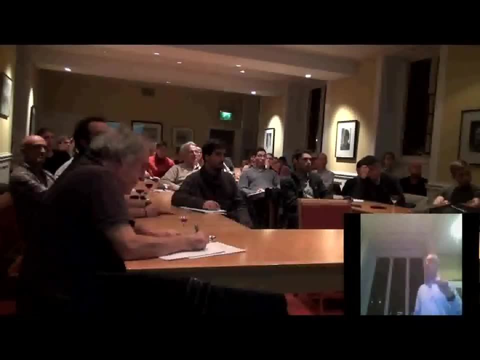 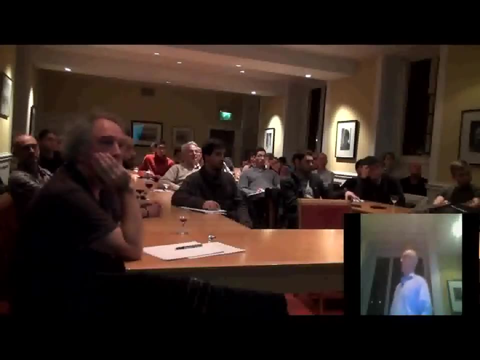 They don't strategically react to what any other firm does, And the theory asserts that simply because of the number of firms. the firms are prostatates And Mankiw. the way Mankiw was the textbook. I most love to hate him for its simplicity. 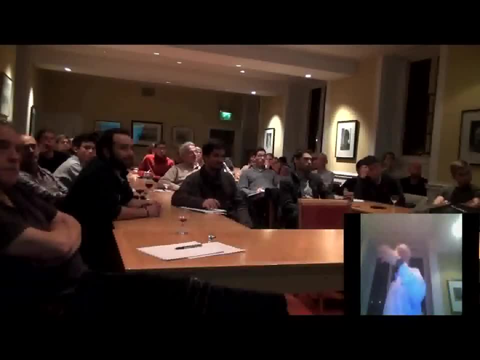 the way it's dumbed down, a pretty dumb theory. to begin with, he says a competitive market has many buyers and sellers trading identical products and so that, in other words, therefore, each buyer and seller is a price taker, which translates to saying that the demand curve. 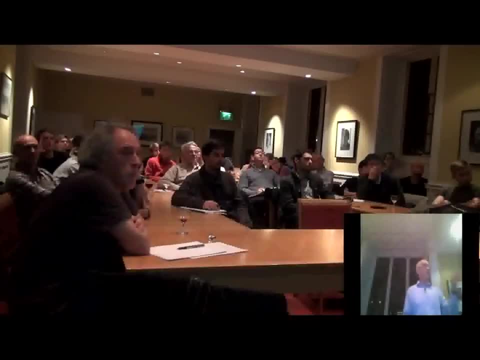 facing the individual firm is horizontal. So you look at the slope of the rate of change of market price with respect to a change in output by a single firm. that's zero. That's a large part of the instruction that all undergraduate students go through. 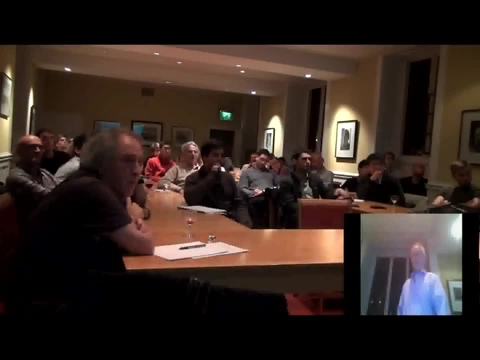 And it was proven to be mathematically correct. It was proven to be mathematically false in 1957 by, of all people, George Stigler. You go back and look at George Stigler's paper, which was an invited paper in the Journal. 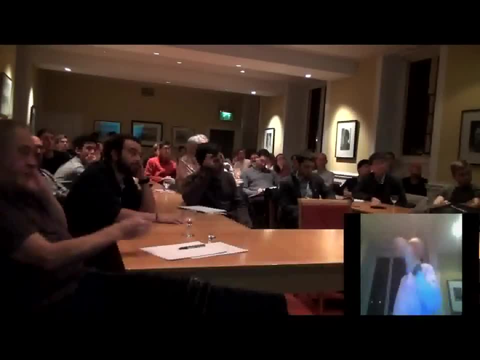 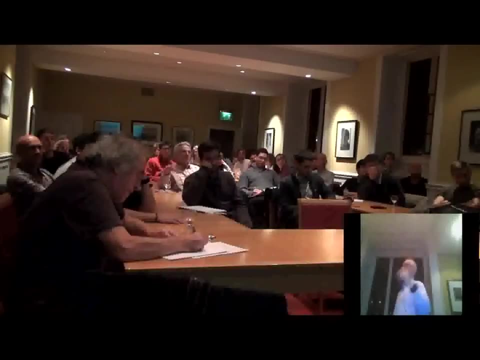 of Political Economy. As we all know, that is not political economy as we mean it- one of the most conservative and therefore prestigious journals in the discipline. They invited George to write a historical piece called Perfect Competition, Historically Contemplated, And he simply applied the chain rule to say that the firm's demand curve is the market's. 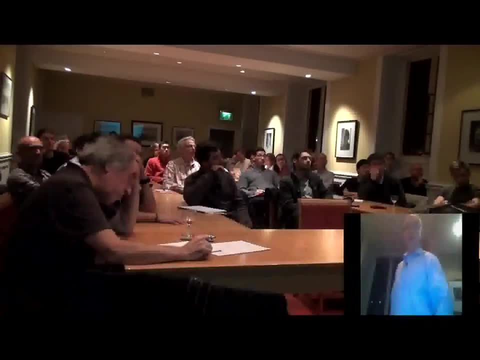 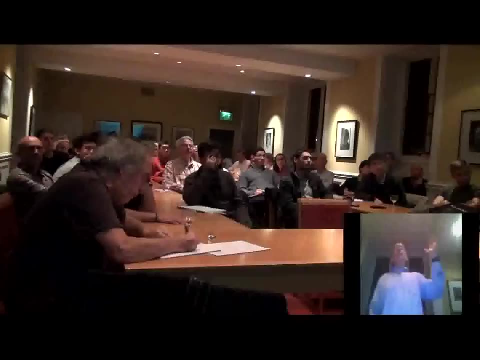 demand curve times. the market's demand curve, It's the slope of the market's demand curve times. how much the market output changes given a change in output by a single firm. So you simply do this little piece of simple mathematics. Slope of the individual firm's demand curve is the slope of the market demand curve times. 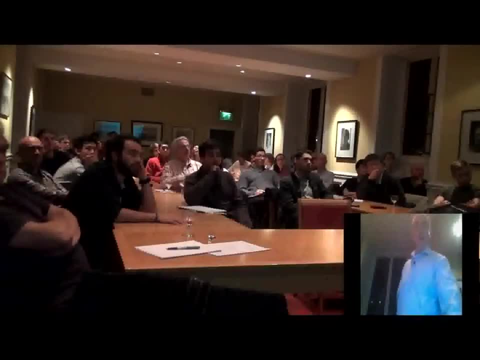 how much market output change is, given a change in output by a single firm. What's the value of that? Well, Stigler's Maths, hence the journal, and this is a particular footnote 31,. if you take a look at footnote 31,, he says that the slope, the change in a market output given a change, 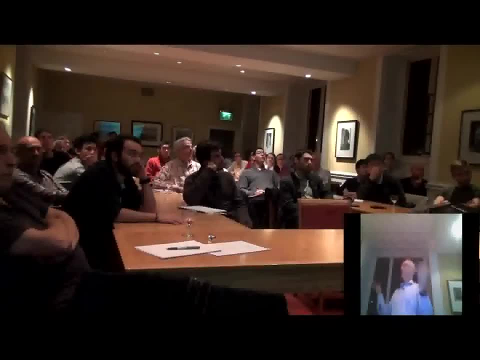 in output by a single firm is one which is basically saying that one firm increases its output and the others don't strategically react, then the market output increases by as much as that firm increases its own output. That's all it's saying. So that means you can then throw out that expression and say that the slope of the individual 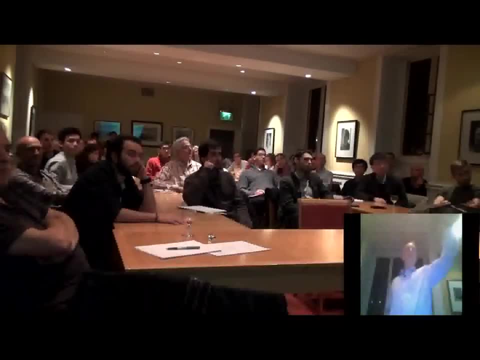 firm's demand curve is the market demand curve times the big 2d, little q, which is the market demand curve times one, which is the slope of the market demand curve, which is negative. So the slope of the demand curve facing the individual so-called competitive firm is its 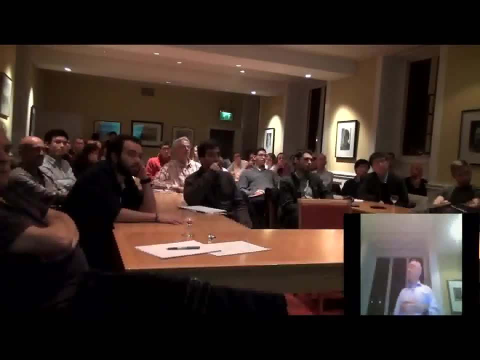 exactly the same as the slope of the market, demand curve. So under Marshallian conditions, there is no such thing as perfect competition. Now, that's not exactly what Stigler wanted to prove, as you can imagine. I think he was trying to be a bit elaborate and clever here, and, oh shit, there's a hole. 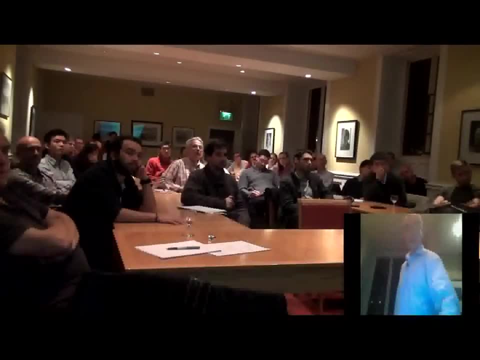 in my foot. Can I fix it? Well, he thought he found a way out, and that's what the footnote actually is on about, because he said, as you added more firms to the market, you converged to perfect competition. So he said, it's intuitive. 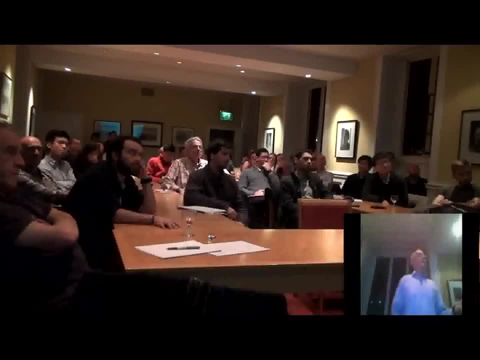 Intuitively plausible. That's a phrase I often see on the interclassicals making an outrageously wrong statement. With infinite number of firms, an infinite number, I like that one too. all monopoly power disappears, and you then get this result. 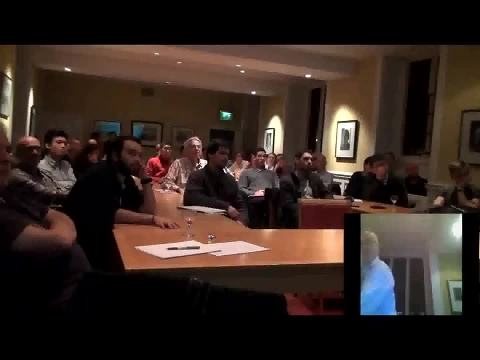 He says a simple demonstration: if sellers are equal size, all you've got to show is this: discretion is true, and that's saying Marshall: revenue equals price plus price divided by the number of sellers multiplied by the market elasticity of demand. Now, this is a mathematically accurate, true statement. And that term goes to zero, as the number of sellers goes to infinity. Quite true. There's only one problem with it. It would be mathematically correct about what would happen in competition as well if firms set output by equating marginal revenue and marginal cost. 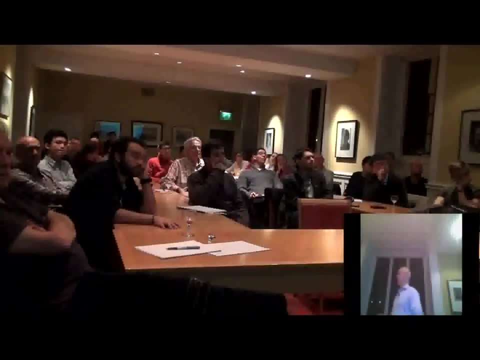 And that's what the theory says. they do because they say it's profit maximising behaviour. Only, it's not. It's provably not profit maximising behaviour. Let's look at that. They assume it maximises profit. this is what Mankiw says. 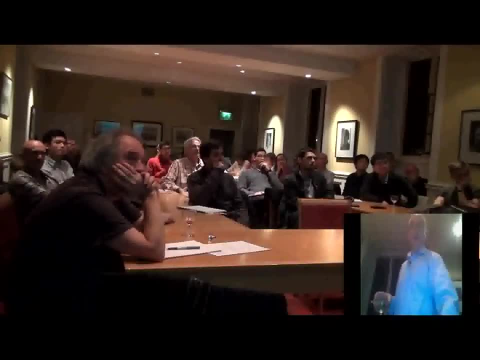 Profit maximisation occurs. Profit maximisation occurs, Okay, Where these two curves intersect. It doesn't, Because one firm's profit in an industry depends upon what other firms do as well as what it does. That's even even if it doesn't know what the other firms are doing, even if there's. 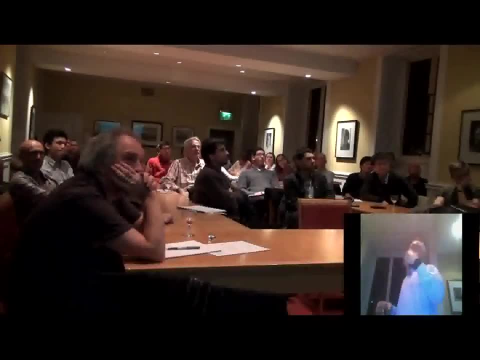 no collusion, simply because this is a simple mathematical statement. your profit depends on what other people do as well as what you do, So therefore, the true maximising profit point is not where you solve for this expression being equal to zero, which is the rate of change of your profit with respect to your own output. 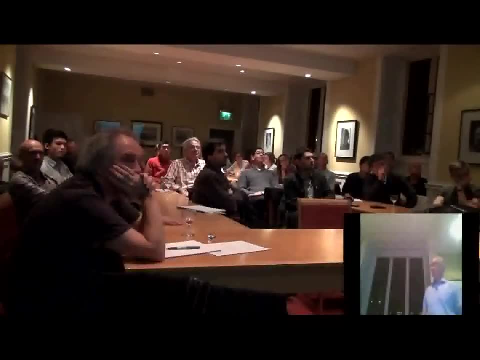 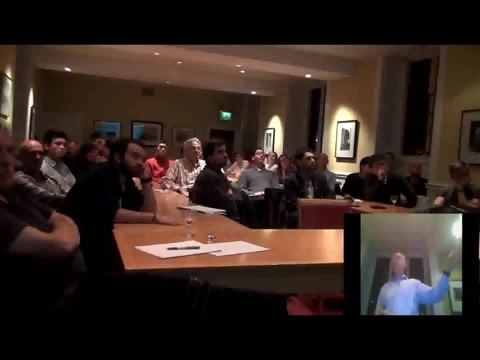 you solve for Q, where the rate of change of your profit with respect to total market output is zero. That's the true or not profit maximising point. Well, let's see what happens. when you work them out. What you find is, rather than that being the profit maximising function, 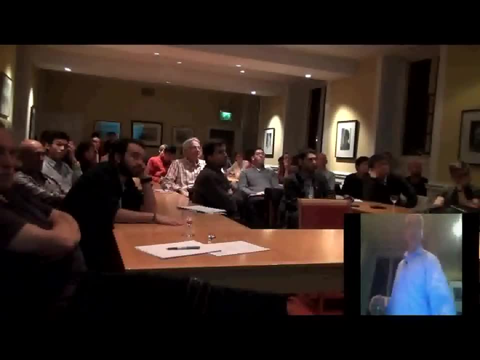 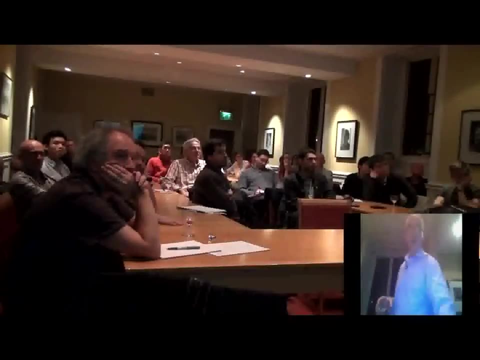 which therefore profit maximisers would follow, and therefore you'd get superless conversions. the actual answer is this one. Now notice the difference. It's not trivial because N's a big number. The neoclassical formula emits the number of firms in the industry as a multiplier of the second term in the expression. 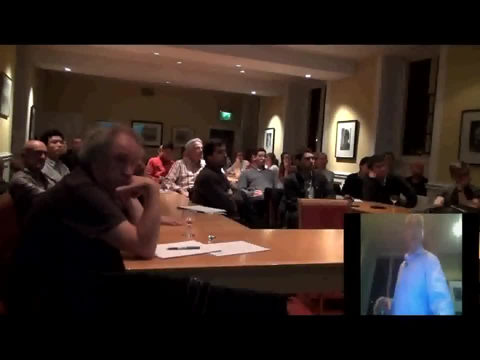 And therefore the neoclassical formula is only correct for the monopoly. Let's go through the logic of that, A bit of mathematics coming up. That's what you're trying to set to zero. That's the rate of change. pardon, the, you can't quite see the D of the differential there. but the rate of change of market, The rate of your profit. the profit of the i-th firm with respect to market quantity is the sum of the partial derivatives of the change in your profit, given a change in output by the j-th firm. of all the firms in the industry of whom the i-th firm is one, 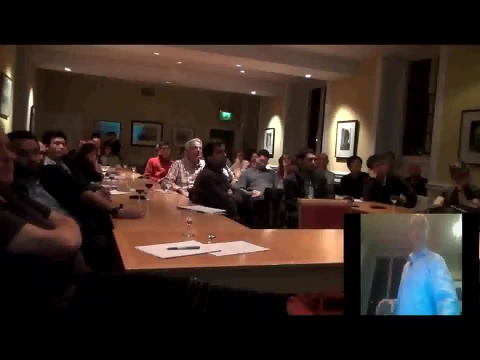 Let's take a look at this bit, That's saying sum over all firms in the industry. This bit is how much the profit of the i-th firm changes given a change in output by the j-th firm. And the final bit here is the inverse of what I've just shown as one under martiality and conditions. 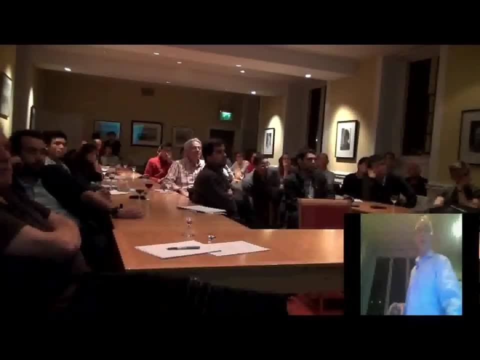 So you can just say that's one And expand this using the product rule. I'm just expanding the revenue part here. So the partial differential of the revenue of the i-th firm with respect to changes in the output by the j-th firm is P times partial Qi partial Qj plus Qi times partial Qj. 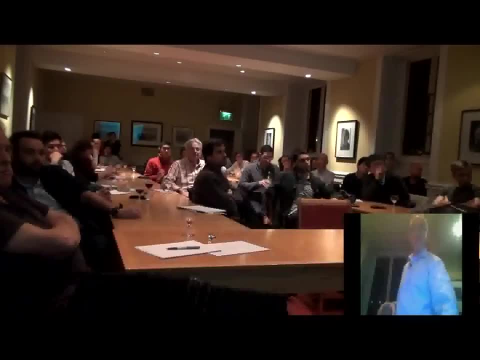 So that's one copy of P And the partial P part of the partial Qj. Now when you do that expansion, that is, how much does the output of the i-th firm change, given a change in output by the j-th firm? 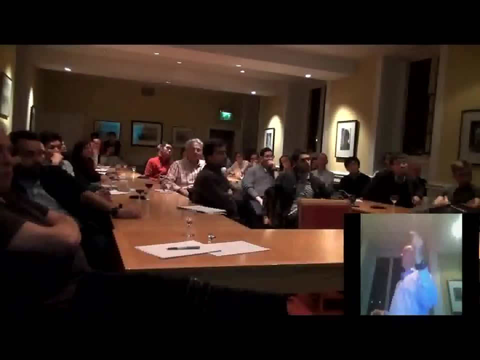 Because we're talking non-collusive behaviour. N minus one times that's zero, But once It's partial Qi. partial Qi, Therefore it's one. So what you get out of that is one copy of P. This bit here is change in the costs of the output of the i-th firm given a change in output by the j-th firm. 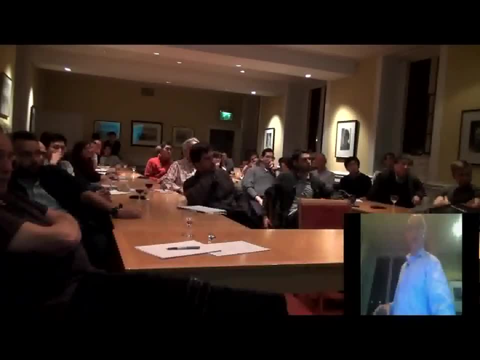 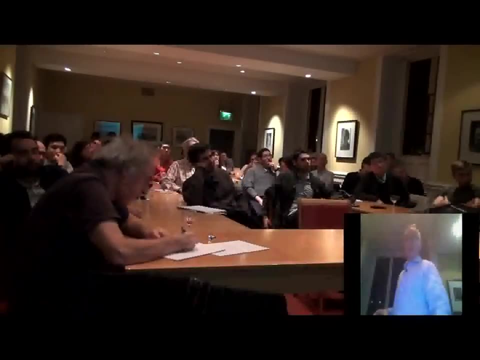 Again, N minus one times. that's zero Once It's marginal cost of the i-th firm. And this bit: here, as Figler has demonstrated, you can substitute the slope of the market demand curve for that expression. So what you get is N copies of Qi out of that. So what you get is the i-th firm maximises its profit where one copy of the market price plus N copies of the output of the i-th firm times the slope of the market demand curve minus marginal cost of the i-th firm equals zero. That's your true profit maximising formula. 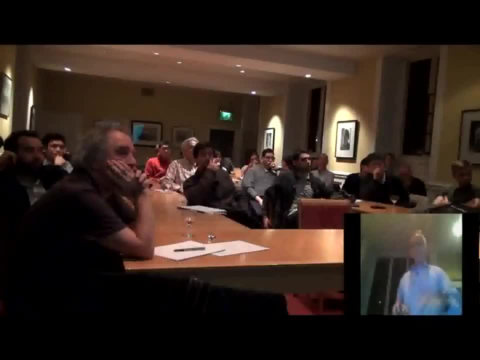 And if they're genuinely profit maximisers, that's the output level they'll choose. You rearrange that. That's where you get the marginal cost equal to P plus N times Qi, And that's what's left out of the neoclassical formula, which is wrong. 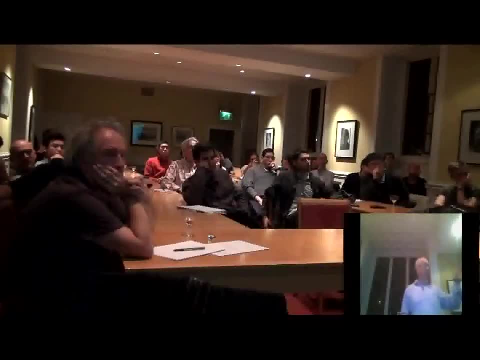 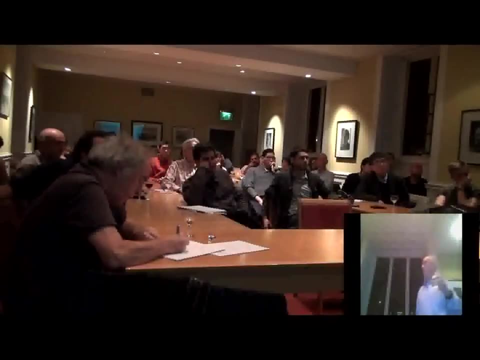 Mathematically false And there's a lot more to it. that's in that linked paper there in the Real World Economic Review And that's been rejected by a number of neoclassical journals, amongst others, Published in Review of Real World Economics. ultimately, 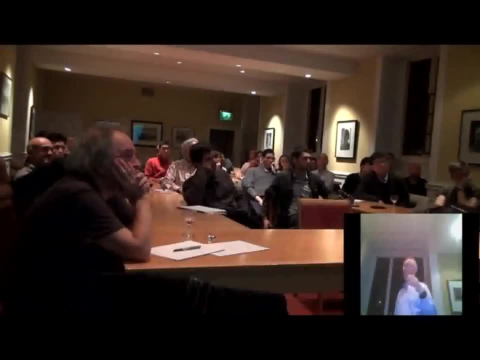 And one of my favourite rejections came from Robert Clower when it was submitted to the Journal of Economics Education. I know it's Robert Clower. He might as well have signed it. There were so many funny references to his work, it was ridiculous. 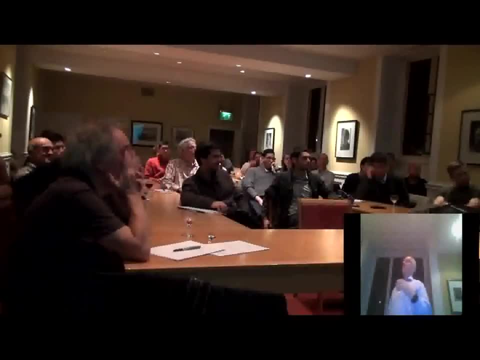 But in that he said George Stigler's attempts to. He said George Stigler's application of differentiation here is contrary to the spirit of Marshallian economics, Or something of that nature. I'll have to send you a copy, Tony. It's a good laugh. 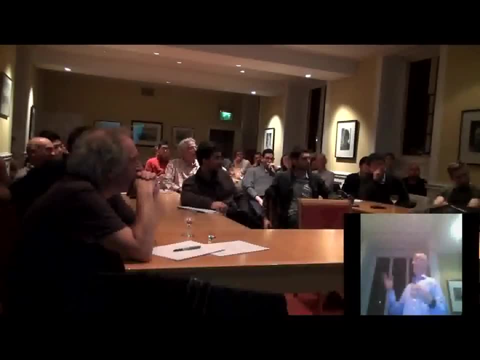 But he is a pretty progressive as they go, neoclassical economist objecting to the use of calculus in economics. Why? Because it didn't reach the results he wanted, So it pretends to be mathematical. It ignores results when in conflict with the teleology. 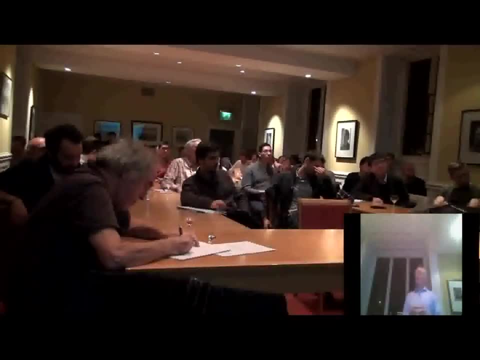 that dominates the theory And it also ignores empirical facts, And I had to mention this today, given that Fred Lee died tragically young, very recently. Fred's work was to point out that the assumption they make of rising marginal cost is empirically false. 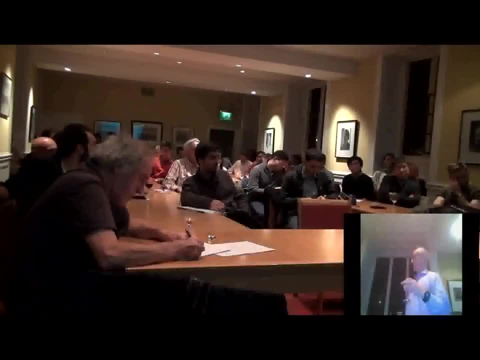 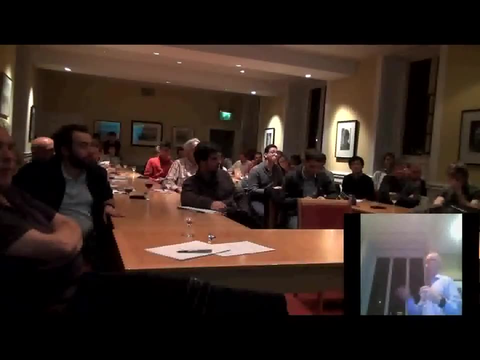 We have about 150 studies, including most recently Alan Blinder's extremely neglected book Asking About Prices, And every one of those studies has concluded that the minimum 89%, which was the level that Blinder found, but normally 95%, which is the level that Eichner and Guthrie- 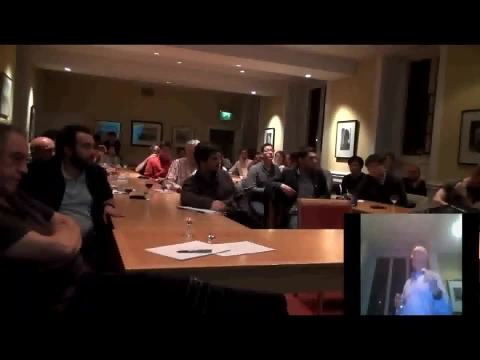 and Deans and so on tended to find in their surveys, have constant or declining marginal cost. What do you see in textbooks? Rising marginal cost. Why don't you see the empirical reality? Because it doesn't suit the theory. This is not a mathematical science. 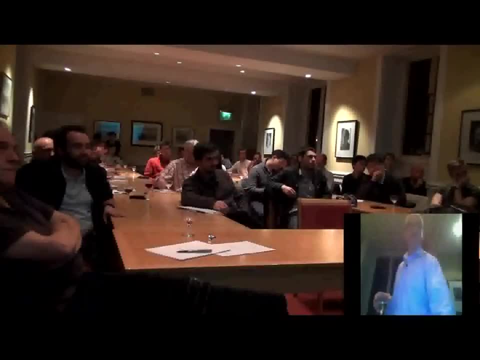 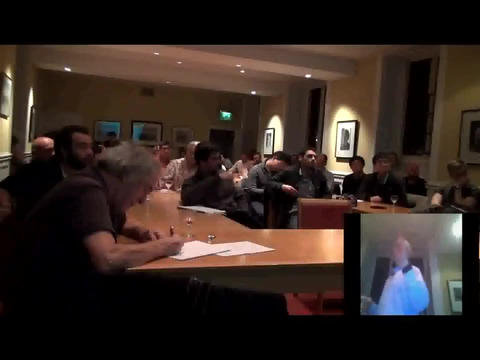 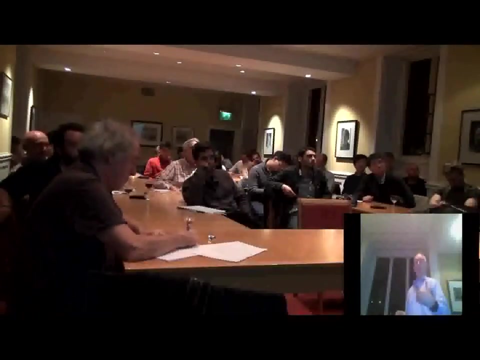 It's mythonatics, not mathematics, So I want to go on now to talking about using it as a tool of logic, rather than just criticising the neoclassicals. How did it help build a new economics? Well, there's a lot of disputes in the post-Keynesian and heterodox fields. 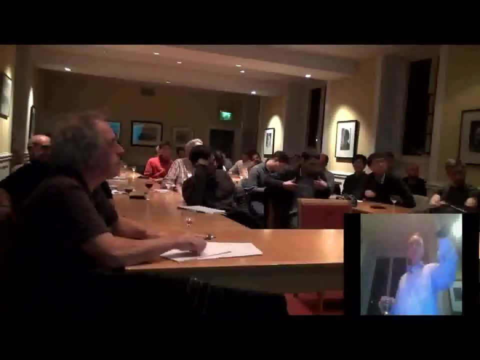 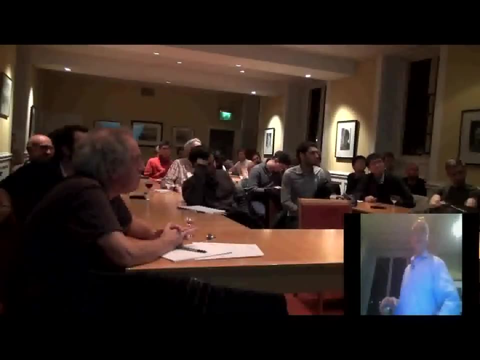 in general, which can't be resolved in words alone, And this is an area where people have much more respect for ontology as I do. Realism is an essential part of how one has to think about modelling the economy, But then you get caught in various theological conundrums. 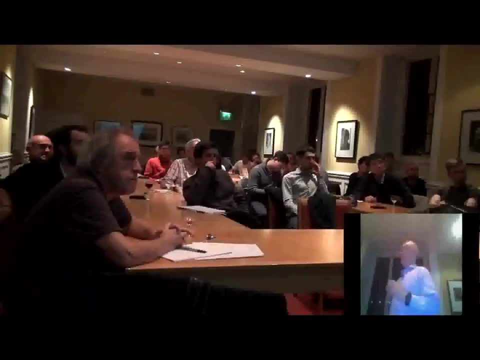 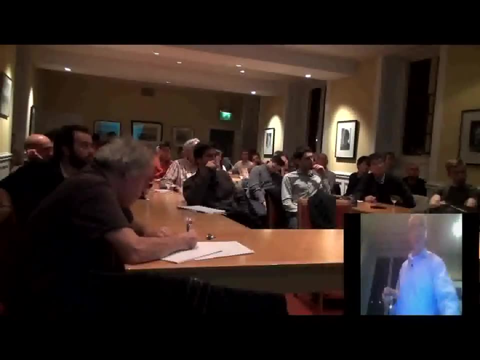 For example- and this is the one that I've been most heavily involved in recently- does a change in private debt play any role in aggregate demand? Now, people have associated with particular stories, which I'm going to modify in the course of today's presentation. 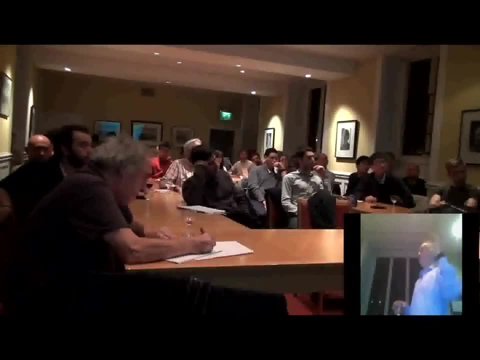 But I'll start with the empirical data, because I have always argued that change in debt does play a role in aggregate demand. And look at the empirical relationship. You'd think there's got to be something going on here. So that's change in private debt versus unemployment. 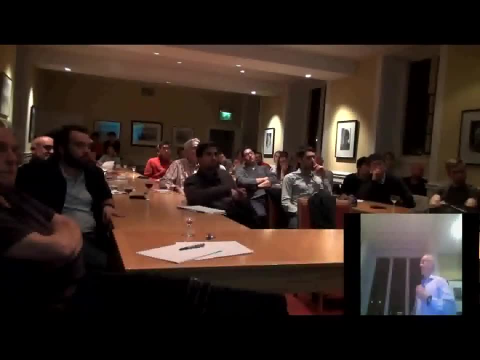 And the correlation coefficient over there over the last 25 years is minus 0.9.. Now I think most of you would know that if you do any correlation at work at all, you'd be rather pleased to get a figure that big. 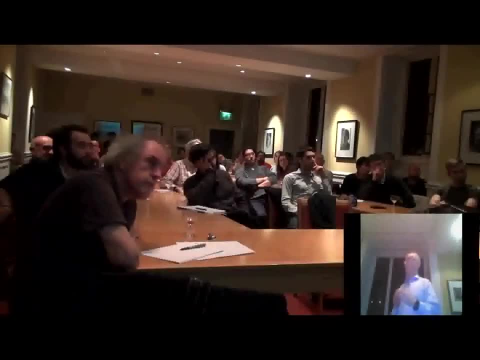 For anything trivial, Let alone something about the relationship of change in private debt to the level of unemployment, when you're told that it should have no correlation whatsoever if you follow neoclassical logic- And Bernanke made that case in his essays on the Great Depression. 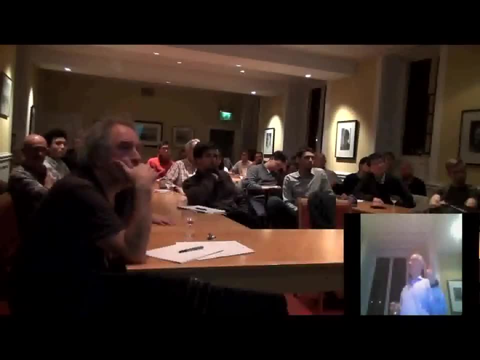 Now, of course, correlation isn't causation, But how do you explain this regularity? This is something which, for genuine scientists, simply having shown this, would be like a black-body radiation problem in physics. How the hell do we explain the sake of this curve? 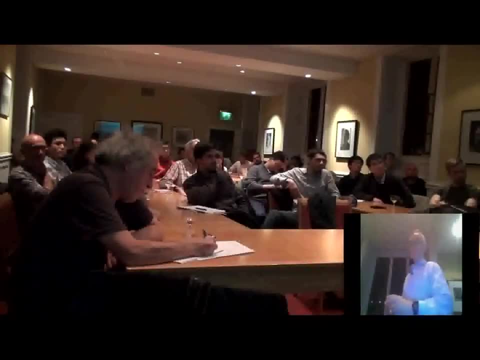 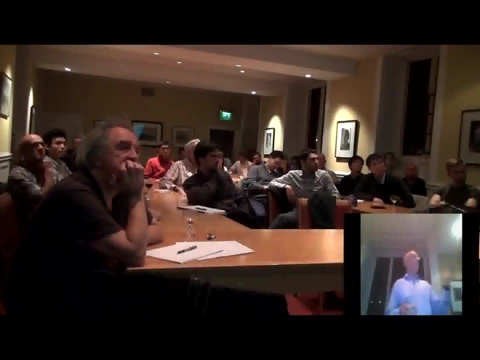 Well, my original shorthand was to say that aggregate demand is income plus change in debt, And I got castigated by not just neoclassicals now, but also a lot of post-Keynesians, Because this implies expenditure exceeds income, Which is a dilemma I was aware of. 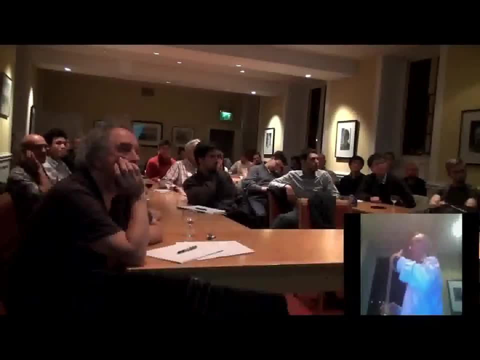 And I made various attempts at making some sort of temporal argument, So saying that change in debt comes first and then the change in income, Et cetera, et cetera. But they went nowhere in terms of persuading staunch critics. 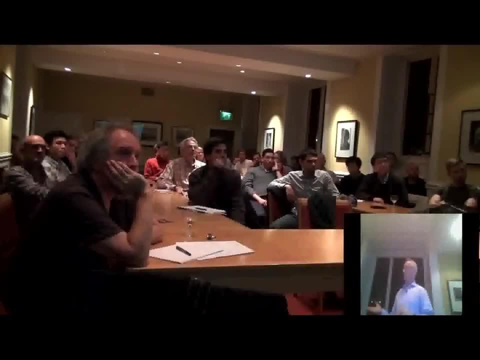 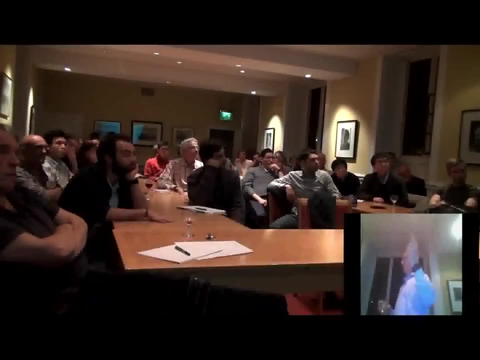 Persuaded some people but not others. And, for example, there's now the review of Keynesian economics. the last edition, the last volume, had a debate where I put my case forward And it was challenged by Mark Lavoie and Brett Feiberger. 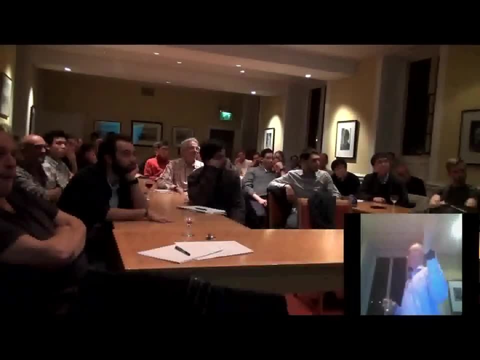 But agreed with by Tom Pally, but with some qualifications. Now, Mark just wrote that sentence at one point. I will not deal with the correlations. I'm sorry if we're truly scientific, Mark, This is good mate. I like Mark a lot. 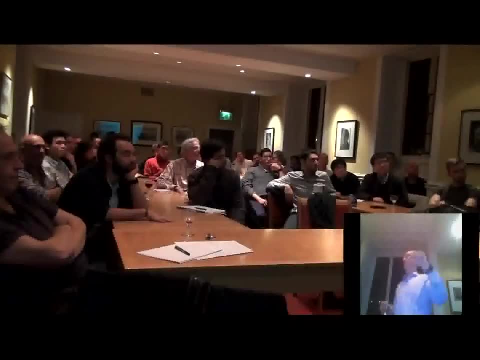 One of these days is going to beat you with tennis mate. You have to investigate stuff that's this. outstanding Correlations like that can't just be rejected on correlations in causation or you know aberrant data, et cetera, et cetera. 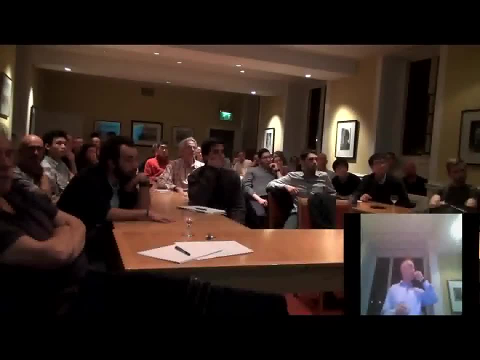 Brett Feiberger made a rather more reasonable statement, and this is actually what provoked me into getting a solution. He said: unless I can explain how the purchase of wood does not provide income for the seller, then I've got to rethink my claim that extensions can force an inequality. 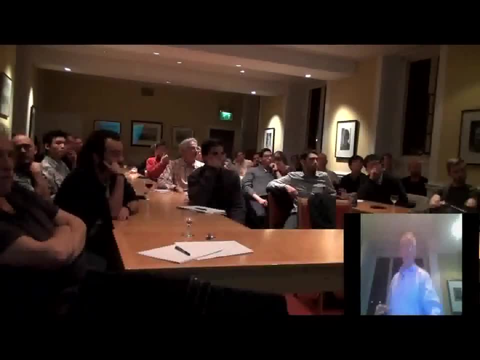 Okay, So he's saying expenditure equals income. How can I reconcile that with the argument that a change in debt plays a role in good demand? Well, my response mathematically was: well, can I you know? this is a good challenge. 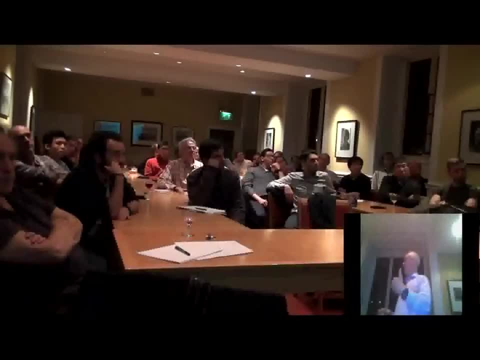 Can I derive the arguments I've got from the argument that expenditure equals income? So I thought I'd put it to an expenditure table- And maths are essential here- because I had to express this. I could have done it logically. You could probably call it more logic than mathematics. 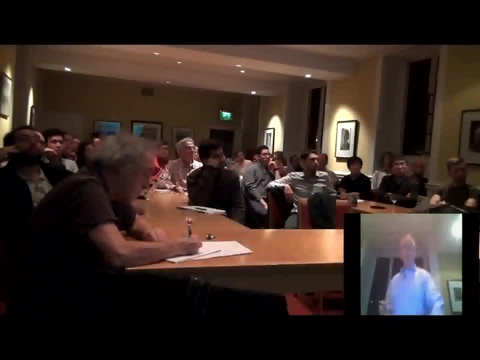 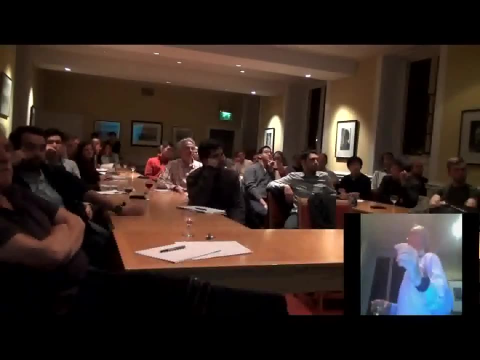 but it's putting it in a mathematical, logical form. So I say expenditure is identical to income in an expenditure table, and then I include debt in both the way the neoclassicals think about it, which is, loanable funds, and the way post-Keynesians do. 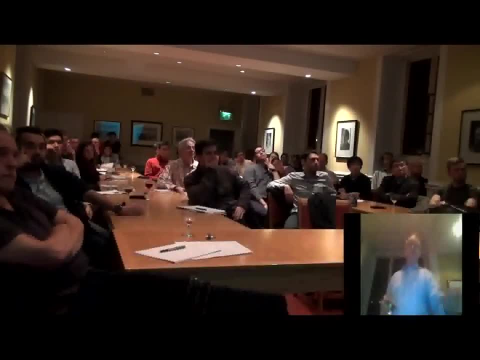 which is endogenous money, and see what happens. So consider a three-sector model. You've got S1, S2, S3. And I show expenditure which is not debt finances: E, X, Y, where X is expenditure by sector X on the output of sector Y. 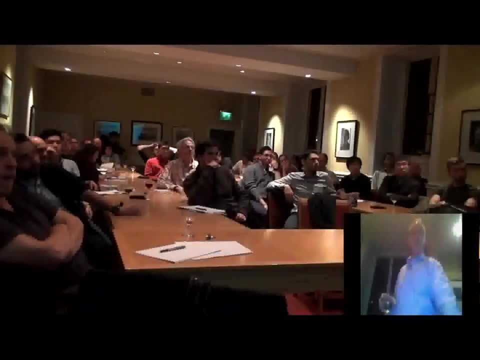 So I can make up a table to show those relations between three sectors And I'm going to consider where there's no borrowing possible at all. You might call that Say's law, but it's actually the inverse of Say's law, Or borrowing from other sectors is possible, which is loanable funds. 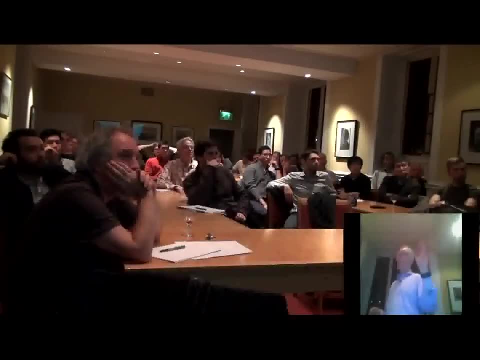 Or borrowing from the bank, which is endogenous money. And let's take a look: This is demand creates its own supply, by the way, rather than supply creates its own demand. So here we have a table, and I've got the three sectors. 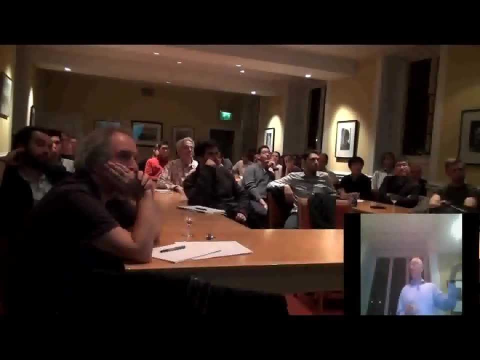 Net income is the sum of the columns, Expenditure is the horizontal. So expenditure of sector 1 on sector 1, we don't look at that. We look at sector 1 on sectors 2 and sector 3.. So the minuses here are the expenditure and the positives are the income. 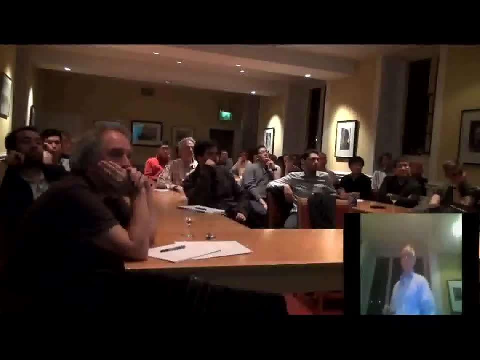 So the negative sum of the diagonals is therefore aggregate demand And the sum of the off-diagonal elements is the net income. This is aggregate income. OK, And they're necessarily going to be equal. Now, when you do the adding up, this is what you find. 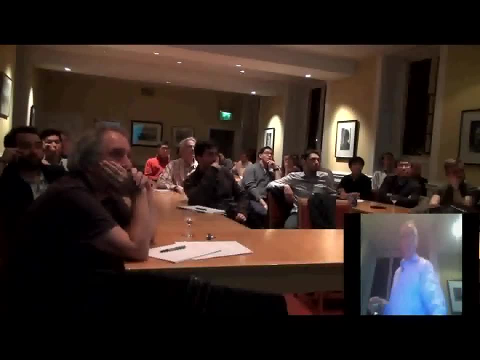 It's aggregate demand under the Say's law situation, Aggregate income under the Say's law situation. One equals the other. Now I'm going to look at loanable funds, where sector 1 borrows from sector 2.. So they're going to borrow delta D from sector 2.. 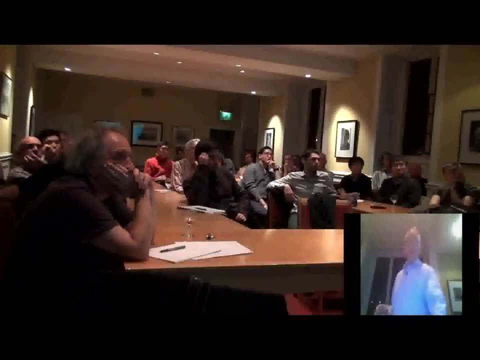 Sector 1 borrows delta D from sector 2. And that increases the potential spending by sector 1. But of course it reduces sector 2's potential spending by exactly the same amount. And I then have sector 1 spending more on sector 2 and sector 3 using alpha and 1 minus. 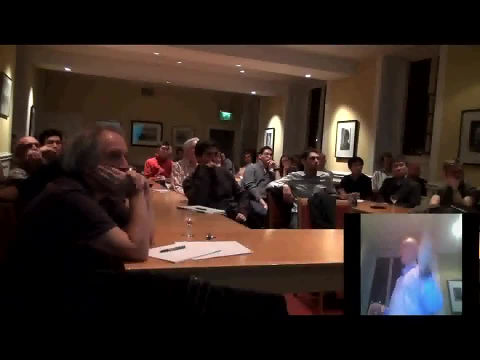 alpha of that, delta D And sector 2's spending, falling by beta and 1 minus beta on sector 1 and sector 3.. So this is now the pattern, including a change in debt where it's financed under the loanable funds idea of one non-bank agent lending to another non-bank agent. 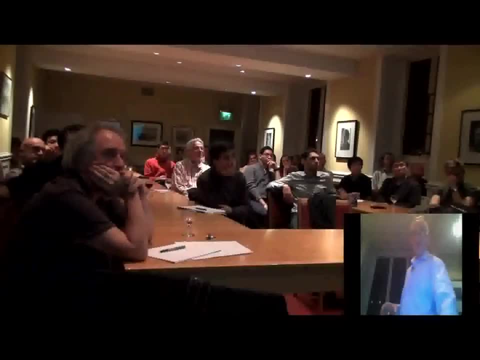 And when you then do the mathematics on that, yes, if you don't do cancellations, you get this nice yucky looking thing here where delta debt is turning up as part of the argument. But when you then do the cancellations, what do you get? 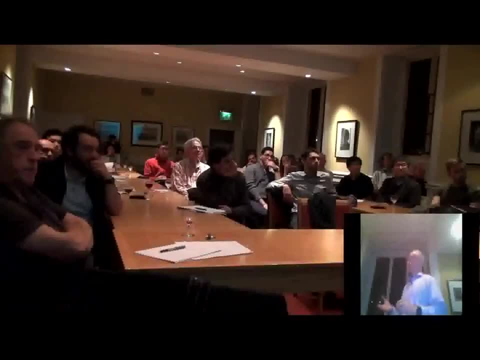 The terms in delta D, cancel. So you're back to the same situation. If loanable funds were true, the neoclassicals are quite right, quite logically justified, in saying change in debt plays no substantial role. There'd be a change in terms of how behaviour might shift between the two agents, but that's. 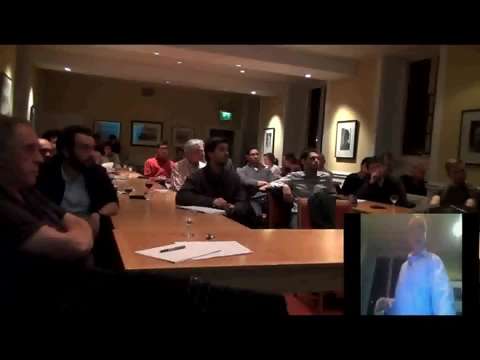 about it. So they're correct. logically, They're wrong institutionally. Now, indulgence money- The borrower's funds- are coming from a bank, So the bank increases its assets by delta D, There's an identical increase in its liabilities, which is now money in the hands of sector 1, and that delta D is then spent on the outputs. 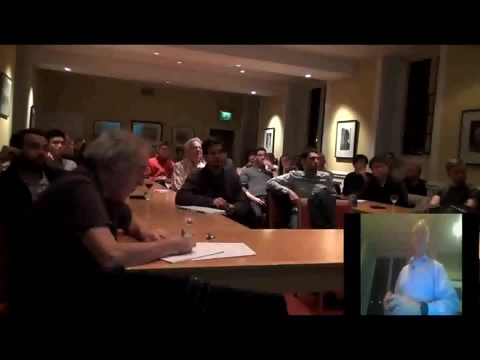 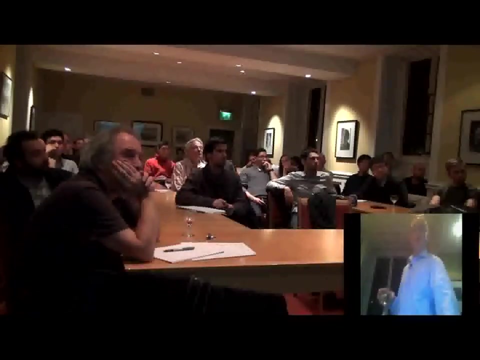 of sectors 2 and 3.. So here's your equation there, or your table. It only lifts by no minus delta D on the second row to the loanable funds. And when you work it out, there's the full expression and the terms in delta D, no longer. 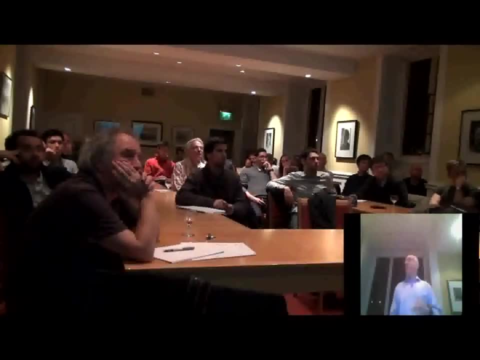 cancel. When you get the reduced form, you find aggregate demand is change in debt plus expenditure financed out of existing money And so is aggregate income. So both aggregate expenditure and aggregate income and non-debt financed expenditure, which is the turnover of existing stock of money plus the change in debt. 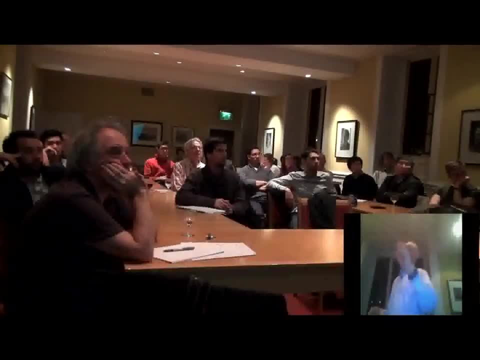 It turns up in both of them. Now, that was not a surprise to me. It was nice to get that resolution. It also generalised to a flow of new debt. So if you have, rather than just a one-off, change and you're looking at a flow of new, 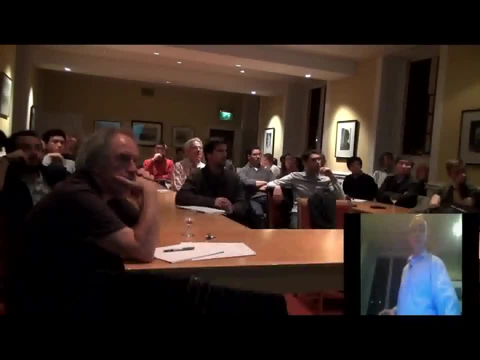 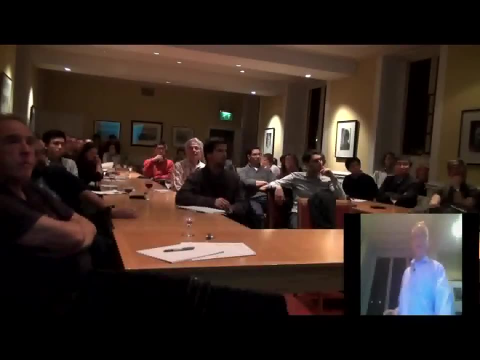 debt, a flow of new lending coming in from the banking sector. then you can expand the expenditure financed out of existing money by velocity, And I'm bringing velocity back into this. So that's the argument about net-care economics again, plus the change in debt, plus also. 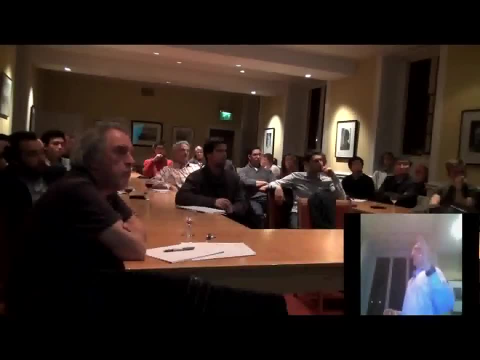 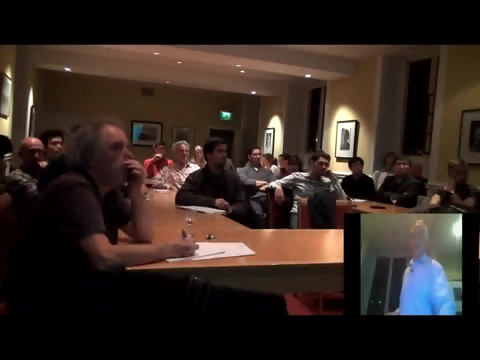 net gross financial transactions. We're talking aggregate income, That's income of the lenders and the borrowers. So both those terms- that was surprising. I didn't expect that, I must admit. The same sign for revenue for depositors and the revenue on loans. 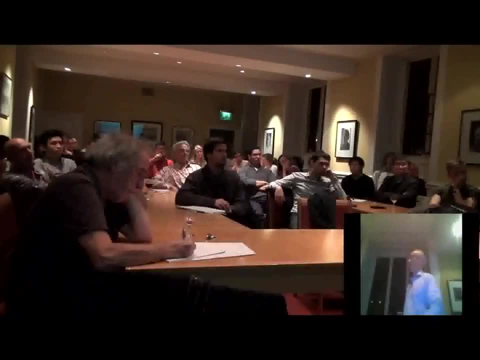 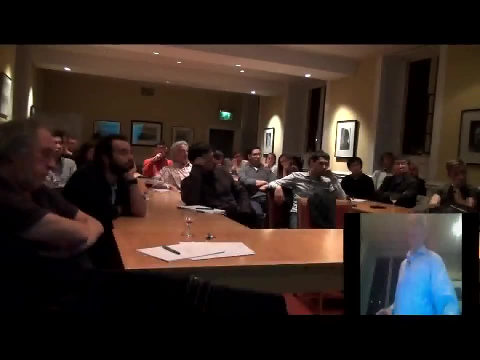 And we now look at the change in aggregate demand, I've got an acceleration term coming up. So the argument for a long time that acceleration of debt is a major factor in the change in demand, And now I've got the mathematics behind it. 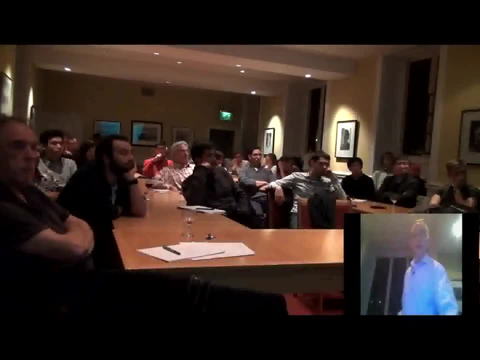 So I've got a different conclusion to what I expected. Certainly the most strongest one for me, which I was surprised, was these two having the same sign That I didn't expect. It took me a while to understand it. I had to accept it because it's a mathematical conclusion. 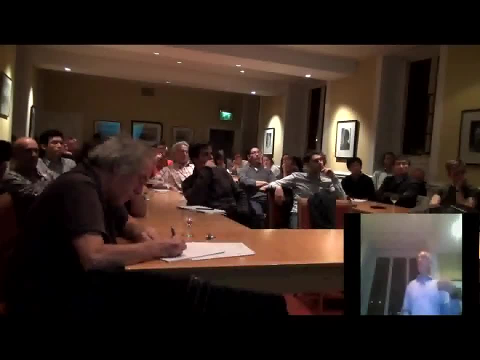 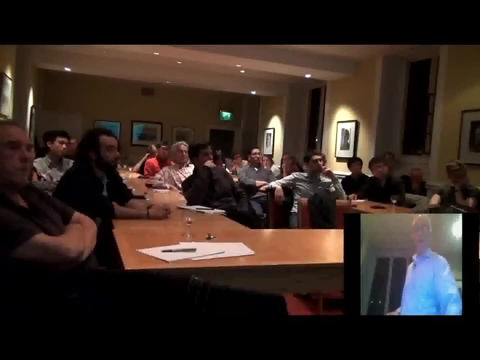 And it provides a causal explanation for that correlation, And particularly- And this depends upon the circumstances- The larger the level of debt, the larger those terms are going to be. So it really applies more to post-1970s data than beforehand. 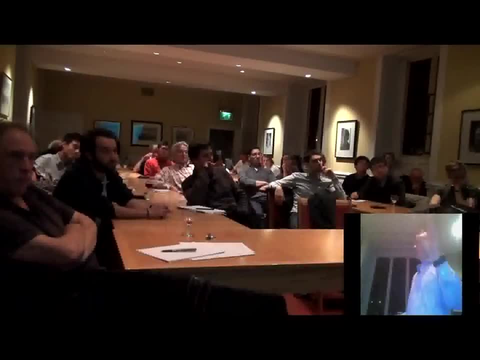 But it also ends up with a different conclusion about rejecting the role of change in debt in aggregate demand, And I hope it does transform how post-Hansions think about the role of debt in demand and in aggregate income. So that explains these ridiculous correlations. 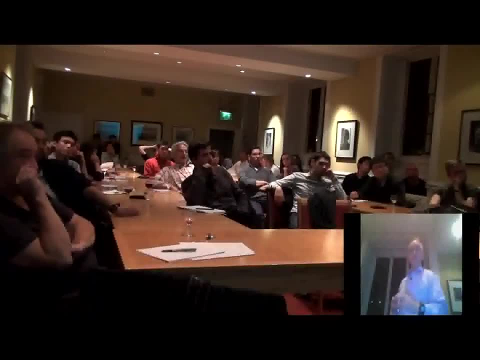 This is taking a look at the correlation of the acceleration in private banks. This is taking a look at the acceleration in private debt and change in unemployment in America over the last 25 years, That's minus 0.89.. Again, not to be ignored. 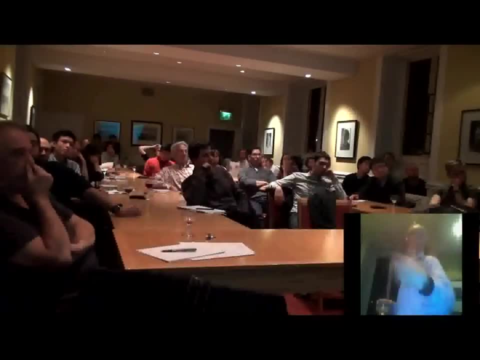 But it's still ignored by neoclassicals on a priori grounds. And what are the a priori grounds for ignoring it? Well, it's the loanable funds issue. This is where I had a good old fight with Paul Krugman. 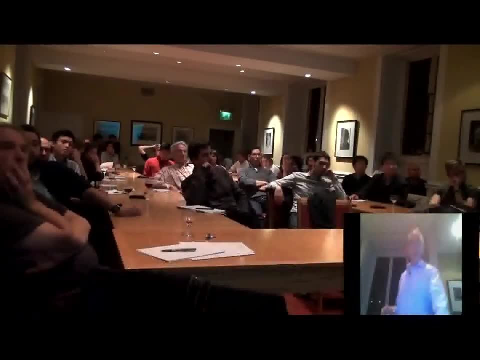 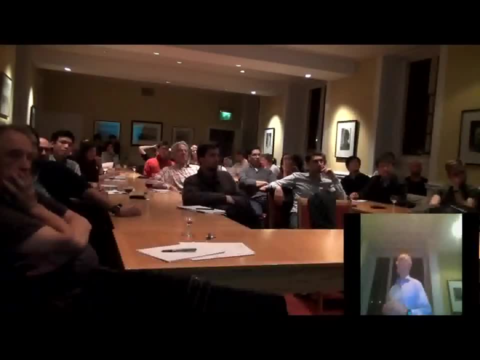 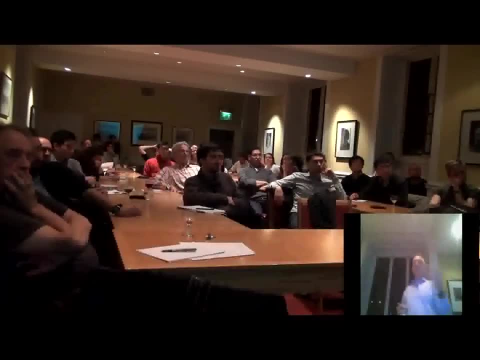 This is the thing which people who don't study economics actually don't realise. They're shocked when I tell them They think economists are experts on money And say: no, they're experts in finding reasons not to consider money Good, So they'll get employed. 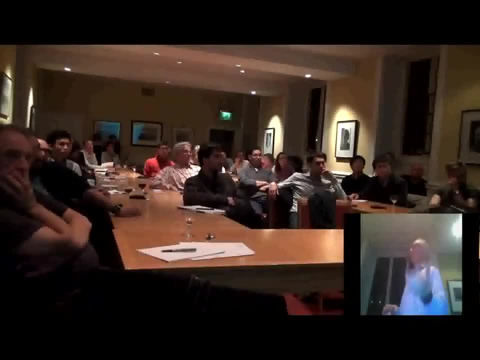 So they're. else, If they're still in government, why wouldn't they be good enough to include some of this information into their savings economy? Right, And they are experts. It's just a one off, All right. But here's Krugman saying self-proclaimed Minskyites- which obviously is me and many. 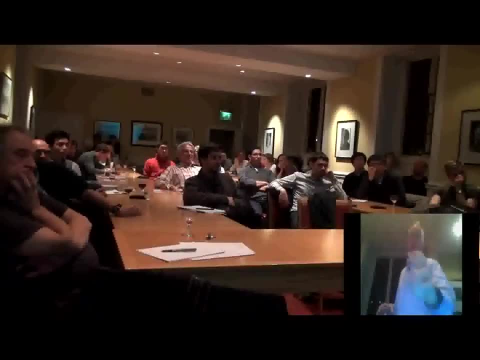 others of you banks that are somehow outside the rules of the rest, he says. I don't see it that way. Banks don't create demand out of thin air any more than anyone does by choosing to spend more. In other words, he's making an equivalence between banks lending money and individuals. 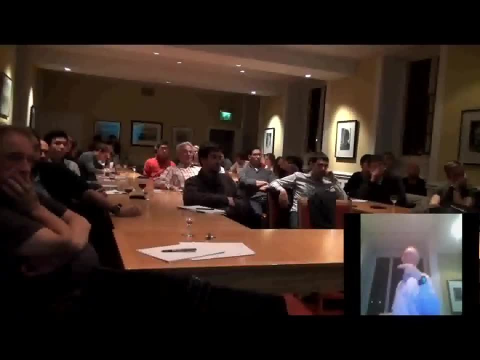 lending money to each other And he says: you'll get the claim that he doesn't understand it as he does and it's the mystics who have it wrong And, in my opinion, he and the neoclassical school in general- the barter mystics. they 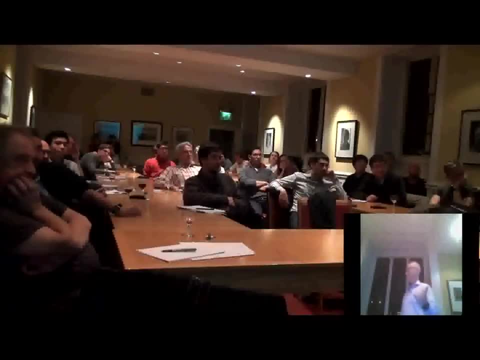 imagine you can model capitalism without banks, debt and money, And to me that's like trying to model birds without wings. Good luck, So again another statement from him, from his in this depression. now he said when: 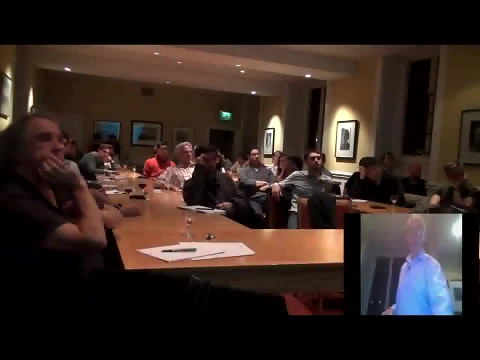 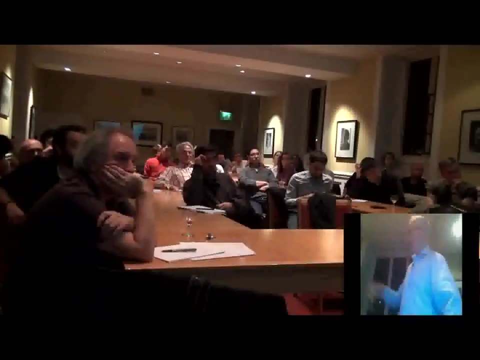 debt's rising. it's not the economy as a whole borrowing more money, which I think is precisely wrong in indulgence money terms. It's a case of less patient people borrowing from more patient people. Now I have I've given up on arguing with these guys, but it's fine to take their arguments and 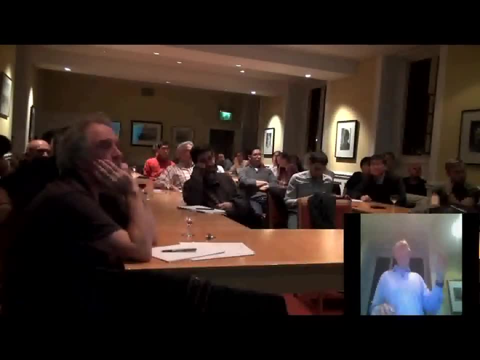 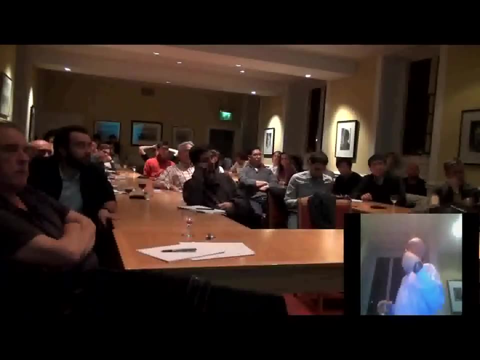 put it in a mathematical form and show who's right by just changing the structure. So what I've done is build a model in my soccer package, Minsky, which is a rendition of the loanable funds model of banking you can find in the appendix to Eggertson and Krugman's. 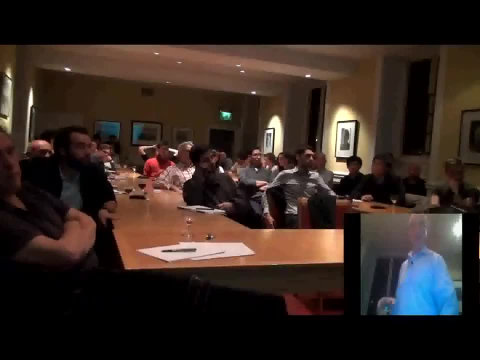 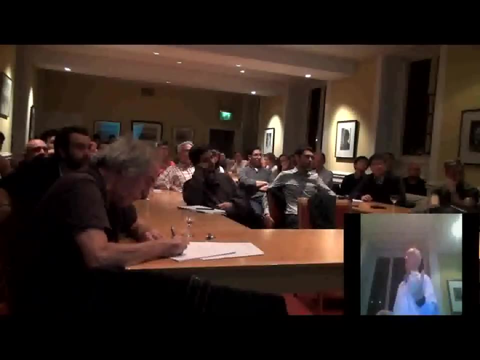 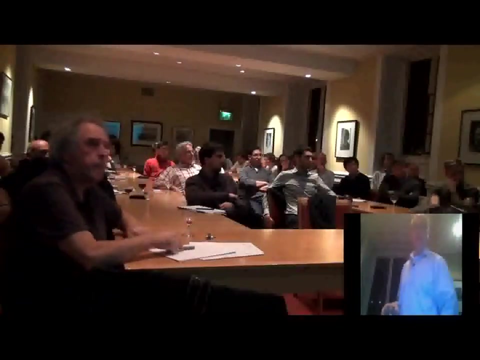 paper in the Quarterly Journal of Economics Got a very stylized banking model at the end of that particular appendix And I can show that they're right. If that's the actual structure of lending, if patient agents lend to inpatient agents, then you can forget about bank's debt and money. they don't matter, except during a liquidity. 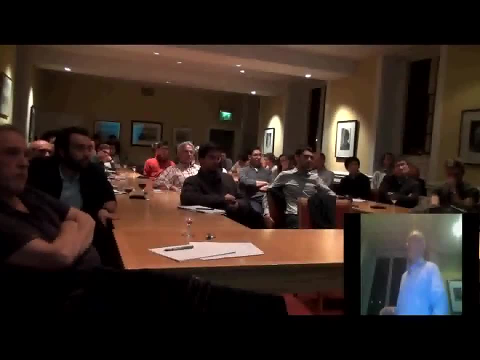 crisis And change of debt do have minor impacts. but just by changing the velocity of circulation Then I can just alter the structure of that model from loanable funds to indulgence money in roughly 30 seconds. You can time me if you like. let's see how long it takes and see what happens when you. 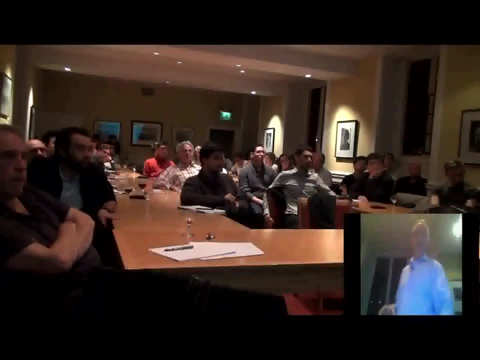 look at the world where the banks are the ones doing lending rather than patient agents and inpatient agents. So in the appendix what he has is a consumer goods producing agent lending to an investor goods producing agent charging interest for the loan, and then the bank has arranged the 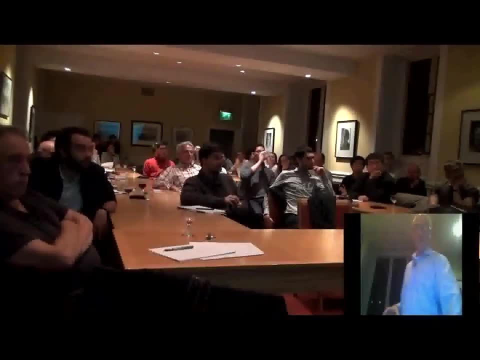 loans, so the bank gets an intermediation fee. That's the basic structure of the banking model in that particular paper. So I've set that up in Minsky and it looks like this is a balance sheet. I've got a bit more detail in the actual model, which I'll show you in a moment, but there's 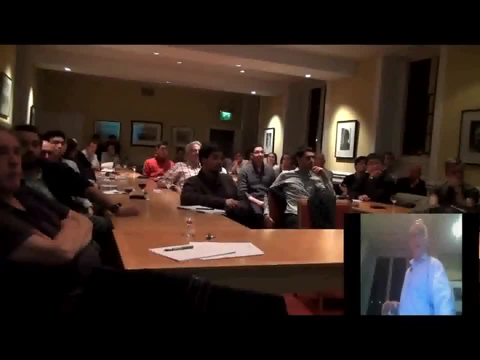 lending from the consumer agent to the investment agent and that's the flow of lending from positive to minus. The convention there is- I'm using Uminski and it's also very similar to the convention used in accounting- is that assets are shown as a positive and liabilities 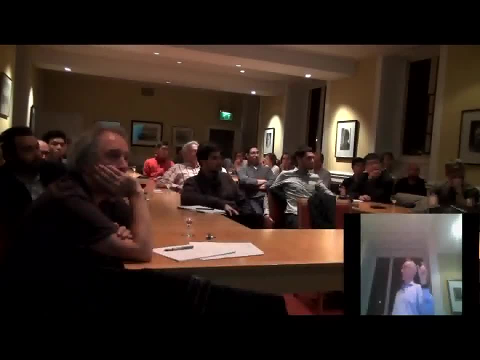 and equities are negative, So the flow and the flows always go from plus to minus, and that can be changed across to debit and credit for those that are in accounting. exactly the same concept. So that's the flow of lending. there, Notice, debt doesn't turn up because 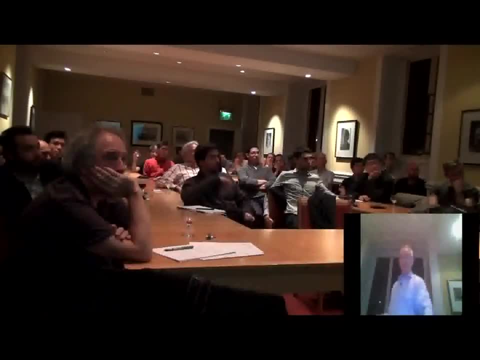 I've got. this is the bank's point of view, and the bank doesn't actually own the debt in this model. so debt has to turn up in another table, and that's the one for the consumer sector and also the investment sector, because the debt is an asset of the consumer sector. 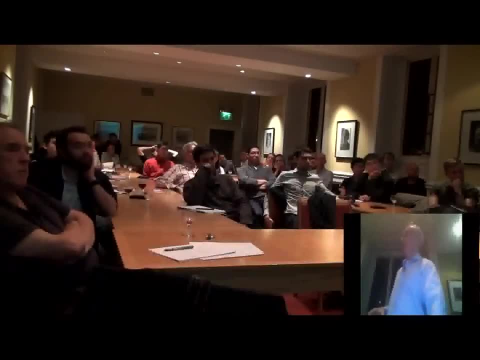 and a liability of the investing sector. So there's the debt turning up as a positive asset, as you can see, of the consumer sector And lending reduces the flow of lending and that's the flow of lending. Lending reduces the consumer sector's cash but increases the asset they've got in terms. 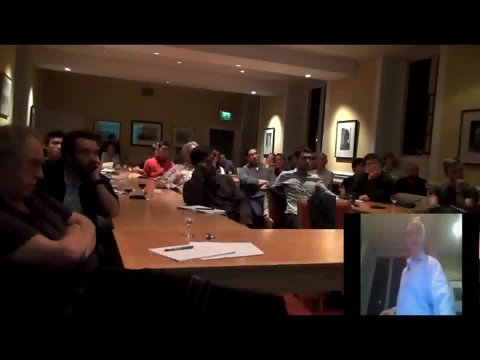 of a loan. So there's lending reducing the amount of money they've got in their bank account, but it increases the amount of asset they've got which are earning money by having been lent to the investment sector, and it's got to do with that cash for the duration. 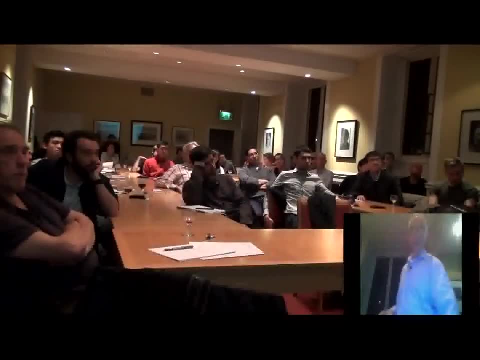 of the loan. Now, when you simulate the model and I'll bring it up now, oh dear, I didn't. I thought I'd set that up to be- it automatically started. I think I've just mistaken my presentation. Let's see if I can find the file itself. Pardon. 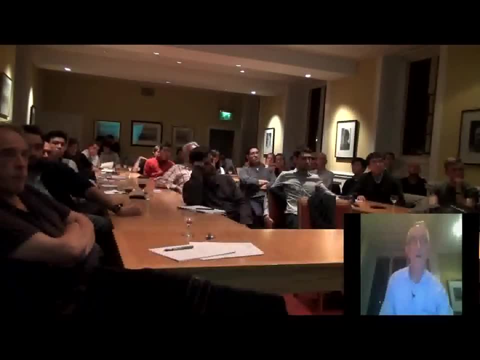 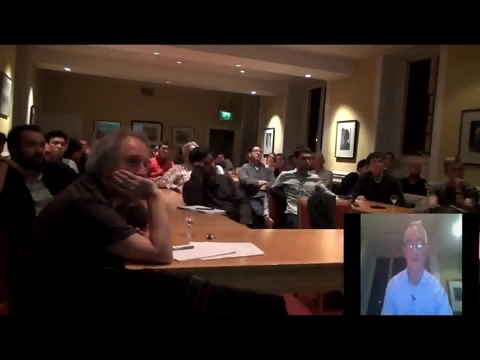 me. So this is the Minsky model. Minsky is a piece of is a beta software. We're still revising it. There's a particular bug in this version where the we can resize the size of these tables that show banks, but unfortunately it's not stored when you save it, so it's 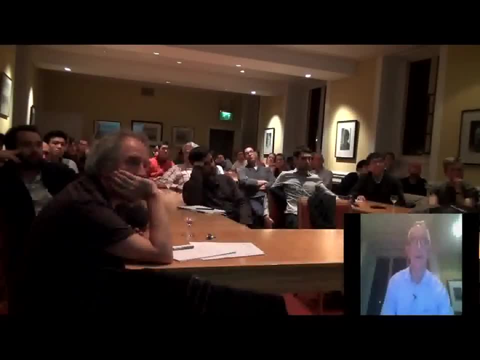 got to save, reduce the size here So you can actually see what I'm doing. Let's go back to zero again, And this is where I'd like to have a larger screen, but you've got to live with what you've got. So if I simulate, 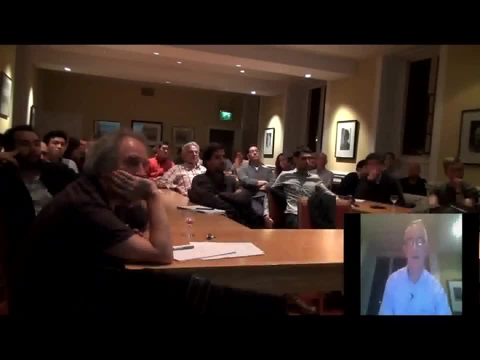 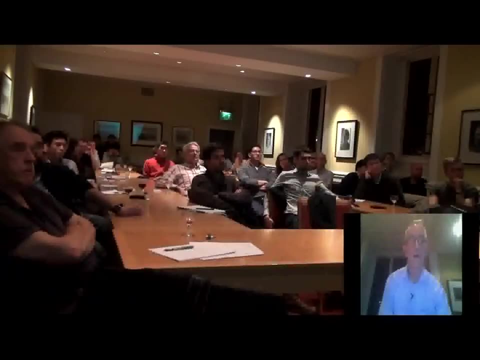 this model I'll just bring up. let's see what's a good graph to show here. Bring up a large graph of GDP and then simulate the model and change the rate of return and you've got a little bit of an increase in the net income and the net profit. So we're 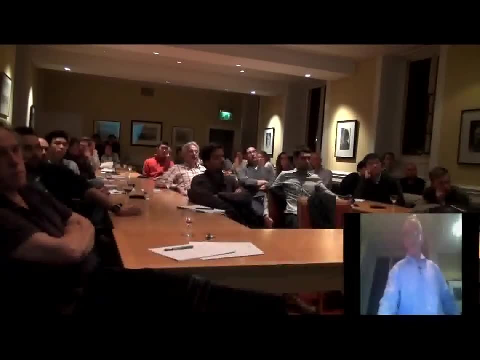 going to go to the number here and we're going to hit a few, we're going to hit a two, So we've got a value of zero and then a value of five. So that's how we're going to see where it's going to be. 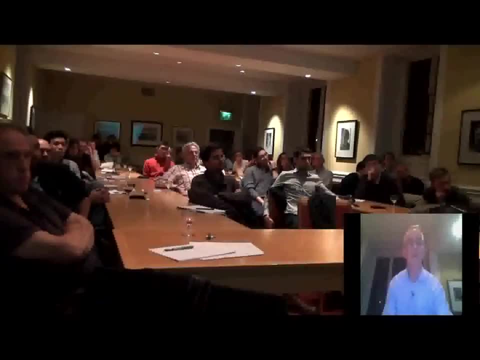 If I say double the amount of borrow, it'll go down to zero. So we can see now that I'm going to lower that value. but if I go back below- and let's just put it down here and see where it went back- it's going to go down there. If I do that, I'm going to get a zero. 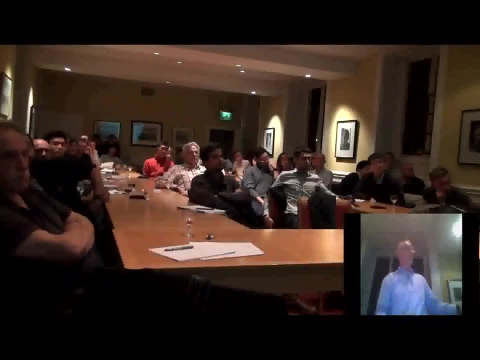 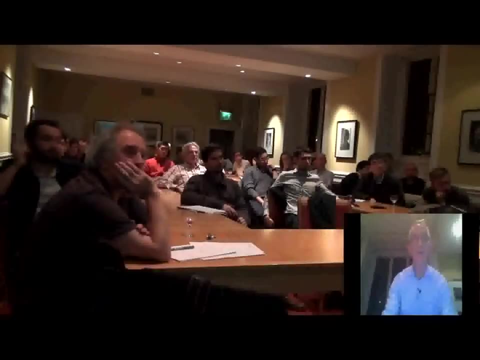 So you can see a dramatic change in the stock of debt compared to the amount of money. Keep on simulating and go back to the original situation: total collapse of lending, very slow lending. then back to the original situation and then increase in repayment rates and then. 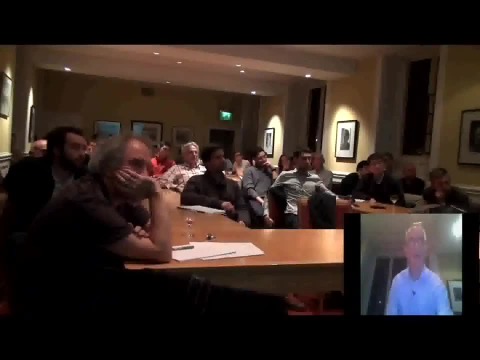 decrease back to the original situation. Lots and lots of changes in the ratio of debt to money. looking at what's happening in GDP, almost nothing. The simulation has now been running for 1260 years and we're still looking at a GDP rate. 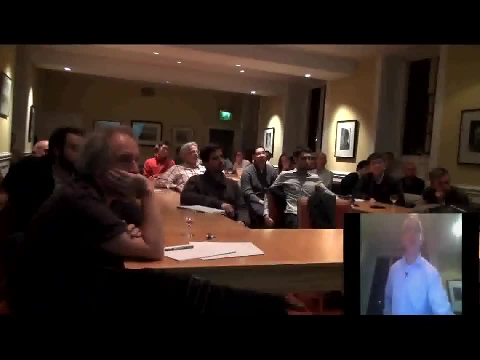 of roughly 200.. So it made huge changes to the rate of lending and had bugger all impact on the macroeconomy. So if they were correct, it would mean you can ignore bank's debt and money in modelling capitalism. But here's going to be a really mystical thought. 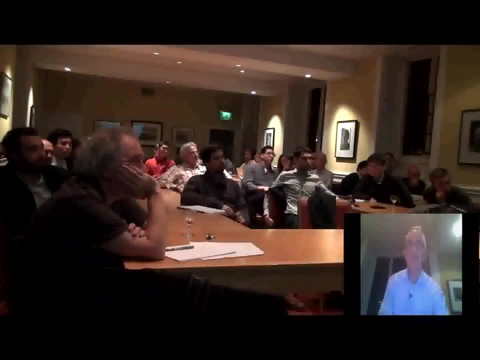 What if it's banks that do the lending rather than the consumer sector? Well, bring up the consumer sector table here and notice I've got debt there as an asset of the consumer sector. Well, it's not. It's an asset of the bank. 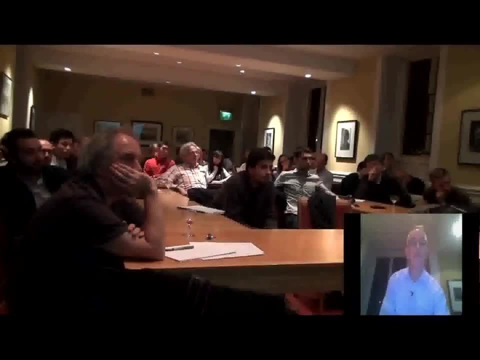 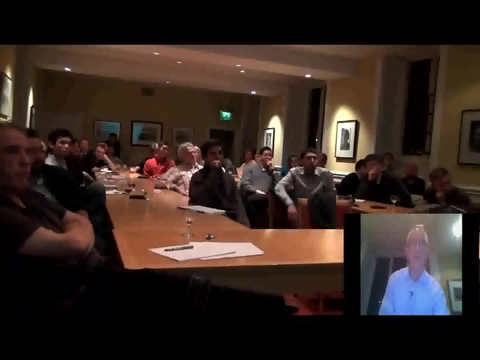 So I'm going to delete that column and I'm going to delete all the financial operations that in fact go to the bank instead and come back. I've got a couple of things I should fix up a bit more accurately, but that will do as. 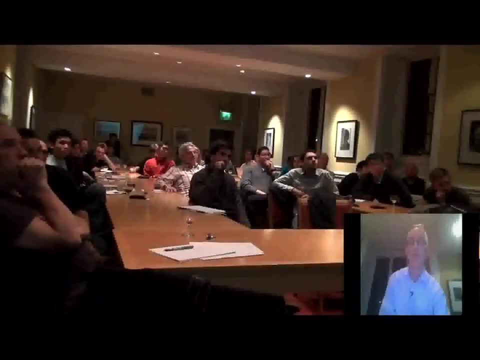 a start And then come over here and add additional asset into the banking sector's table. The program remembers the debt is still there, so it brings the operations across the table. So I'm going to delete that column and I'm going to delete all the financial operations. 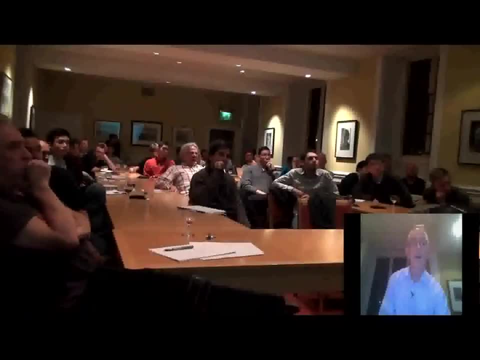 that in fact go to the bank instead. That's quite a bit of mess for me And all I have to do now is say: well, all the payments here go to the banking sector rather than going to the consumer sector, And I'll delete this now superfluous bank fee. 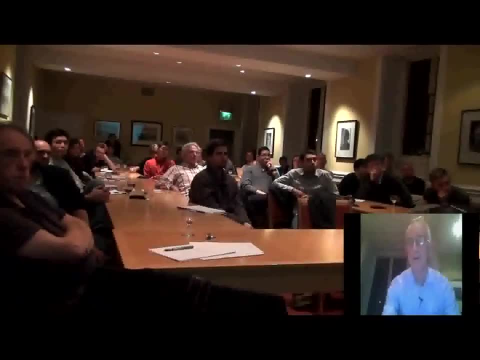 And if I had the option I could delete, see, rather than the amount, then you'd be depending on how much is in the consumer sector's account. it's actually related to the level of debt. just to change that, Stop the whole system. 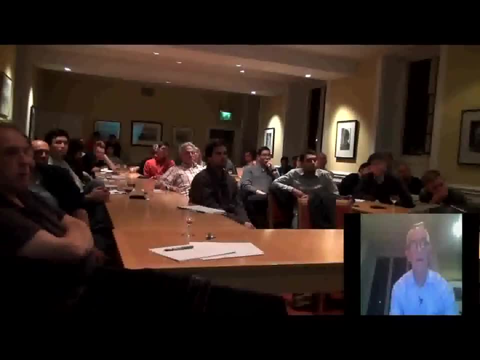 and simulate again. let's just move down a bit. I shouldn't do these things live. you know it can go. it's working. notice the red lines rising. the amount of money in the economy is growing because of the lending. if I now have an increase in the 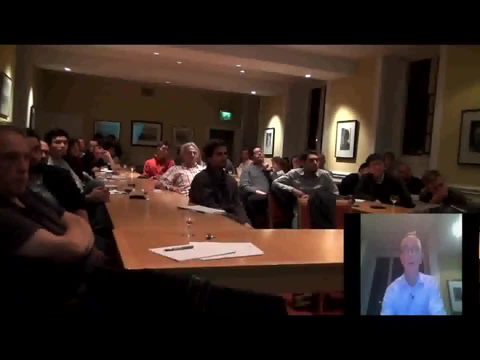 rate of lending and a decrease in the rate of repayment and notice the red lines rising a bit faster again. if I didn't have repayment happening much more rapidly and lending much more slowly, then down we go with the amount of money in the economy. I now restore the original situation and let's check. 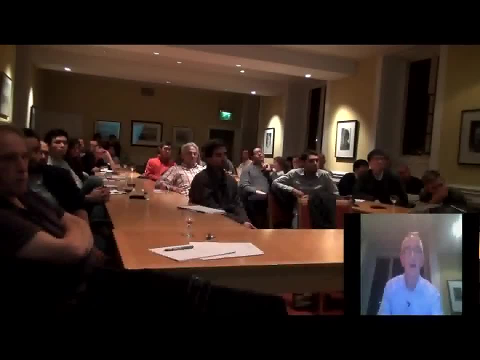 and see what's happened to that GDP figure. we've had a boom and a slump, so a typical simple piece of realism, and I hope I've trashed loanable funds. I don't need to do it for this room, obviously you, but that's how simple it is to illustrate the difference between the. 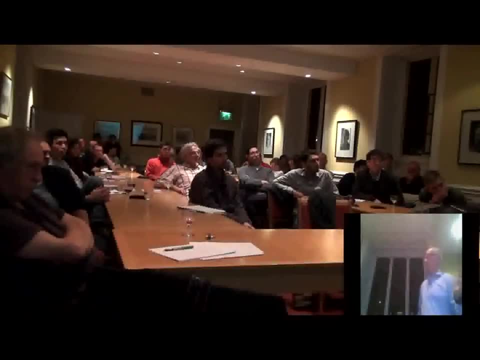 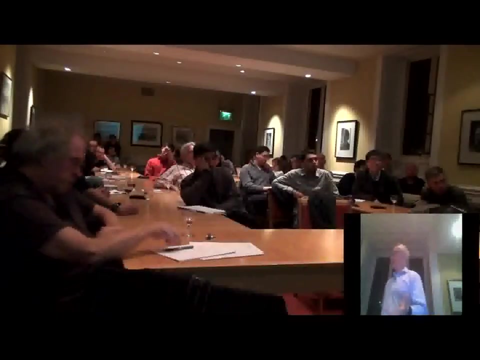 two. when you have a mathematical tool that connects, you, do it. otherwise you run around in circles talking the poor program and I'd rather do other things that I'm running around in circles. so that's the outcome. change in debt matters. the banking sector matters. money matters, debt matters. it's, it should be a. 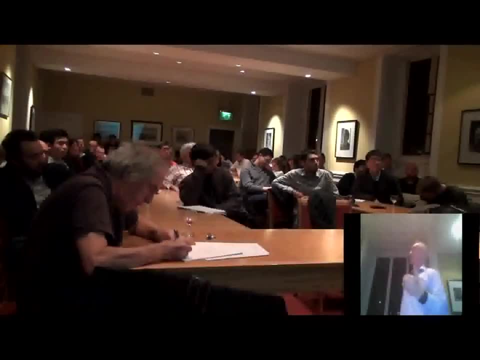 no-brainer to solve that. of course the heart, the no-brainer part, is getting them to actually look at a simulation like this and saying, oh dear, we didn't realize that. but of course they won't do it. so the banking mystic ŠIZστ as 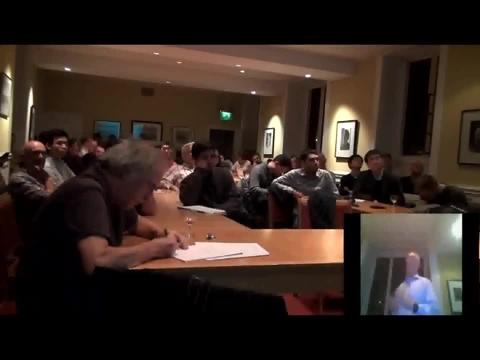 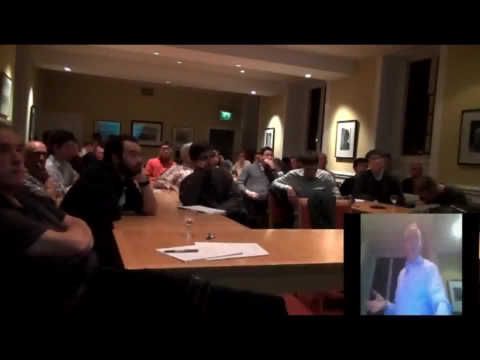 Cuban calls him arrived. a changing debt has a dramatic effect on the macroeconomy and what's actually going on mathematically is that learning all funds is what's called a conservative. not, that is right wing, which is concern something. it doesn't change the amount of money. if you stupid, where the money. 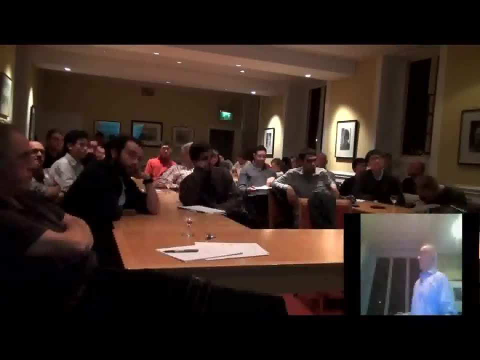 is that it doesn't change the amount of buying an existence versus還 use money as well as quality. significant money exists, just it doesn't mean to something dissipated. it means it's not. i think, if i just ref custom kit now and then just allowing them to manufacture a system, that doesn't mean that something being dissipated, it means that nothing's gonna disappear, for that's called a dissip etmek. sistemون broament emdokнос money fitness boolah gem. 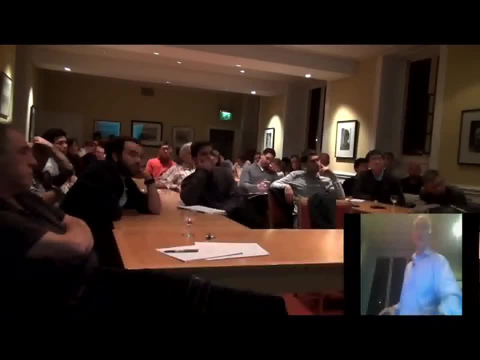 is nothing remaining constant. there's no given quantity that isn't altered by the dynamics. so money creation- money is created by increase in debt and destroyed by debt repayment, and we can spend our rest of our lives running around circles arguing this verbally, or we can show it in the 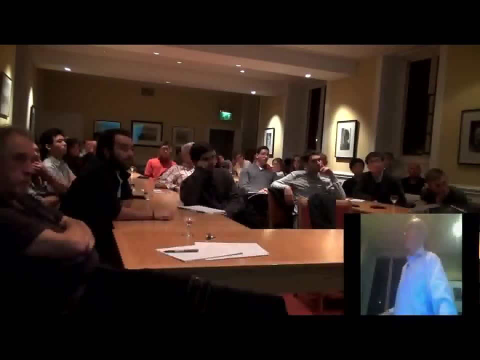 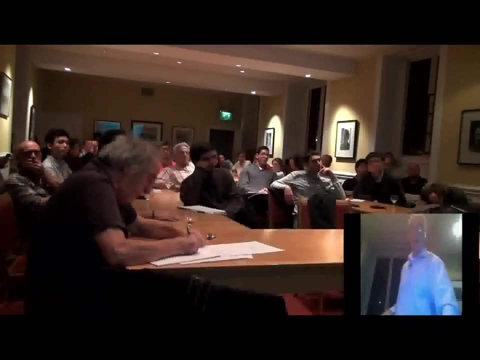 mathematical model, and i think mathematical model wins. as a way of you know, i don't argue for those who believe otherwise. so if they behave like mathematicians, then we'd get rid of this particular dispute. but of course they don't. they'll continue ignoring it. but what if mathematics? 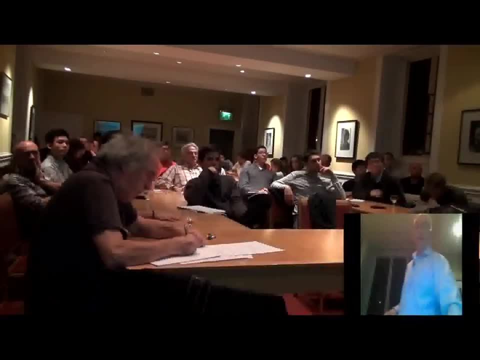 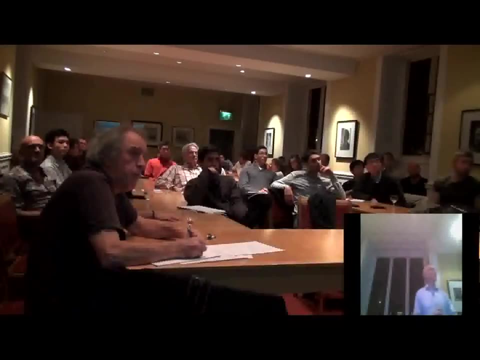 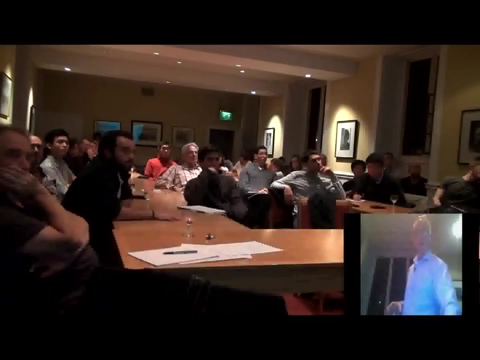 actually was a mathematical discipline. what would it look like? well, i think i could say that it would be complex systems analysis, which could be described as a modeling of social realities, an emergent phenomenon of human interaction, not only optimistic, highly transient, reproduced and transformed through practice, the process of cumulative causation. 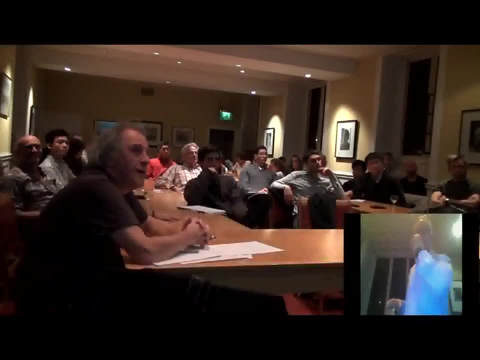 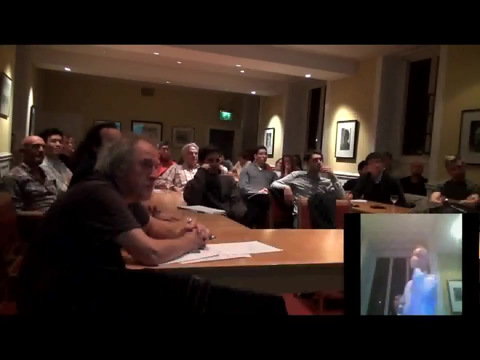 aware that social reality is causal and processual, prior to prioritizing the goal of being realistic, fashioning methods in the light of that ontological understanding and recognizing limits of a taxonomic science, in other words, consistent with lawson 2013.. and there are mathematical tools for open systems. they do exist. they've been commonplace in sciences. 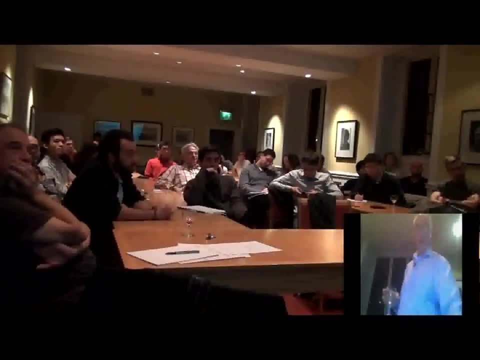 for the last 40 or 50 years, rather than the reductionist and atomistic nonsense that neoclassicals are still hanging on to. and the start was back in 1899.. ponkar a did the proof that there was no solution: the three body problem. that was the beginnings of our technical awareness of chaos and complexity. 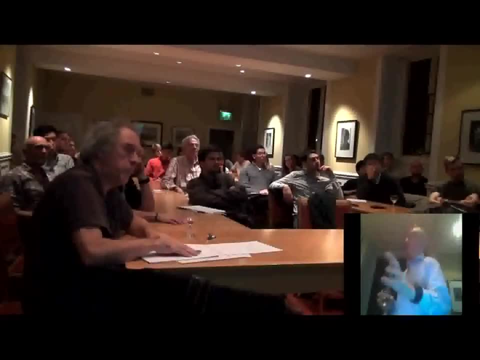 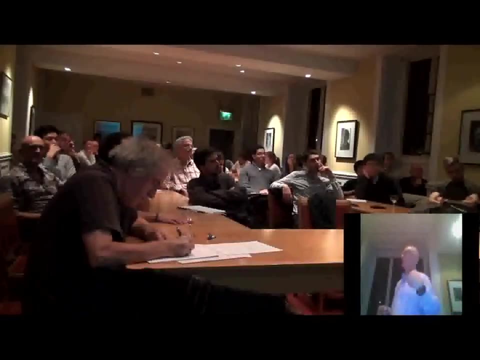 that began with lorenz's demonstration of deterministic non-periodic flow and his focus, as a weather modeler, was saying that we're invalid to use linear models and pattern matching. they can't do that. it just doesn't work because most of the energy comes out of non-linear interactions. 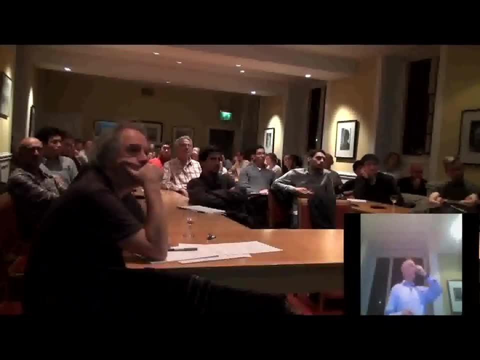 and he says, in dissipative systems- which is why i made a comment earlier about dissipated versus conservative- governed by finances of linear equations- constant forcing leads to constant response, you see? but that's not. it's a non-periodic flow. if you have a linear perspective, it looks. 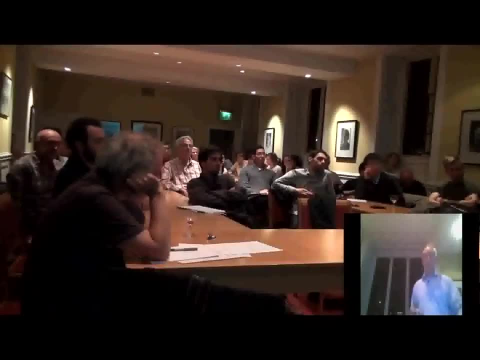 like something. it must be a result of something coming in from the outside. but he said that is not applicable at all when you've got a non-linear system, and it is was the classic example of chaotic and complex systems. so you have a simple model that has just three variables in continuous time. 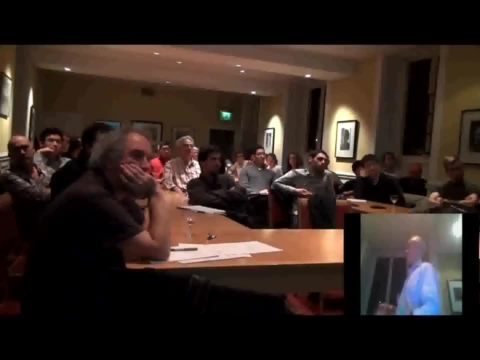 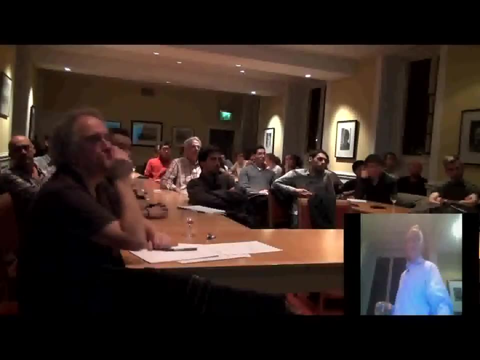 and three parameters, three scalar parameters. it generates three equilibria, all of which, for realistic values, are unstable, and you can't model that as a system. this is a sequence of equilibrium states, because it's never in equilibrium. so this is, in fact, lorenz's model. 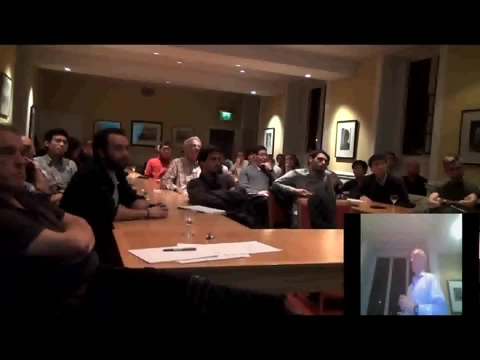 in equilibrium, which i think is an extremely exciting thing. the xy plot from the top shows the xy variables plotted against each other. the two bottom ones show the variable over time. exciting, isn't it? this is the same model. let's bring it up, but i hope i've got this one set up properly. 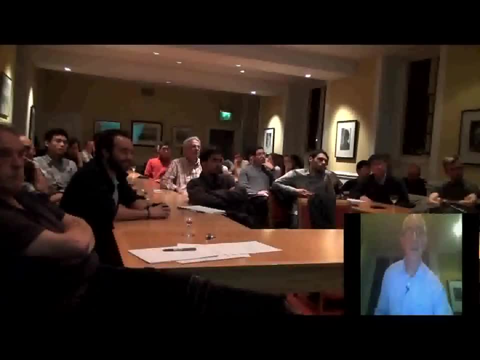 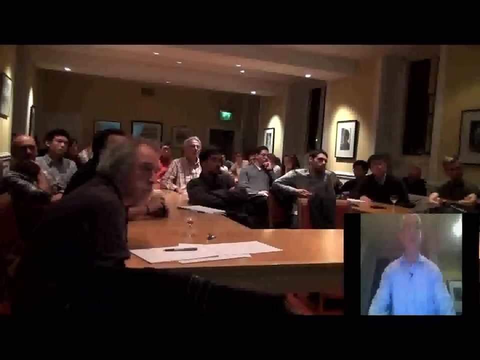 oh, i haven't. bloody hell. okay, can i stuff up some presentation? here's lorenz's model. let's simulate it live. so if i simulate this without a shock, what you see is equilibrium. okay, starting off with this very equilibrium, if we start, and start just tiny fraction away from the equilibrium for the first, 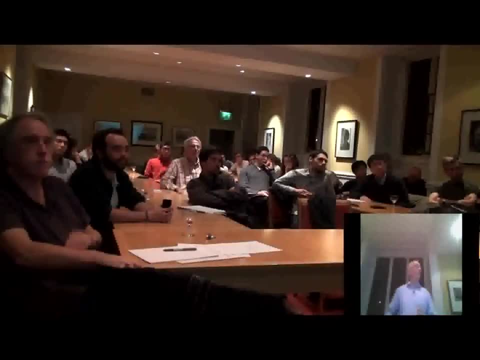 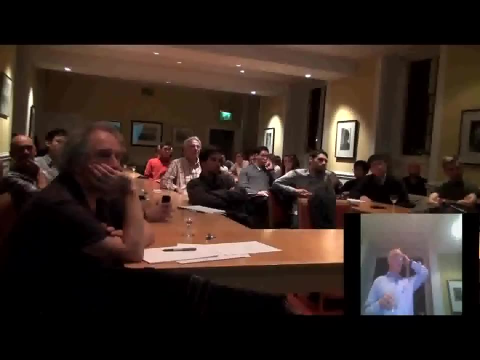 step and then you get rid of the shock and run it on. this is what happens. as i said, there are three equilibrium in the system. there's a zero, zero, zero equilibrium, and two involving the positive and negative square roots of uh, of a quadratic plus uh. one more, one more constant, and you can see that the system started. 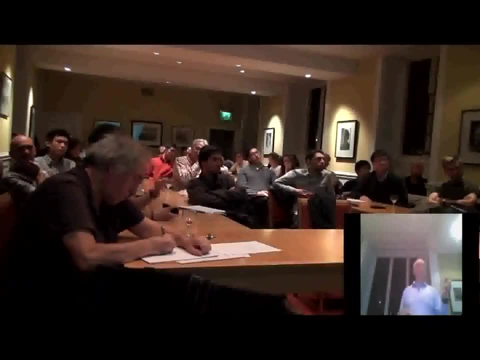 near one equilibrium rather than moving away and returning back to it after a shock, which is the usual neoclassical thinking- it blasts off out of the system. it doesn't blast off to infinity, and then it starts to cycle around the other two equilibria and through the third or past the third. 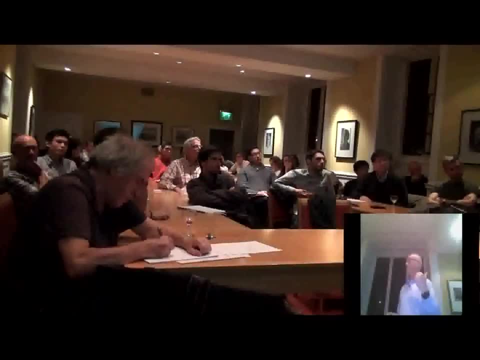 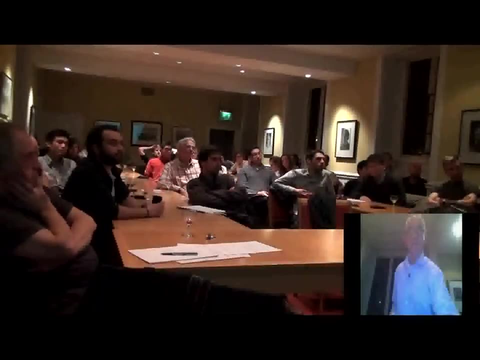 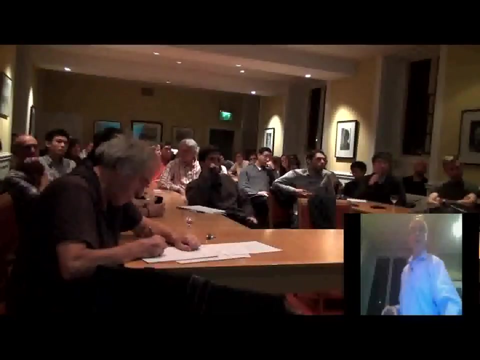 equilibrium. this is the system. you can see. this is the equilibrium of equilibrium, is not the equilibrium of equilibrium. it is the equilibrium of equilibrium. it is the equilibrium of equilibrium. so if we ran this demonstration for a million years, it would still be no end. it would never reach the equilibrium values. the system is inherently non-equilibrium and that's. 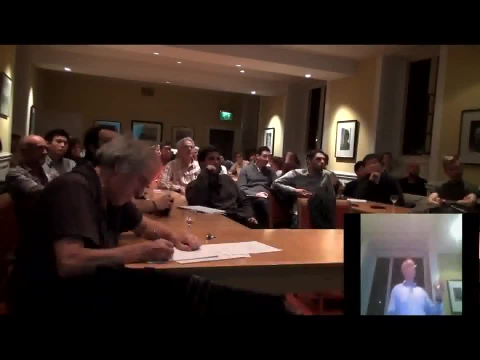 commonplace in the real sciences today. so that's the system: just one, 0.1 for the executive and the other two values in equilibrium, and this is consistent with what you'll find in physics, what I could call applied reductionism. A wonderful paper called Law is Different. 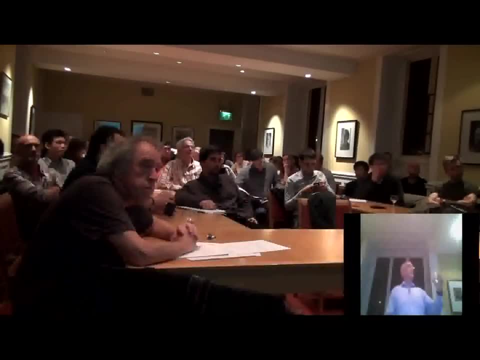 If you haven't read it, it's very much worth a read. And he said the main hypothesis in reductionism is that reductionism doesn't imply constructivism, constructionism. He said the fact that if you can reduce everything to simple fundamental laws, 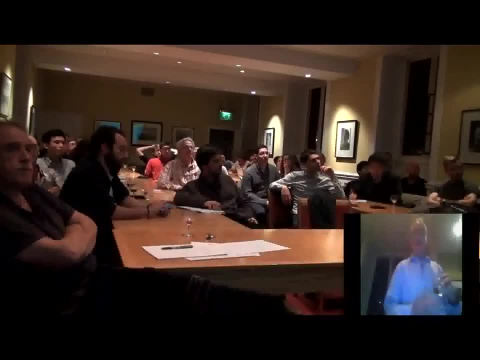 that doesn't mean you can construct the universe from those laws And it breaks down completely when you reach the combinations of both scale and complexity. And of course the economy is a classic instance of both scale and complexity. And he said the behaviour of large and complex aggregates. 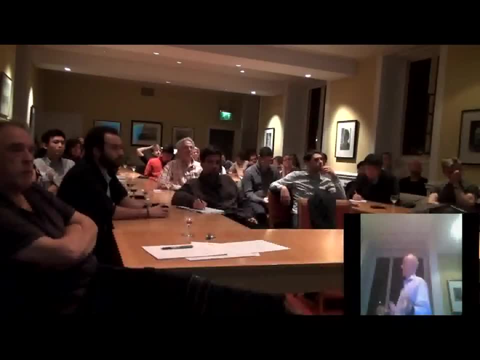 of elementary particles is not to be understood in a simple extrapolation of the properties of a few of those particles. So that really again characterises how neoclassicals think, And what that means is, in a simple way of putting it: 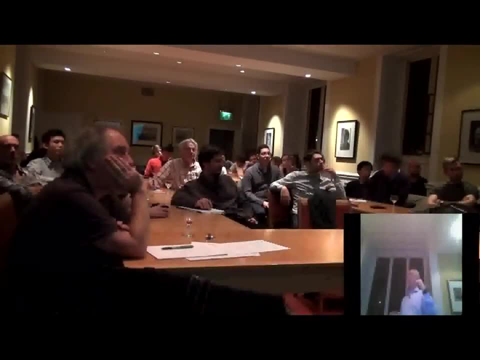 when you do a hierarchy of the sciences. yes, biology, psychology needs biological organisms, but psychology is, It's not applied biology. And yes, you need chemistry to be alive biologically, but biology is not applied chemistry. If it were a typical biology exam question would be: 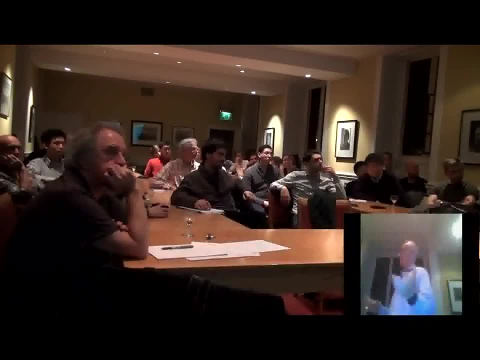 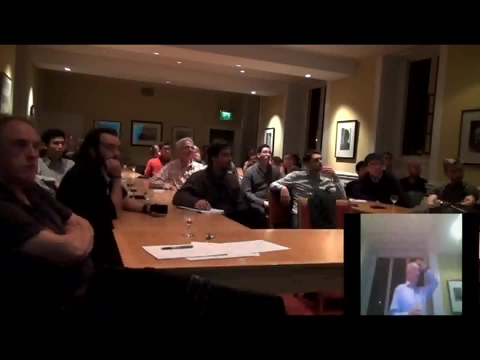 please take these chemicals and create life. Biology is sensible enough to know that's not a very good question, or rather it's too good a question. but economists believe they can construct macro out of micro, So you get entire new levels applying. It's an argument against the reductionism. 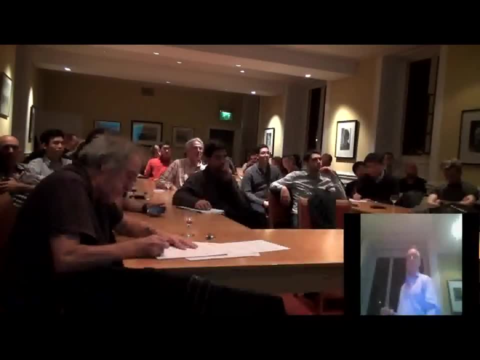 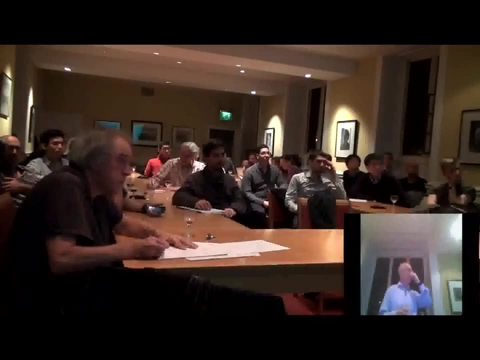 which still dominates neoclassical thought. So the The whole is not only more than, but very different from some of the parts, And one intriguing thing I find about this paper is that it's a curious finale. I reread it before I gave the presentation here. 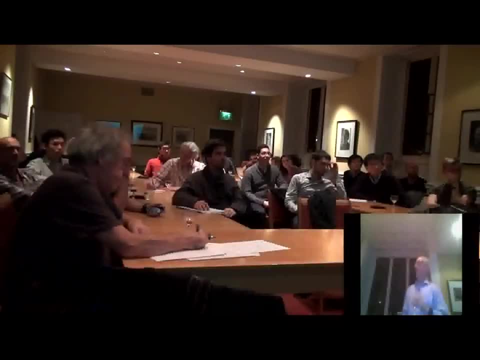 and it hadn't stuck in my mind, but I thought this is wonderful. In the closing, he offers two examples from economics. Who does he choose One? Karl Marx. to begin with, saying that Marx said quantitative differences become qualitative ones. 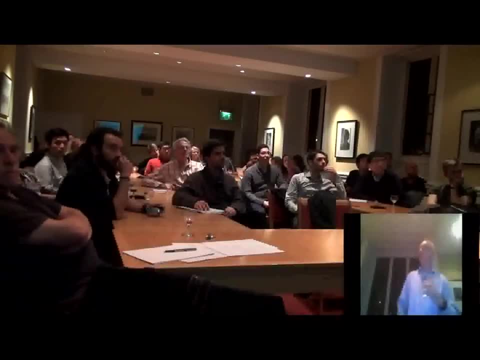 But he said. a dialogue in Paris in the 1920s sums it up Even more clearly. Fitzgerald says the rich are different from us, And Hemingway says yes, they have more money. So maths and economics should start from complex systems. 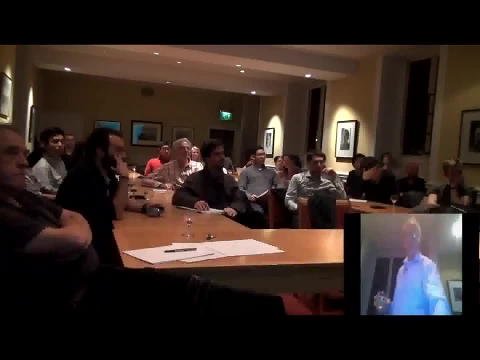 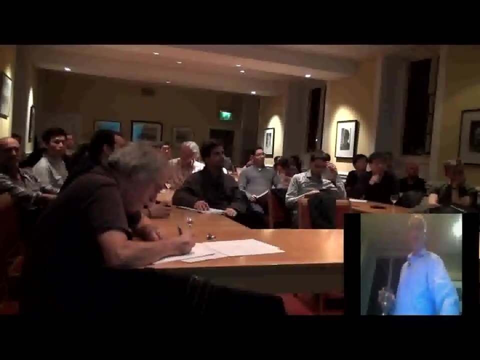 It's not the end of it by any means, and it's not the complete domain either, because there's things you can't do in mathematics. There's more modesty amongst mathematics than amongst any economist. That starts from nonlinear systems, from non-equilibrium. 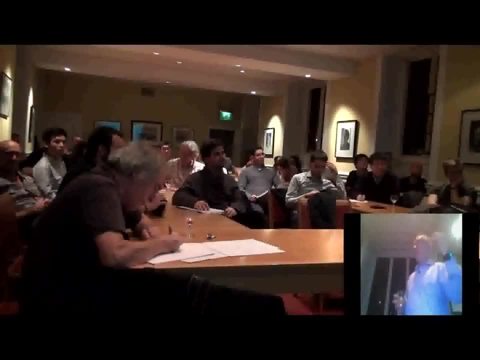 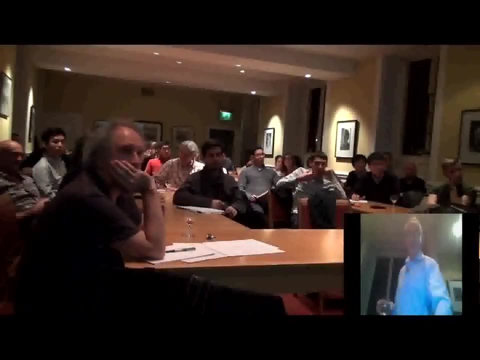 and also monetary systems as well. So. So I'm going to show now another case that's applied this complex systems thinking to Minsky's model of financial instability, which is the main area that I've been researching for the last 20 or so years. 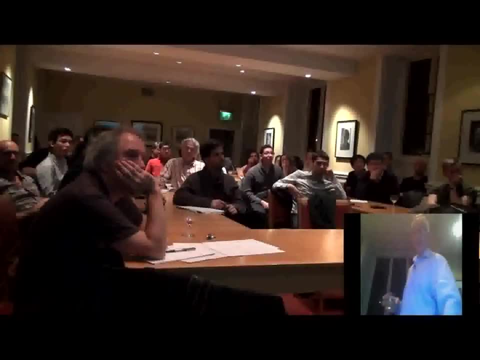 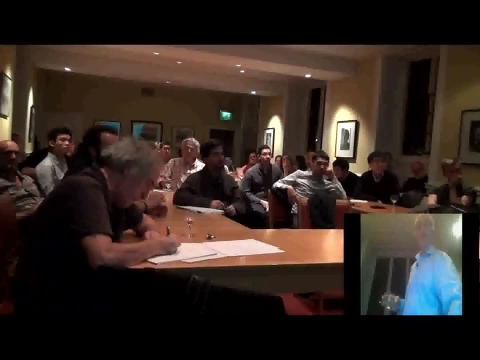 And Minsky did flirt with mathematics in his PhD and a bit of Cholesky later, but he pretty much did the whole thing verbally And I think what I've done is put those verbal differential equations in a mathematical form. So his instability hypothesis starts from this proposition. 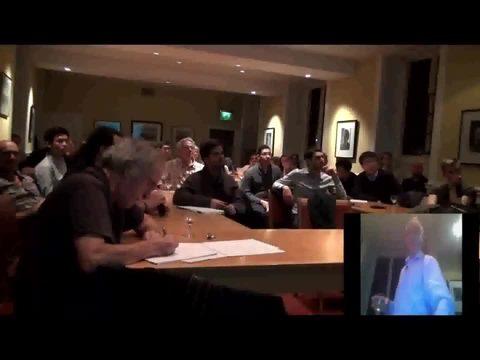 It's necessary to have a theory which makes the Great Depression one of the possible states of our economy, And he had a time and dataware model with an economy in historical time where there'd been a debt-induced recession in the recent past and therefore both firms and the main borrowers in his model. and banks were conservative about the debt-to-equity ratio and therefore only conservative projects got funded. But because the economy has got to the recovery stage, most of those projects succeed. so firms and banks both revised their risk premiums and accept the high level of debt-to-equity. 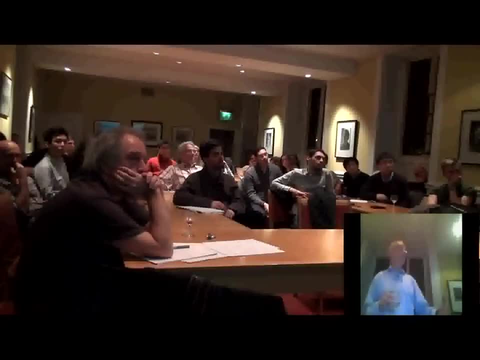 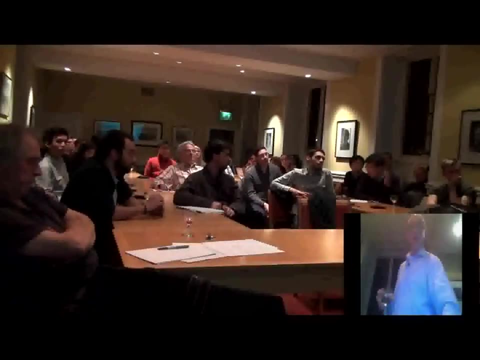 and start valuing assets more highly. And then you get to what he called the euphoric economy, where having a period of tranquil experiences in the economy causes rising expectations, which is that stability or tranquility in a world where the cyclical past and capitalist financial institutions is destabilising. 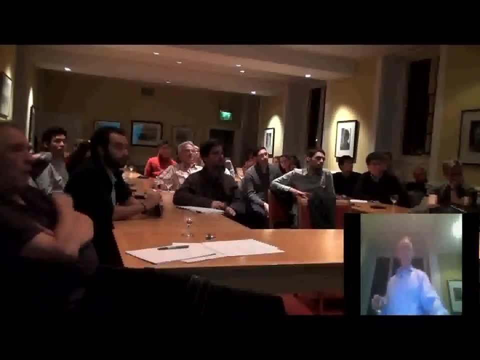 Again, ultimately non-equilibrium thought. So you have self-fulfilling expectations. A decline in risk aversion causes higher investment. That causes the economy to grow faster. You have rising asset prices, making speculational assets profitable. There's an increased willingness for their money. which causes an expansion in the money supply and an expansion in demand, as I've argued earlier. And you get Ponzi financiers turning up whose cash flow is less than their debt servicing costs. They profit by selling assets on a rising market. 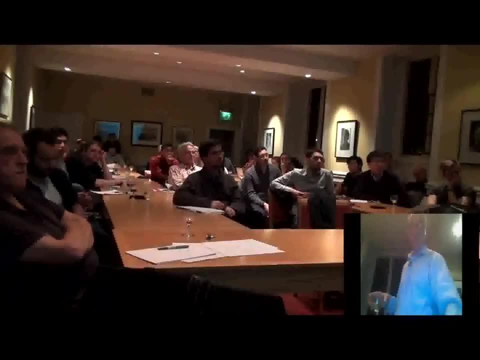 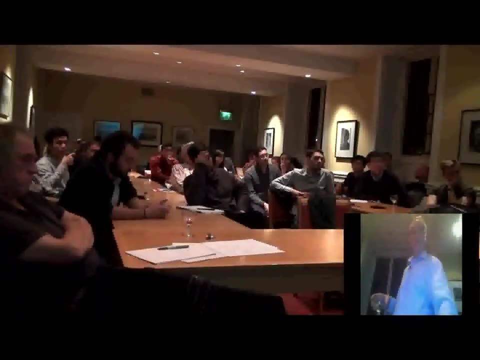 but they're incredibly fragile because they can't roll over their debt, their history, and so is the boom. So that's the verbal model And then you get, ultimately, rising rates can make more conservative projects speculative. You get non-Ponzi investors being forced to sell assets to service debts. The market gets flooded with new entrants, That trend of rising asset prices declines And of course you have loss-making enterprises accumulating losses all the way through. who can fall over when they can't make a debt repayment? And the Ponzi's are the first to go when the whole thing collapses. because they can't sell for a profit anymore and they've got debt servicing costs that exceeds the cash flow they're getting from their businesses. You get an asset price collapse, increasing ratio of debt to equity. Expansion of the money supply goes into reverse. 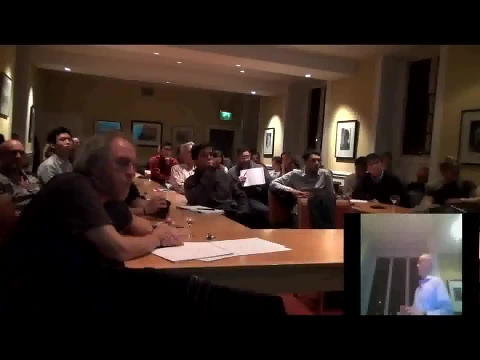 Investment evaporates, You enter a debt-reduced recession, which is where you started. So it's a cyclical verbal model and it's one of the great models in verbal economics. I think the other great model is Schumpeter for explaining cyclical models. 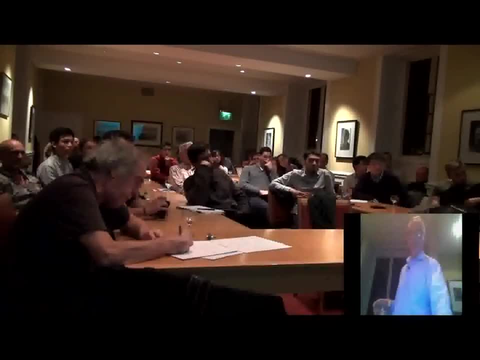 in a model without wipeout prices, like the financial prices that Minsky describes. So modeling Minsky. I start from this proposition, So the natural starting point for analyzing the relation between debt and income. notice, he's also on about debt and income. 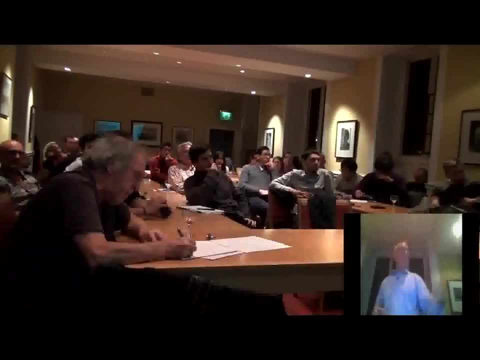 is to take an economy with a cyclical past that is now doing well. Well, I took Goodwin's model of cyclical growth and I added debt finance to it And that's a very simple model saying the level of capital, roughly speaking, the level of motor machinery. 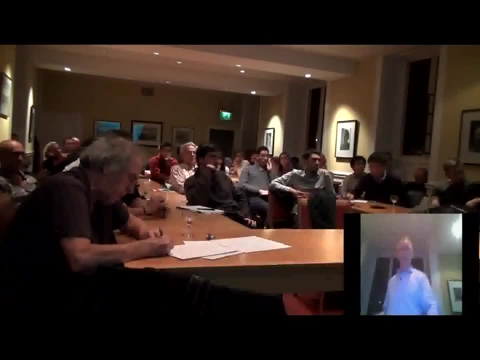 again, this is a measurement issue which needs to be fixed up, but I'm working at the level of a corn economy effectively determines output. Output determines employment. Employment determines the rate of change of wages. Output minus wages and interest payments determines profit. 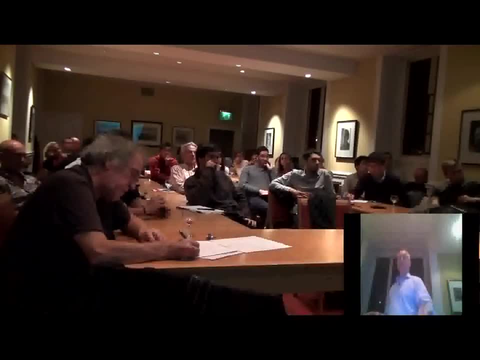 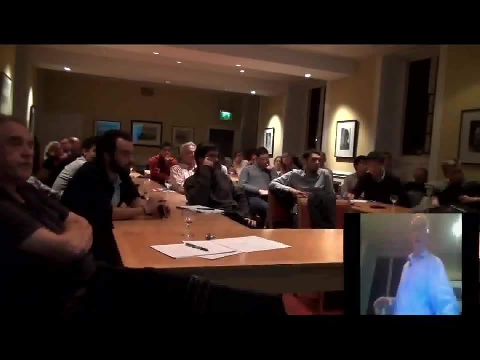 Profit determines desired investment And the gap between desired investment and profit determines the rate of change of debt, And investment is the rate of change of capital. And that's verbally stating the whole mathematical model, And the intriguing thing to me is made by many things. 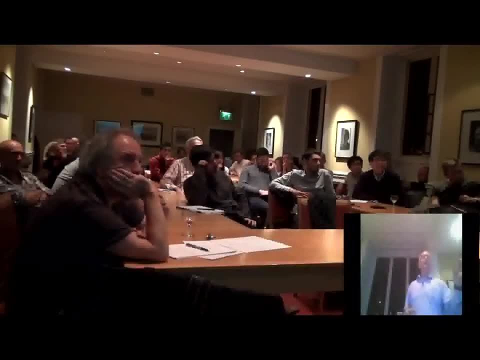 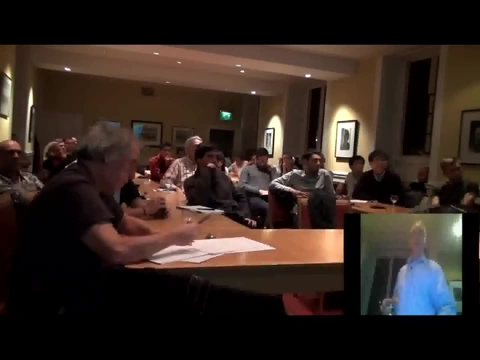 First of all, could I capture what Minsky was talking about, which I did- But secondly, did the model tell me anything that Minsky didn't tell me? And this is the thing which I found quite remarkable, And the more I look back on it, the more remarkable I find it. 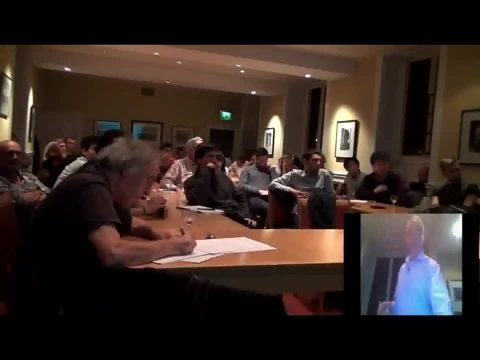 because there were two features I didn't expect in the model and that Minsky didn't talk about, And they were. I'll bring up the model in a moment and show it. First of all, that there was falling volatility before there was rising volatility. 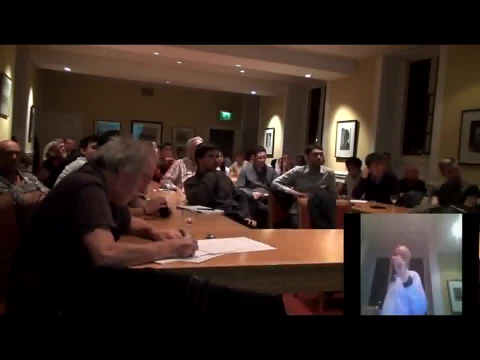 The cycles in employment and the GDP declined for a while. In other words, you went through a great moderation And there was a falling wages share, which, in this model, is a proxy for the rate of inflation. Again, what we saw happening in that period. 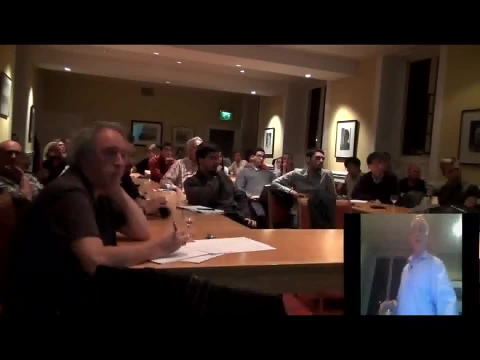 the neoclassical economists patted themselves on the back for. But what actually happened ultimately? And again, I haven't set this up to run properly, My mistake. I'll bring that later in the conversation, during the discussion, if you like. 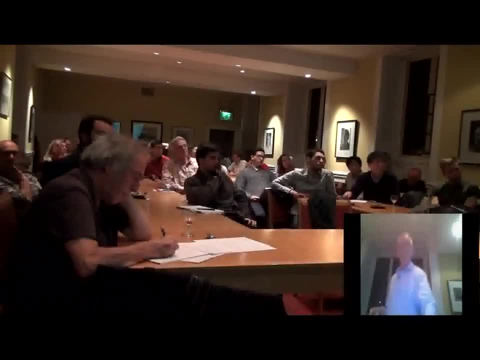 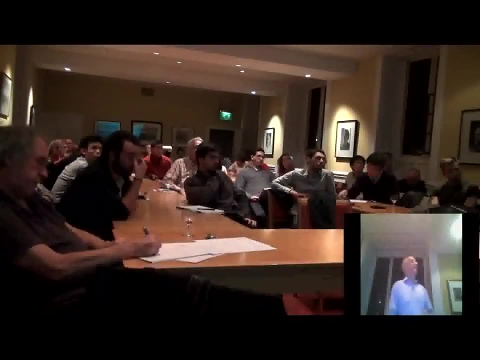 But those are two features that the model gave me that you could not find in Minsky's verbal logic. So I developed the paper before the neoclassicals double S there and invented the great moderation, And it motivated me to write a rhetorical flourish. 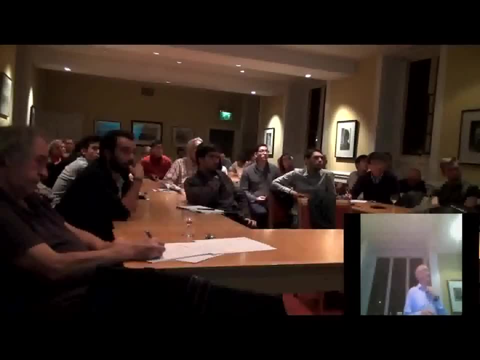 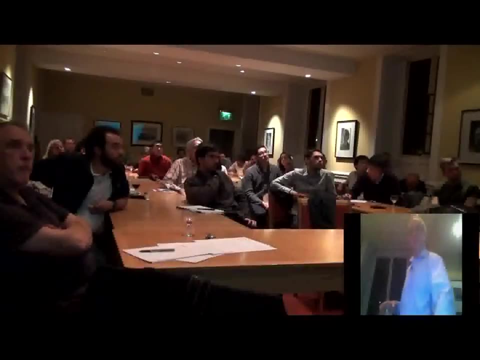 at the end of my paper in 1995.. And I said from the perspective of economic theory and policy. this vision of a capitalist economy of finance requires us to go well beyond that habit of mind which Keynes describes so well: the reliance upon a stable recent past. 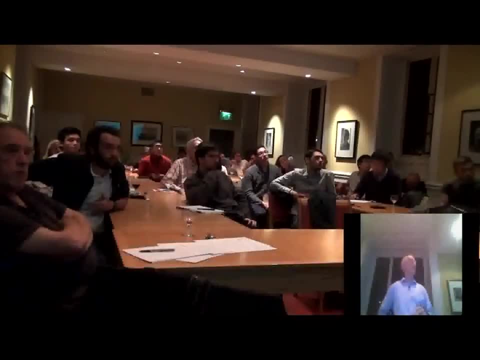 as a guide to the future. This is the rhetorical bit. The chaotic dynamics explored in this paper should warn us against accepting a period of tranquility in the capitalist economy as anything other than a lull before the storm. I thought that was a nice way to finish a paper. 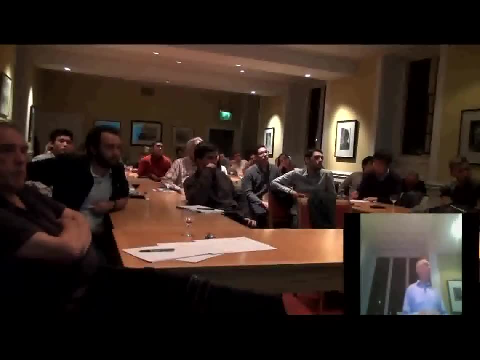 I didn't expect it to become a reality. Now. Bernanke, on the other hand, 2004, talking about this, looking backwards at this period of so-called great moderation, patted himself on the back for saying that it was better control of inflation. 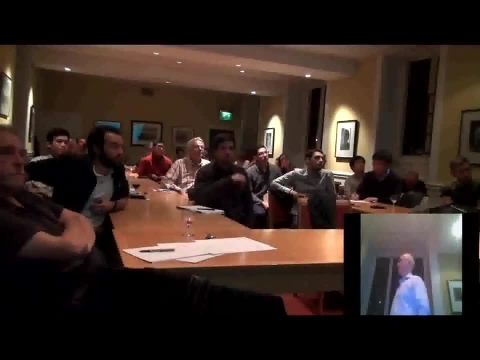 courtesy of monetary policy by central banks that has contributed to this welcome change in the economy. Well, so much for that. That's what they saw: falling volatility- but of course, what then happened was that rising volatility? And, of course, what they were ignoring. 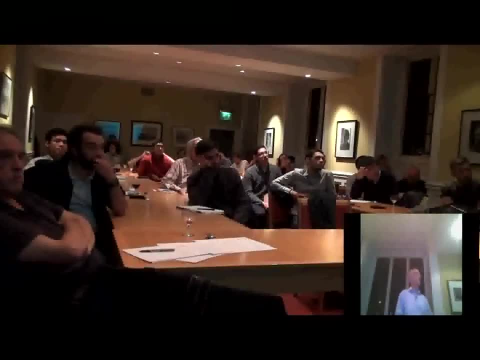 was the level of private debt. When you look at the level of private debt, which they say should have no significant macroeconomic impacts, that's what they missed: this rising ratio of private debt to GDP which is driving the whole process. So that's a simple model. 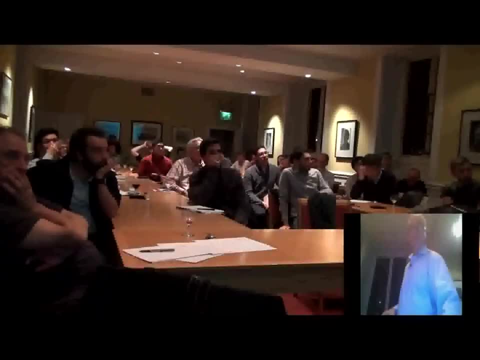 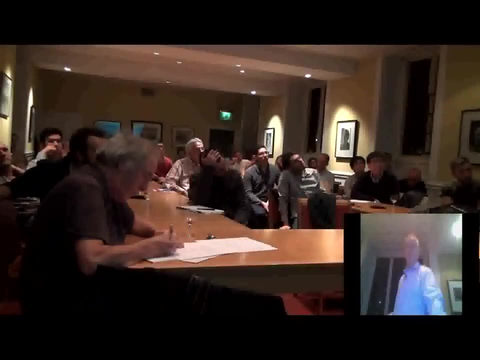 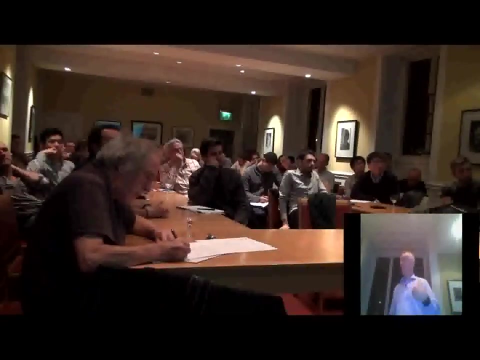 that made predictions that turned out to be correct, And part of the problem is that a verbal model simply can't follow all the feedbacks that exist in a complex system, And therefore I see the type of mathematics I'm doing here and that people like Carl Chiarelli do far better than I do. 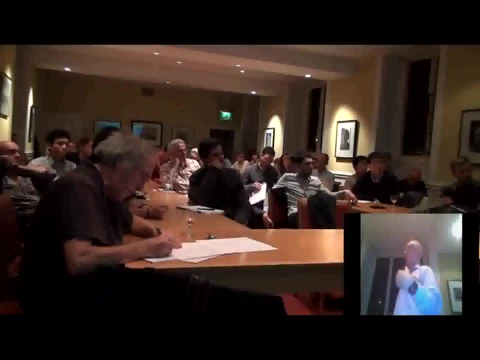 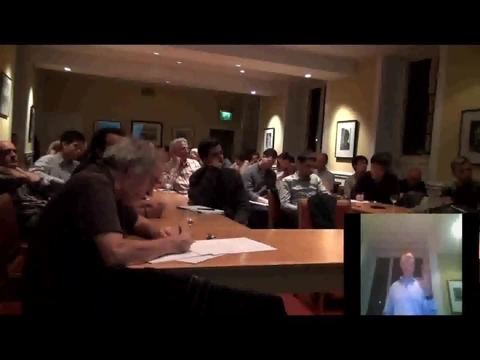 as qualitative mathematical analysis. You're not trying to get quantitative predictions, necessarily. You're trying to qualitatively describe a system using mathematical tools. So you're not after this ridiculous attempt to forecast the future accurately, but you're trying to describe the qualitative behaviour. 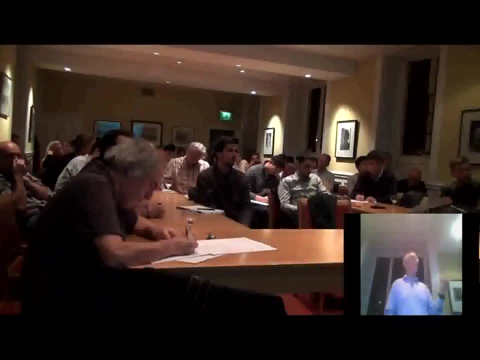 of the economy accurately and out of that get some sort of guide to what might happen in the future. So I see this putting the verbal differential equations of the great non-equilibrium economists, of whom I see Minsky and Schumpeter and Marx. 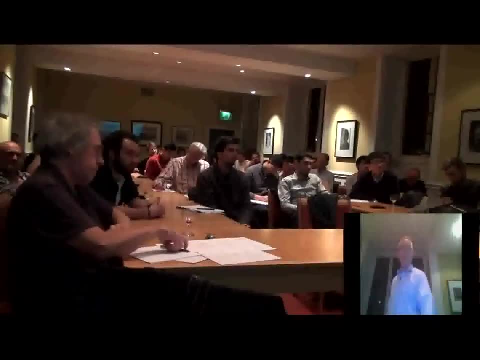 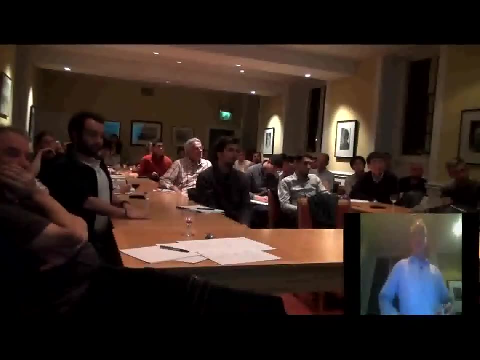 as the major ones in a mathematical form. And of course, ontological issues still abound, because we're modelling human behaviour. And of course Hayek will tell me that I can't model human agency. Yeah, but also I'll remember Marx on this point. 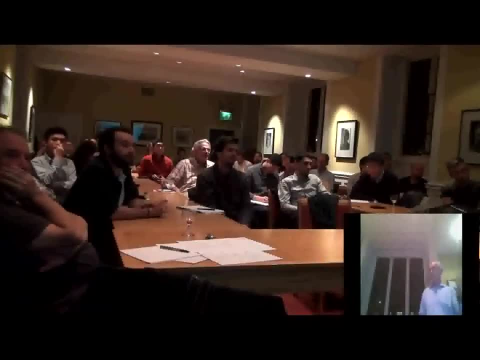 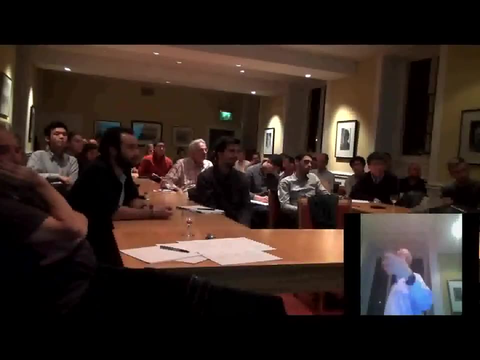 who said that men make their own history as they please. They make it under you know, circumstances forced upon them already existed and given and transmitted from the past, And partly what you get then in this complex system is the dynamics of those structural effects. 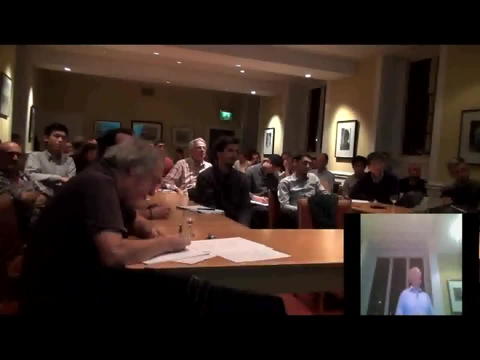 of the existing economy. Now, that's a case for mathematics. What about those who say no, no matter what? Well, I think in some ways we really see our status in life. We can maybe rather too caught up in our own obsessions. 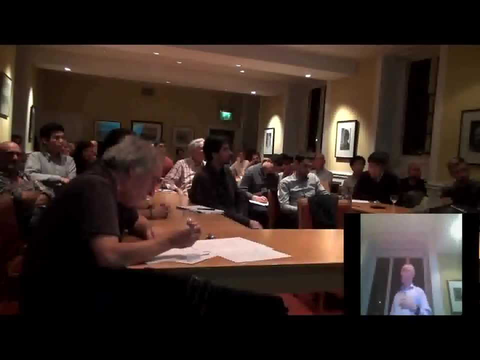 and talk about our importance from the point of view of economists alone, But ultimately, what are we for politicians and for most of the public, We read chicken entrails. We're the alternative to the soothsayers and the witch doctors of the past. 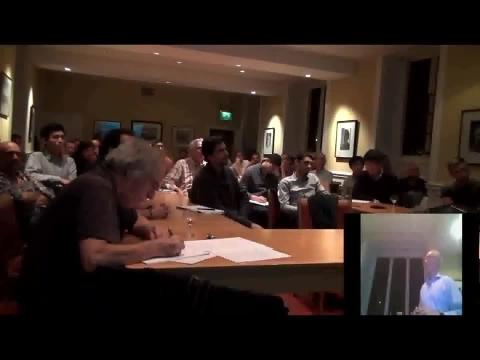 because we provide numbers, soothsaying numbers that politicians can read out in front of press conferences, predictions about the future. And if we don't do it, the neoclassicals will keep on doing it Ontologically false, whatever else. 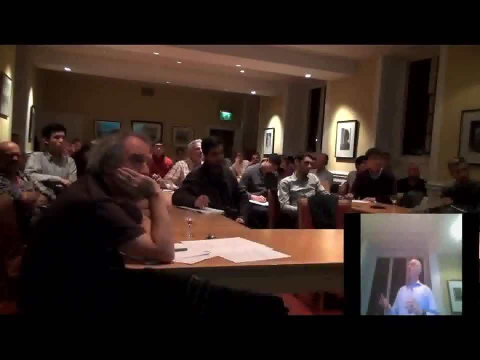 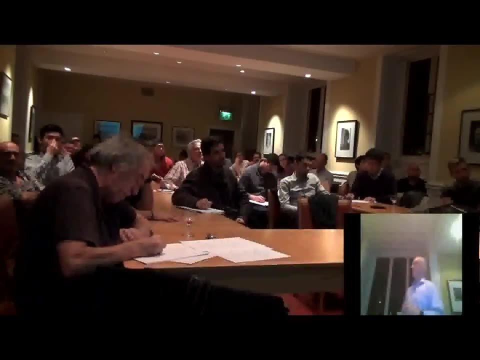 but they'll keep on doing it. So we'll lose the academic battle because we concede the biggest practical function. forget that in inverted commas for good reason, but the biggest practical function we concede to the neoclassicals And I'd rather say it's become: 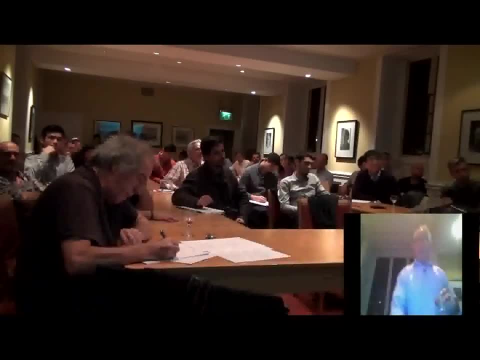 the weathermen of economics, in the sense that everybody wants good weather, especially in England, but nobody expects the meteorologists to forecast good weather. after a storm, You know it's going to get bad again. People inherently accept the weather is cyclical. 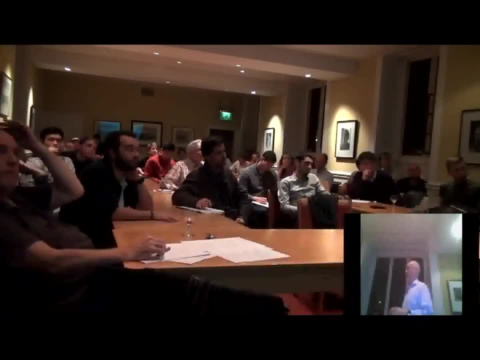 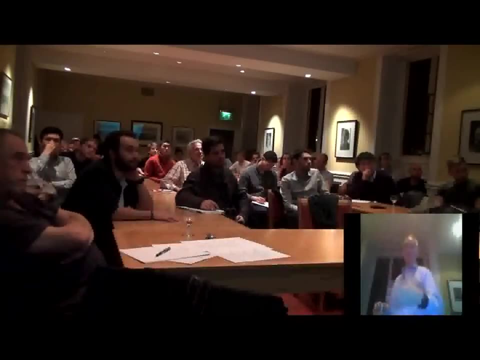 This wonderful weather I've been enjoying in London for the first four months of my time. I know it's not going to last. I'm going to enjoy it while it does. So. we need to achieve the same sort of realism for economics and the same acceptance. 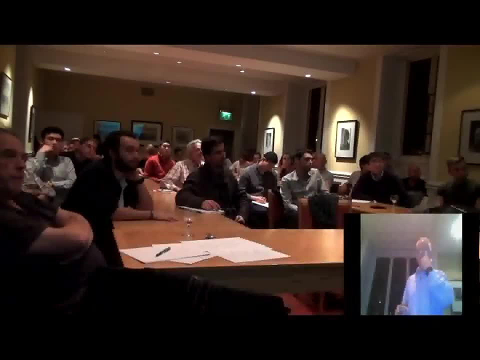 that the economy is cyclical, Prones crashes, booms and slumps, And we won't get that for economics if we cede control of mathematics and abuse of mathematics to neoclassicals. We'll always remain a protest group when I think what we should endeavour to become. 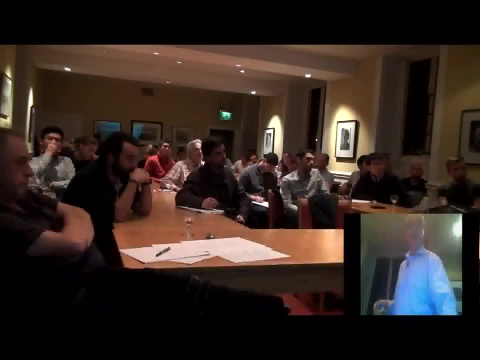 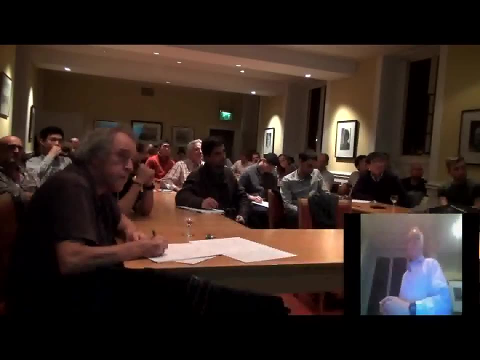 is the mainstream. I'm not willing just to remain a protest about the neoclassicals. I want to eliminate that Interesting but dated theory of economics. So I really see economics as an anti-mathematical discipline. It's myth-o-matics, as I said earlier. 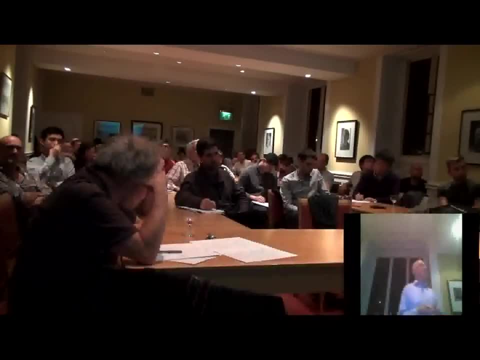 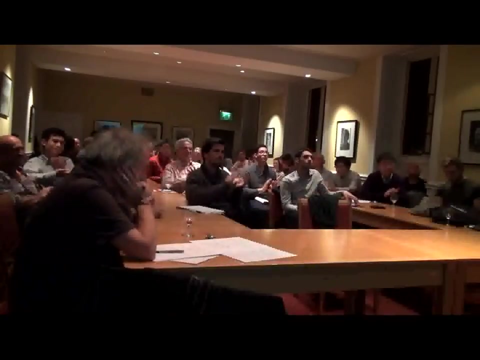 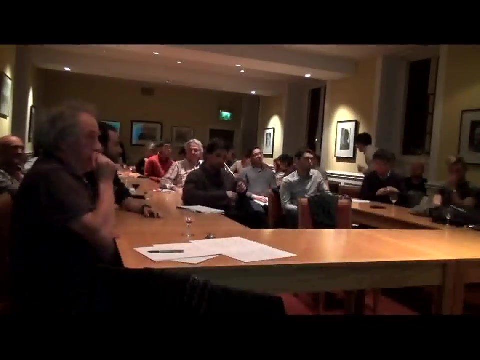 not mathematics. That's the real problem in economics, And my opinion of mathematical economics is rather like Gandhi's supposed opinion of Western civilisation, that it would be a good idea. Thank you, OK, Right, Say that you had a bit of a personal point. 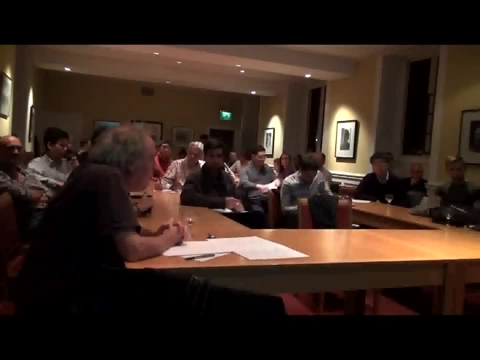 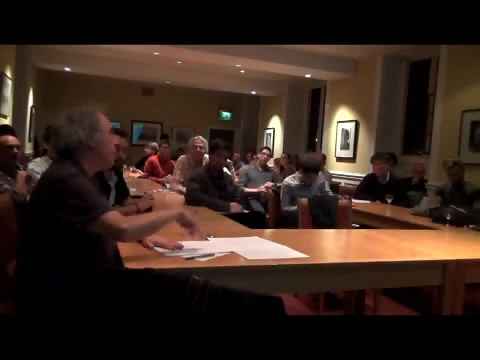 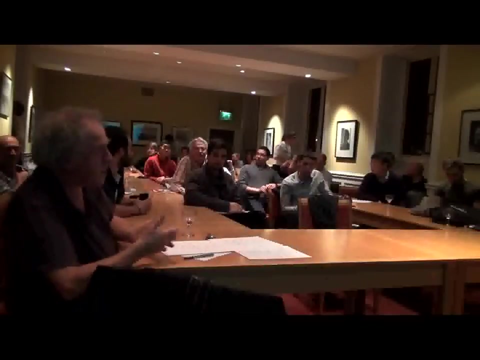 Right? Well, there's a lot there And I'd like to- I'm trying all the time to put my finger on what I think is a fundamental point. I mean, there's bits chucked in like correlations, the fact that you've got a prediction correct. 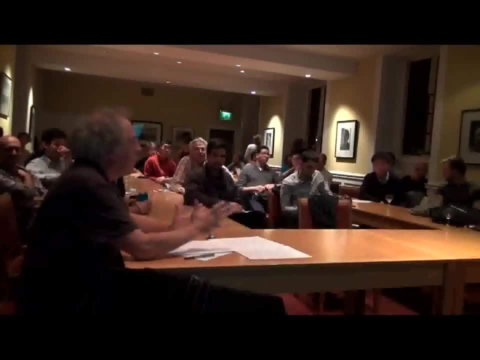 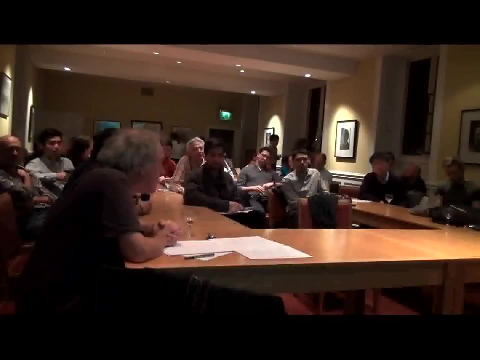 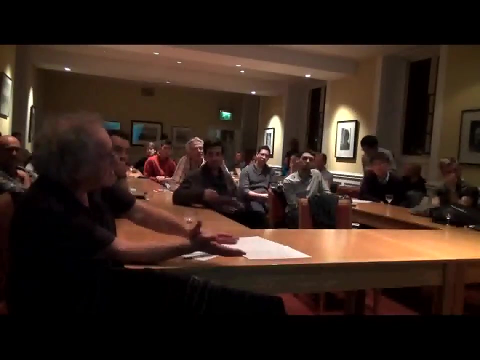 which could happen by accident. Of course, The most persistent feature is: isn't it or is it that you're saying there are certain phenomena, either observed or desired, properties that are desired- that various forms of mathematics have failed to capture? 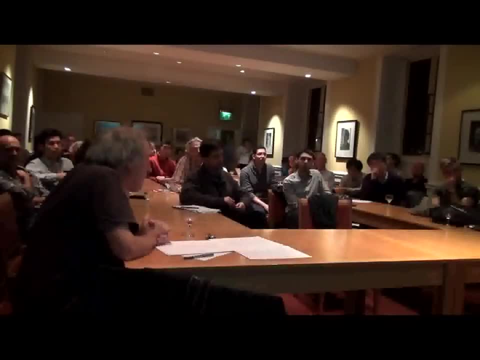 and you are putting forward an alternative form of mathematics that can capture those features. I wouldn't say I'm putting forward mathematics and not an alternative one, because I don't think the neoclassicals have put forward the alternative form, which is why I call it mythematics. 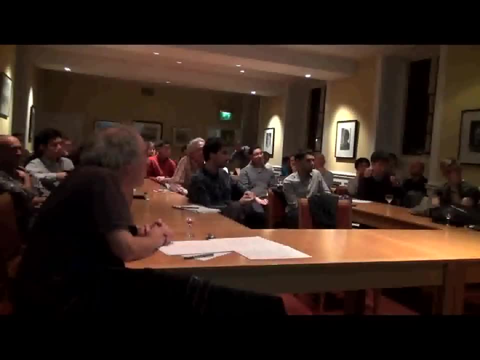 Right, Because if they'd actually done their mathematics properly, you wouldn't even be having this debate. You wouldn't be a minority. But you're correcting mathematics or replacing mathematics, or Using mathematics correctly, Right Yeah, And also using appropriate mathematics. 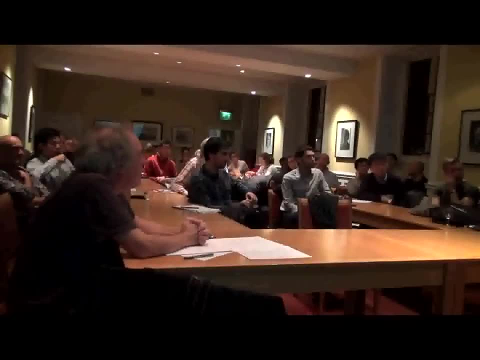 The other thing I'll say about neoclassicals is: nobody else models the economies, models the dynamic system as a succession of equilibrium points, Right, So the equations of equilibrium. only in economics does that happen, And that's why I call it mythematics. 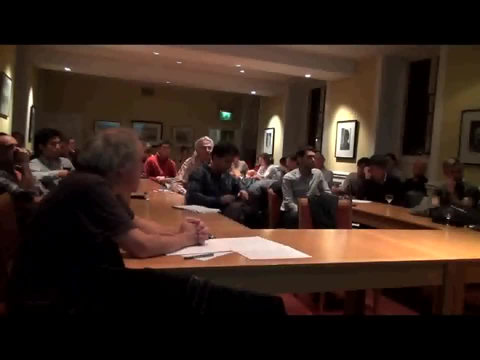 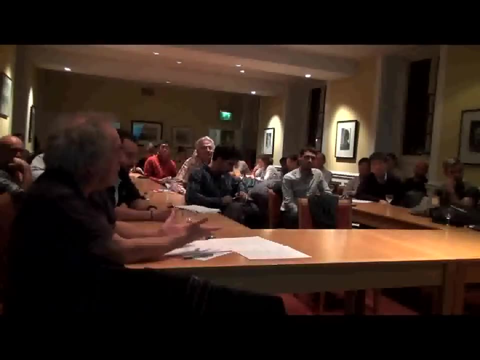 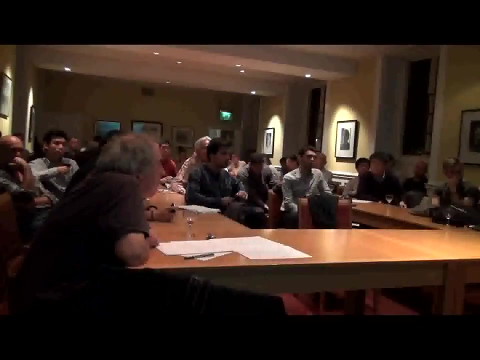 among one of the many reasons. But your criterion of success is that you can accommodate features that the mythomathematics cannot accommodate, generate, And also that I follow the logic of what the mathematics conclusions reach and I try to make the mathematics ontologically correct. to begin with, 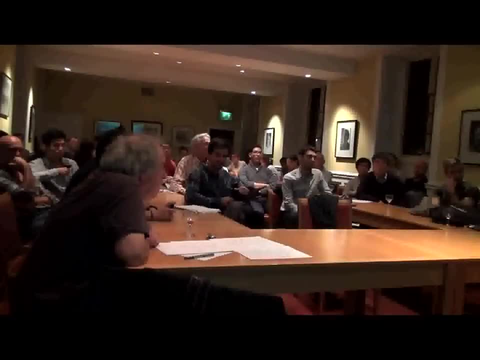 Right. Is that enough? It's an improvement. It is not enough to mean that mathematics will now be magical and get everything right and economics can be solely mathematical, because the great I mean to make my way of thinking- the great insights in economics. 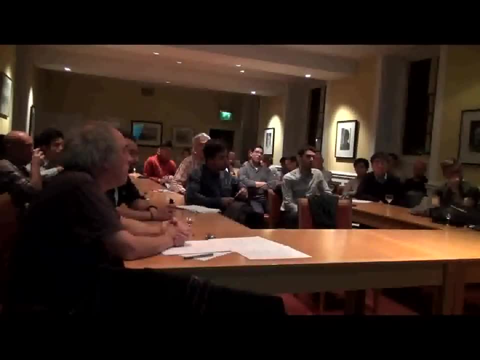 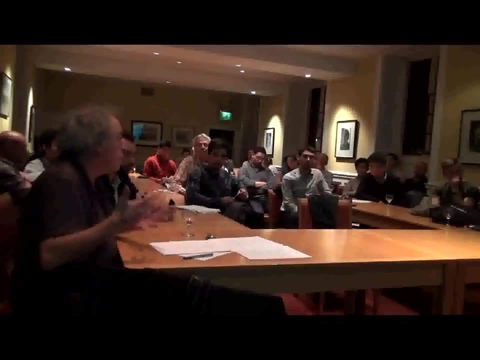 have come out of the people who didn't try to use mathematics: The Schumpeters, the Marxers, the Metzgers and so on. Indeed, you've admitted that you've tried to mathetize, or you've mathetized the insights of others. 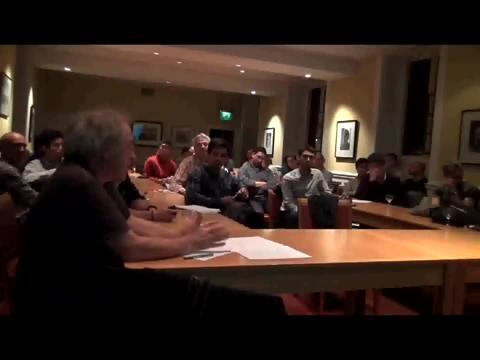 Yeah, I mean supposing. I want to accommodate the insight that all ravens are black. All ravens are black. I can do that by assuming all ravens and vegetables and all vegetables are black and I've accommodated it. 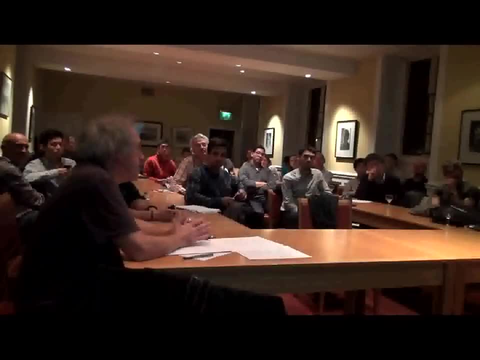 You know there's another model which can't generate. all ravens are black. Have I made it in advance? You're calling a raven a vegetable. That's very neoclassical. It's false. Let's assume it's a vegetable. 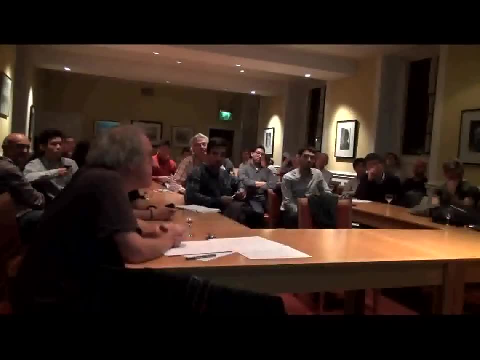 It's false. It's false. Yeah, I know it would be a false statement. So you've got to be starting from true propositions to begin with. Absolutely, If you're not starting from those, you're going to have to start. 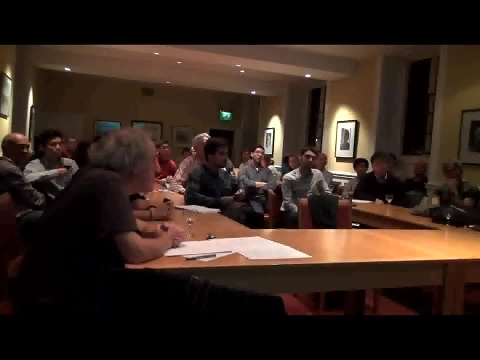 from something else. Yeah, So you've got to be starting from true propositions to begin with, Absolutely. If you're not starting from those, then you're going to produce a false, no matter what Right. So that's what really matters. 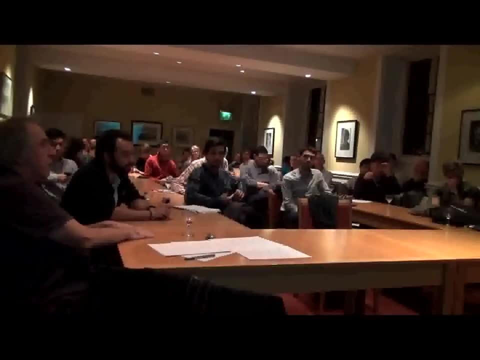 with your models, Not the fact that it can generate properties that you'd like to generate, but the starting points are realistic. Realistic, yeah, Yeah, Has to be, And that things like using risk as uncertainty is an absolute travesty. 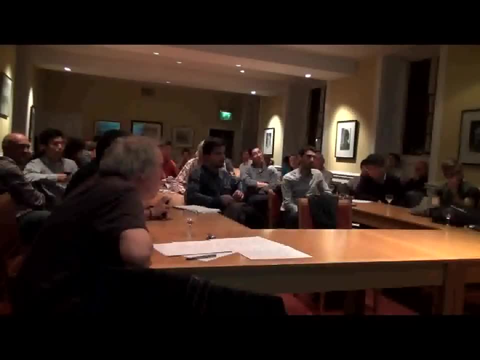 So many things that the neoclassicals have been happy to do that are ontologically false. Have we heard all your starting points? No, Have we heard all your starting points? Are your assumptions all realistic? I mean, I'm sitting there trying, 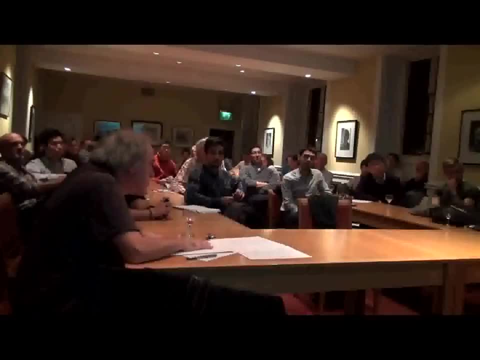 to work out what they are, but In some ways they are, In some ways they are. In some ways they are, As I said, in terms of that model at Minsky I showed you a moment ago, or. 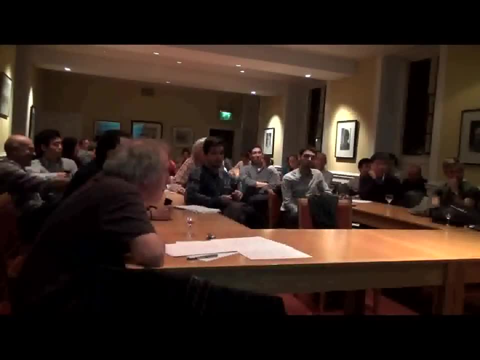 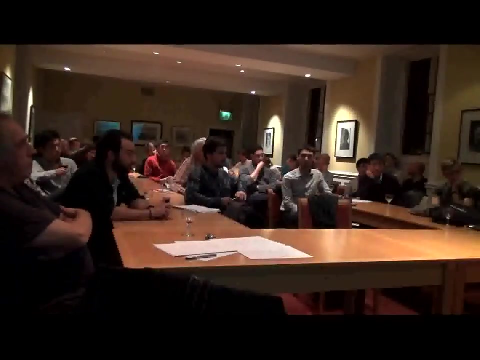 All of them. Let's say that I don't know that they're all realistic, but what guides my thinking about how one does modeling is trying to capture what I think is a realistic description of the system, And when I'm working in microeconomics, for example, it's not realistic to have rising marginal cost. It's not realistic to misdefine profit maximisation. Yeah, It's not realistic to ignore that the real form of competition is Schumpeterian and diversity of products is what defines markets, not 180, et cetera, et cetera. 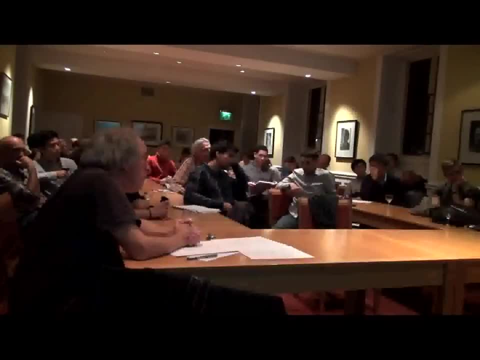 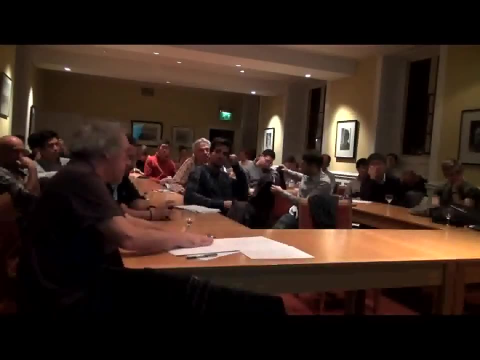 So you have to say: if we're going to try any modeling at all, let's start from a realistic perspective. I know The if bit, Yeah, But all your assumptions render the system deterministic. I mean you might- No, no, the deterministic, the deterministic. 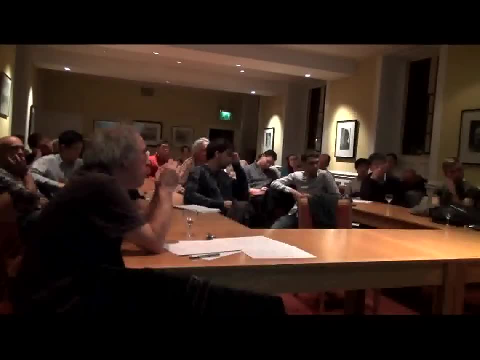 models. the models I've shown you there are deterministic, but they're also non-linear and non-ergotic. That's right. This is one thing I couldn't get through to Paul Davidson ever. Maybe one of these days I will Right. 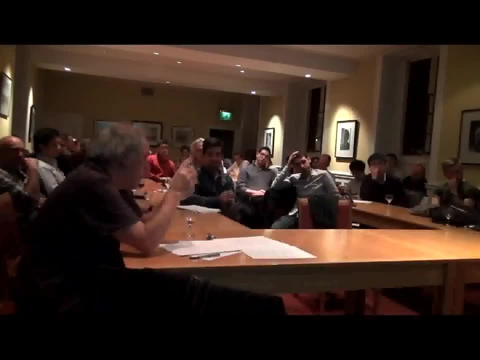 You pointed out, if you change the starting point a little bit, you could blast off to your words. But if you go back to precisely the same starting point twice, three times, you always blast off in the same direction. If every last element of the system is the same, 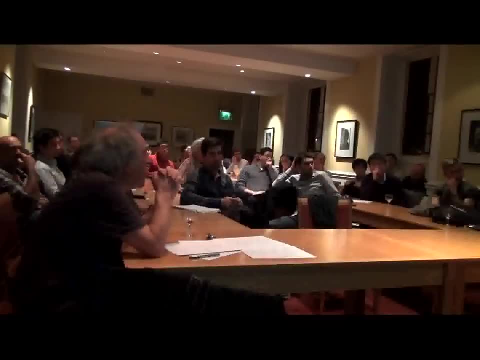 Right, Of course. the reality is there's no such thing like there ever to happen in an economy. No, The economy is always changing. But do you think human beings are such that if we ever did go back to the same point, we'd always go off in the same direction? 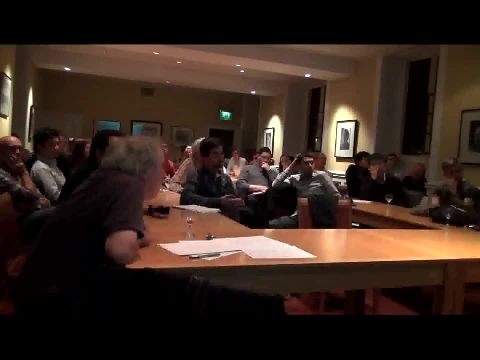 No, because then you get to where human behavior can't be properly modeled. Somebody might make a different decision and therefore there'll be a different outcome, But it's still the argument that Marx made Men make their own history, but not in circumstances of their own choosing. 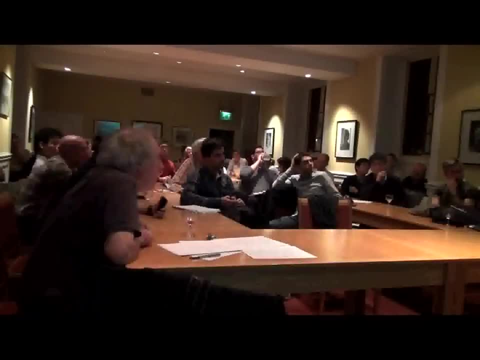 Yeah, The word makes sense. Circumstances play a major role in shaping what it's likely to do. So if, by sheer chance, a couple of hanging chads hadn't hung, and we had a couple of hanging chads that didn't have George W Bush as president of America, then we would 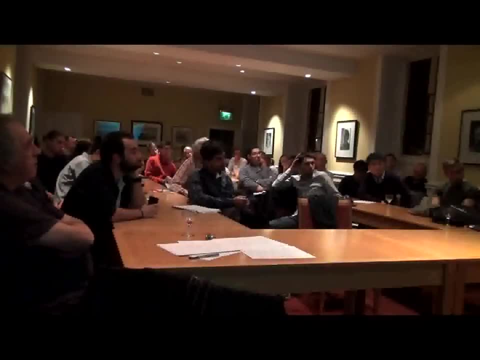 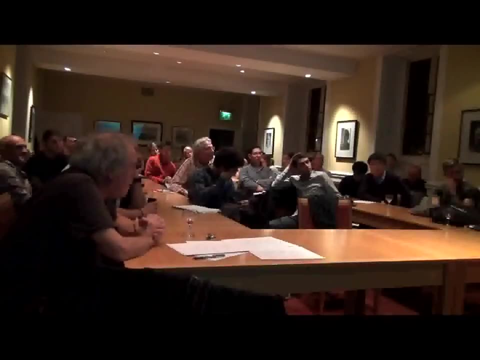 have had somebody who would not have invaded Iraq. the world could be entirely different if a few hanging chads hadn't hung. You don't have to convince me of contingency, Yeah Yeah, But nonetheless we would still have had the other events around that. 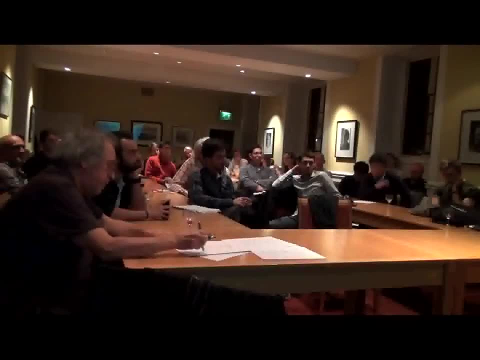 Right. So yeah, the persistence will vary, but it's the structural forces that give you the overall shape of change. That's what I'd like to capture in the modeling I do. Yes, I mean, I don't want to go on forever, but how do you avoid atomism, for example? 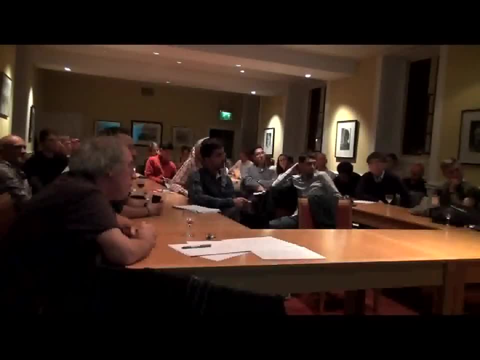 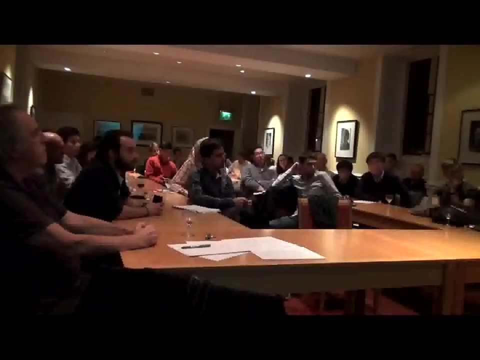 Atomism. well, that's avoided by just denial of reductionism. When you have complex systems, reductionism doesn't work. Atomism is a necessary outcome of the reductionist mindset, If you believe that the sum. That's where May's point about. 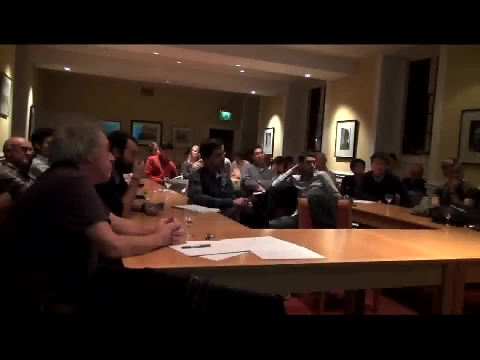 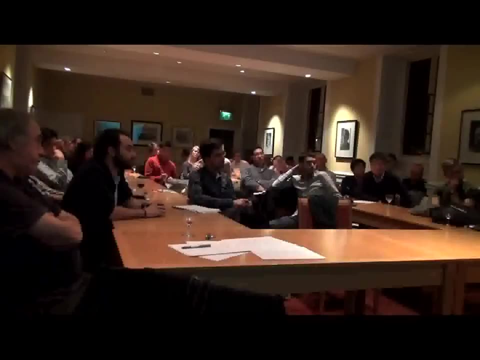 Oh, not May. Anderson's point about constructivism is really important because he said: even if reductionism, If you believe reductionism, that doesn't mean that you can rebuild the universe by getting out of the atoms and adding them up. 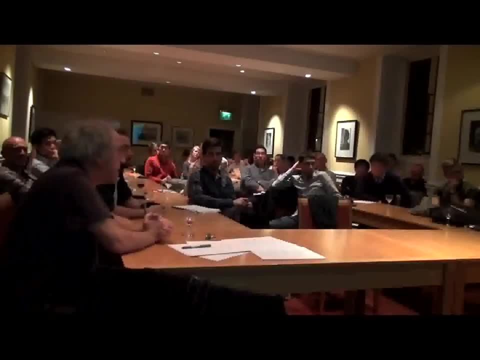 That's Sure. I was thinking more of Keynes' notion of atomism, basically, and the conditions that show us do the same. Why I think On that front I think Whitehead was probably better and he's talking about organicism. 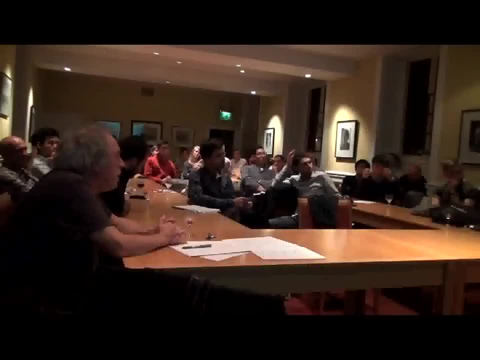 I think Keynes didn't go far enough on his philosophy and the arguments that Whitehead made about organicism are predecessors of the type of complex system we see today. So I'd say Keynes has been deficient on that atomism approach. Yeah Well, he was criticising it. 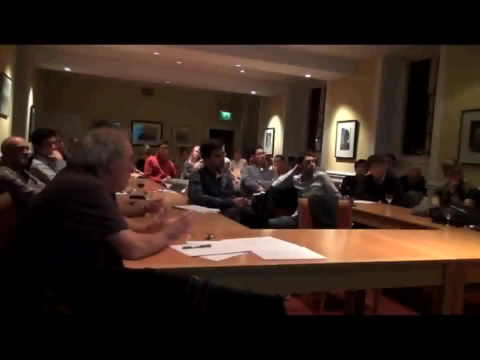 He was using it to criticise econometrics. Oh OK, Oh yeah, yeah. yeah, That was just. It was No, but OK, But that notion of an atom underpin This implicit ontology of your simulations too. no, 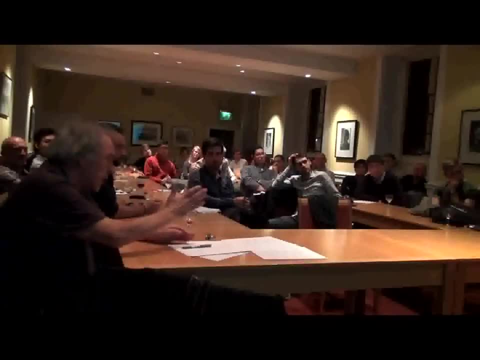 No. Well, when, However complicated your nonlinear equations, whenever x- this starting point after 10,094 iterations, I'm at y. And if I go up to the same starting point after 10,094 iterations, I'm at y. 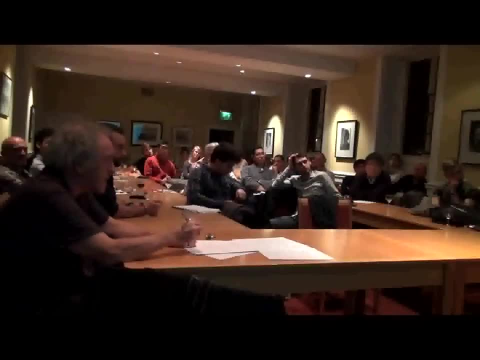 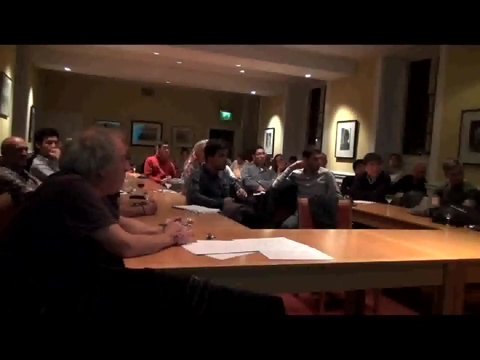 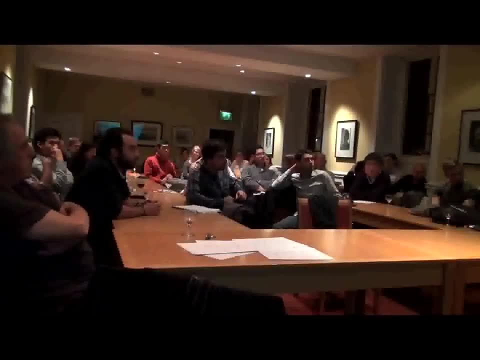 his model back in the days when computers were primitive compared to today, got the results as a set of tables and asked the technician to re-enter the numbers and start the simulation again. The printout- The printer worked out four decimal places of accuracy. 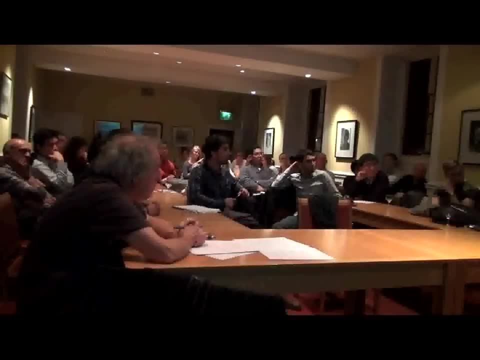 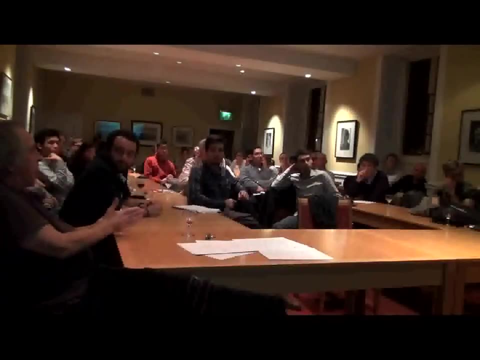 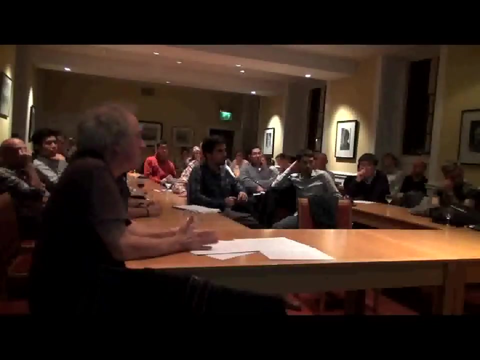 And now look at the. Yeah, the computer worked at six so that I typed in the four decimal points and got a completely different pattern. okay, that's because the starting point changed. the starting point changed by what we regard as trivial differences. you know, I understand that property of nonlinear equations, but still the ontology is an. 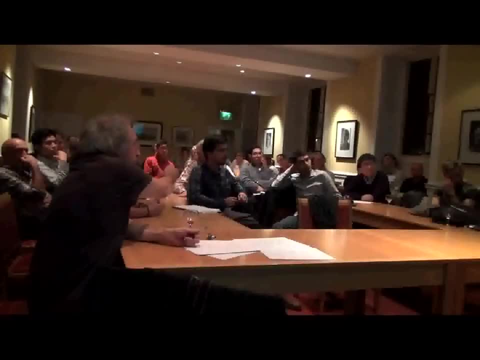 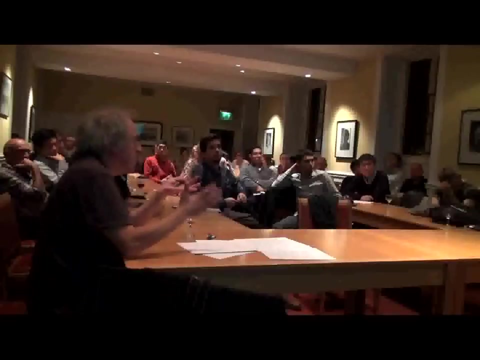 atom if you've got the exactly same starting point. exactly the same atom. exactly the same starting point requires infinitely accurate same starting point. that just isn't the real world, right. but if you did have it you would get to the same thing. I mean, it's not the ability to get. in that case I 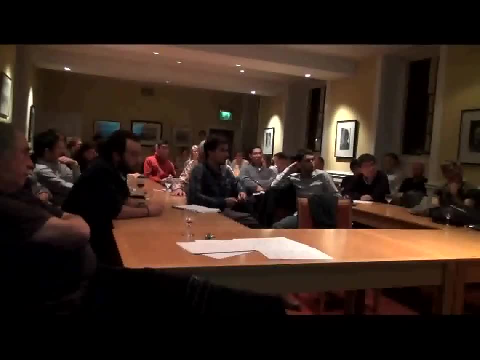 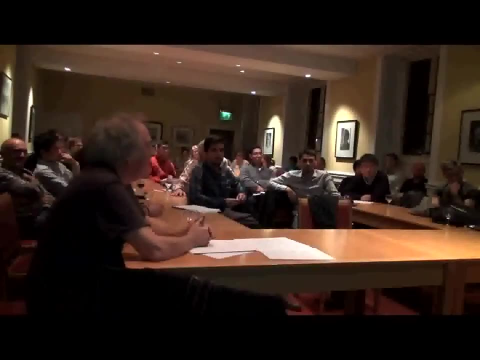 mean, if that's the major objection, then you whack. if you whack in a tiny stochastic term, but there's a fundamental difference between a reductionist, atomistic, linear and a nonlinear system. they're totally different worlds. so you, as Lorenz argued himself in that paper. he said that people think that to get 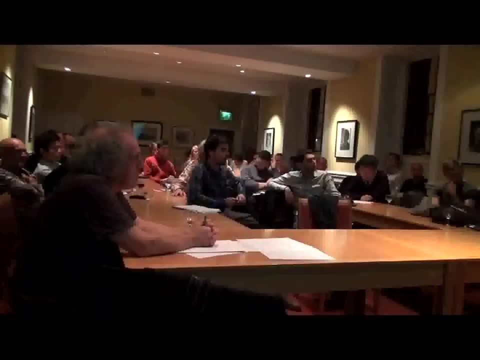 a periodic change, you must have forcing or shocks from the outside. and he said: no, it's just nonlinear relations alone that give you those aperiodic cycles and also you can't forecast them all in a very limited time period ahead. you know you don't have infinite accuracy of measurement as soon as you have an 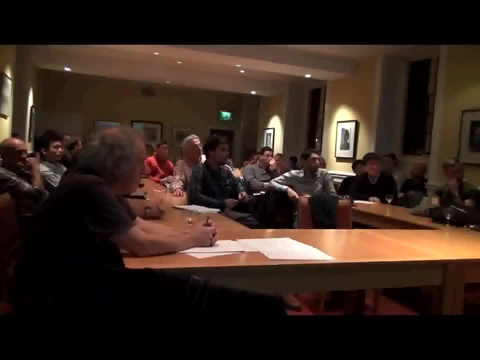 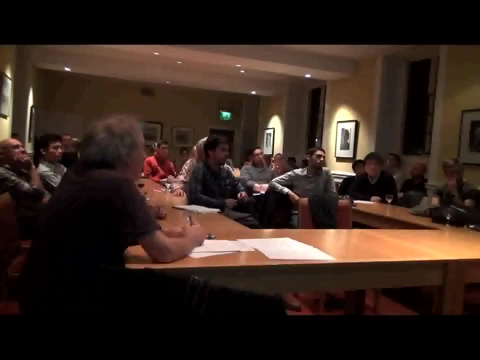 infinite accuracy of measurement. you can't even know whether you are or are not at the same point. so if you were to be able to rerun your experiment, you'd need to know the world. infinite accuracy, I mean everything in the location of the next point on the planet I'm trying to 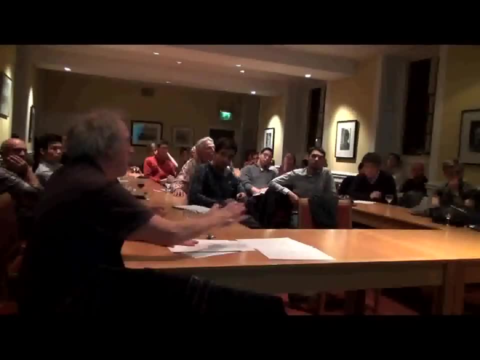 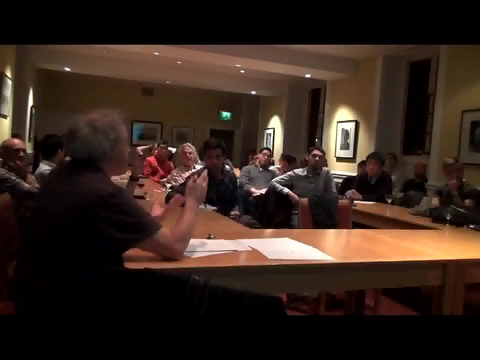 make an ontological question. do you want to go to practical? we go, I don't. I think it's something. at some level of detail, ontology becomes practical anyway. shall one thing, I do it for you. I think a mainstream know where everyone have geworden their anti-mathematics. they think the program like: yes, you think the? 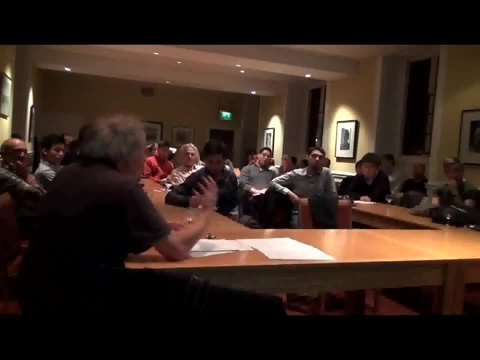 people criticizing anti, but it's along the ground. yeah, people will be calm if they thinkanti mathmatics the problem. but yes, I think the people who put in science are anti, but it's wrongly grounds for it. People defend the proper use of any tool, pro and tort, and we do disagree on the way. 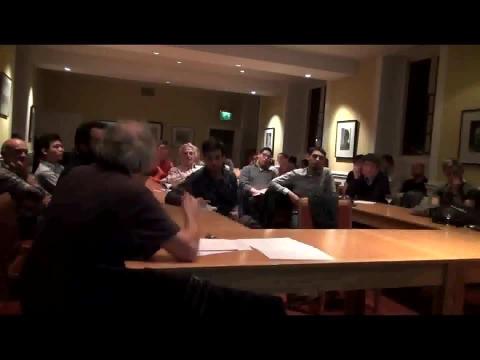 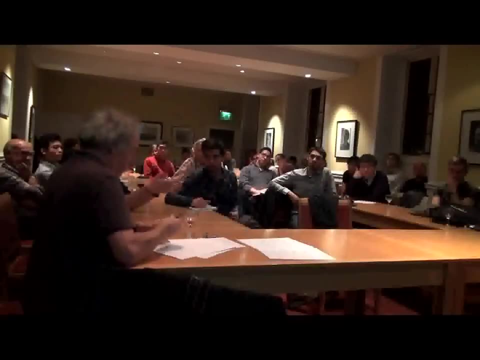 mathematics is abused. I have two questions, one technical and one non-technical. The technical one: I completely agree with the sensitivity and initial conditions, but I was wondering: how do you see your catalysts, given that the tools we use for economics? 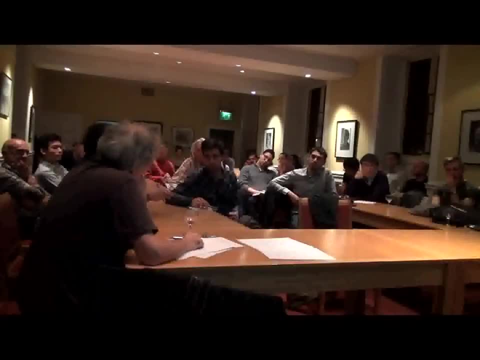 as a science are really unprecise. I think it comes back to that statement that Minsky began with, which is saying that to have a genuine model of economics, you have to have a model in which Great Depression is a possible state of the model. 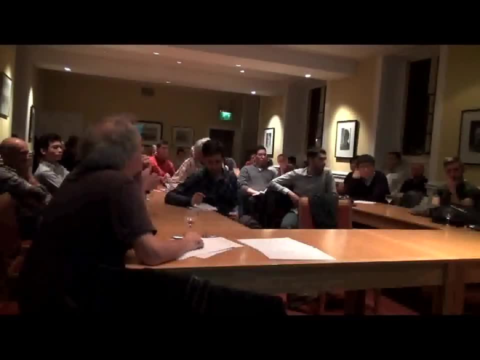 If you have a model that can't generate a Great Depression, you haven't got a model of capitalism. My question was, for example, during the model, for example in Lorenz, if you put the parameters a little bit to the left or a little bit to the right as parameters, you begin with periodic. 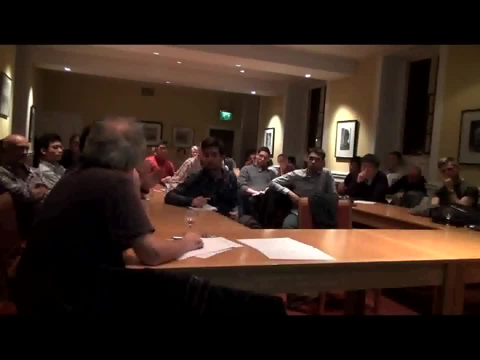 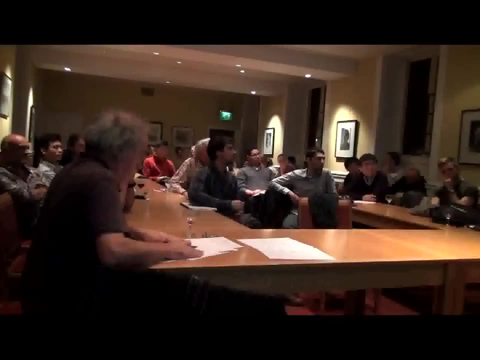 cycles, for example. Yeah, yeah, Yeah, Do you know the precise process? That's an issue that Carl Schiriller discusses a great length in his work, in saying that, because of the sensitivity depends upon initial conditions, you can have basins of attraction. 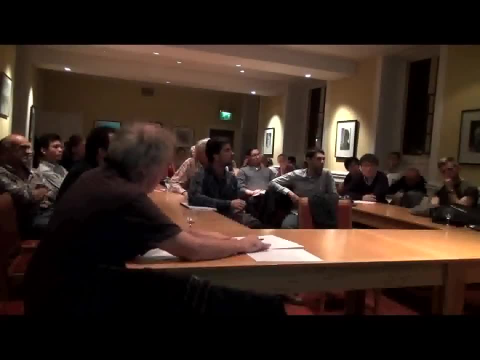 that are stable and unstable and you don't really know how large those basins are. So that is a major issue. But it then comes down to: if you want to assess policy, then a big policy condition becomes: if we make a change to the interest rate settings or the reserve requirements of banks or whatever. 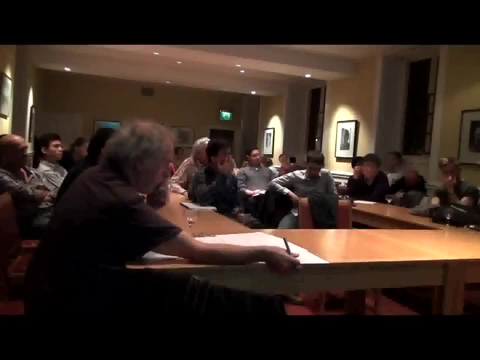 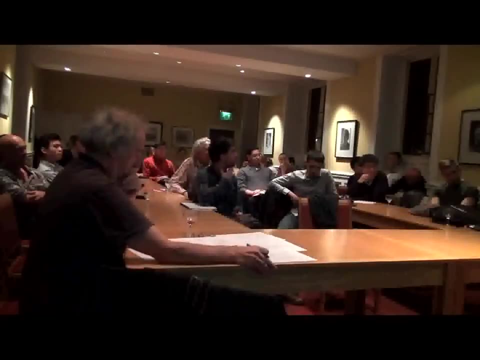 else maybe that will push it out of a basin of stability to a basin of instability. Let's simulate and find out. So it becomes an important issue because to me the only practical, apart from giving numbers that make politicians have something to say in front of press conferences, if we have, 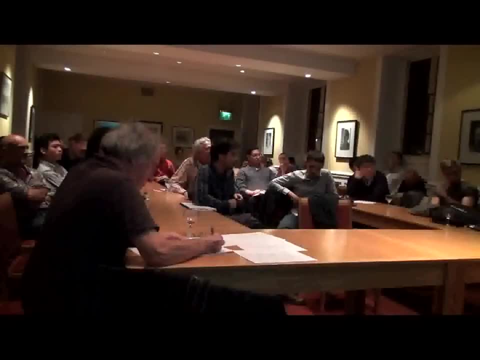 any practical role at all. it's avoiding the calamity like the Great Depression. You don't want to have that system occur again. So you really have to say when looking at the changes you might suggest to an economy or policies to address an economy's current state. the big thing is avoiding a crisis. 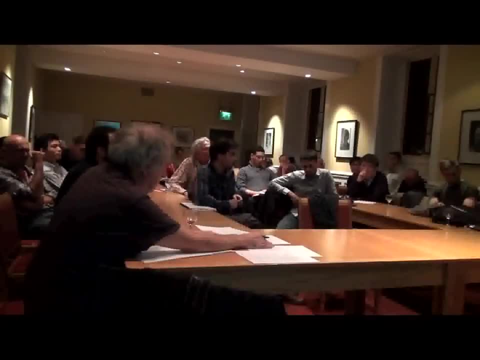 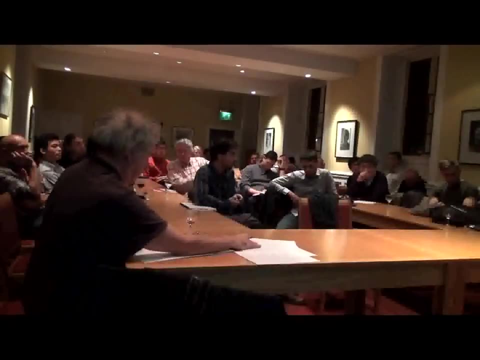 that big, which is destructive of society. So I'm not going to be worried about whether you forecast accurately or not. I'm going to be worried about whether you build a model that you characterise the economy that avoids making the sort of policy decisions that politicians have made in the last 20. 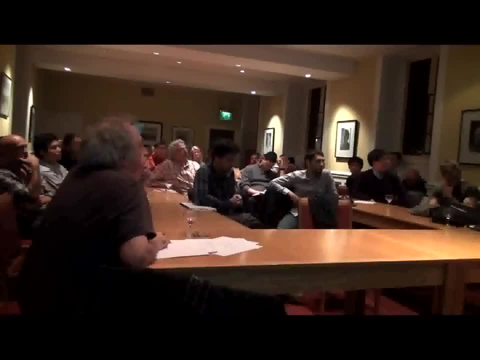 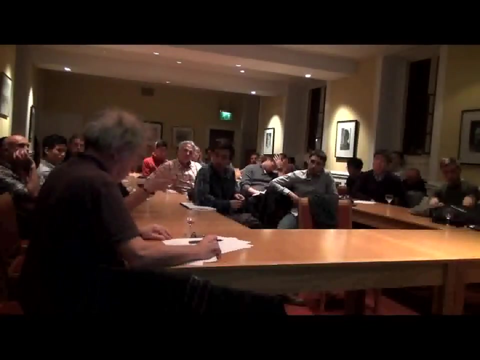 or 30 years which have led to the second Great Depression And the second one, the two, but completely the opposite. Yes, When I read about Lorenz's paper, it was really provocative at the moment because any non-deterministic flow was periodic, but he had the mind relaxed to put it as a title. 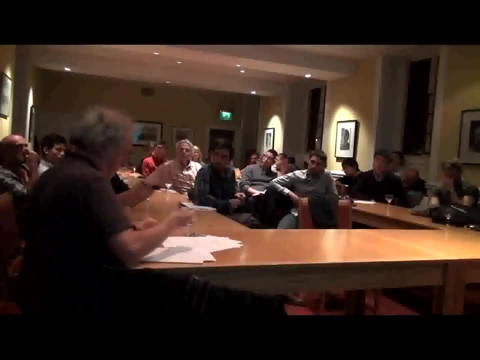 As what is that In the title? He put clearly the provocative sentence in the title, But he was calm because it was math that he was shown. Why do you think that it does not happen in economics, as you suggest? Yeah, I think it comes down to the theological role of the economy. 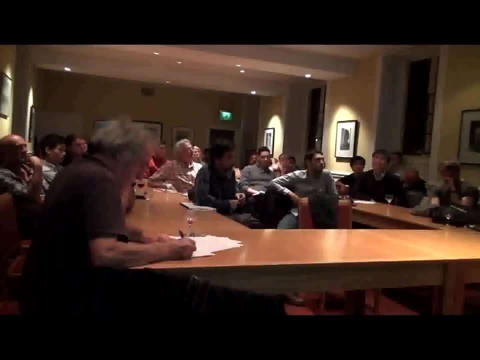 The economists want to reach a set of the majority. the neoclassical majority want to reach a set of conclusions about the market economy reaching equilibrium, And if you show that it's a non-equilibrium system, they don't want to listen to you. 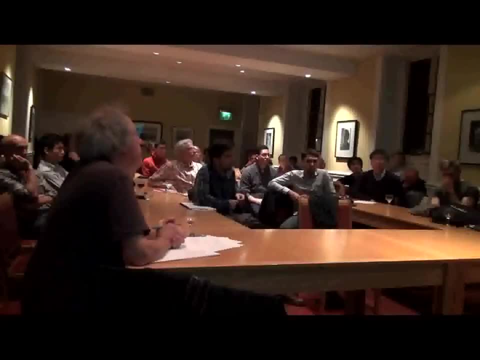 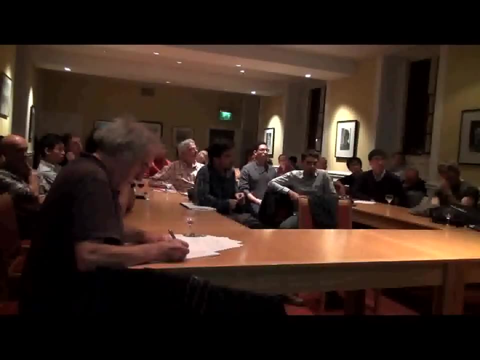 So they ignore this whole tradition, everything that this their area. when you look at neoclassical theory, particularly now with all this DSGE stuff, it's so bloody hard to learn. That's all students do learn And they put so much brain power into it. 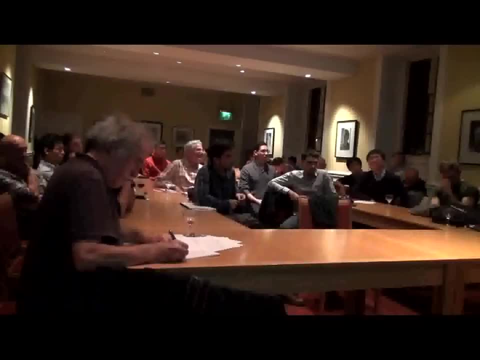 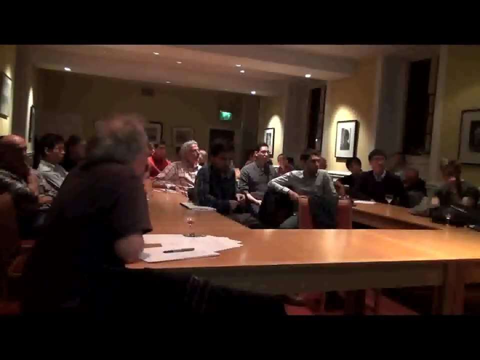 They think it's got to be right because it's so bloody hard, And therefore they reject anybody who comes at them and says it might be non-equilibrium, or banks might matter or whatever else. They just reject. So the way I see it, you have several different classes of models that you discuss. 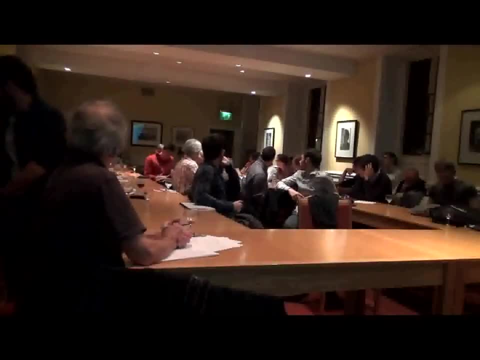 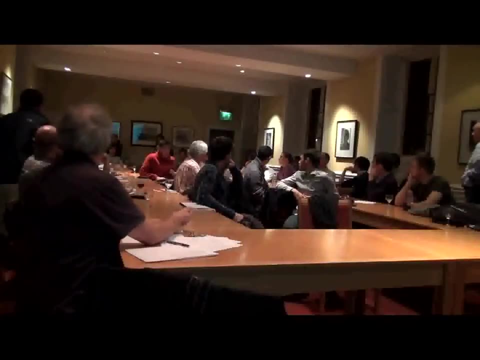 So in what you call neoclassical we have an imaginary possible world given a certain functional form, And it doesn't really come together. It doesn't really contribute much to our understanding of how the real world works. And you have the mathematical criticisms of that, the dual instability theorem, and so 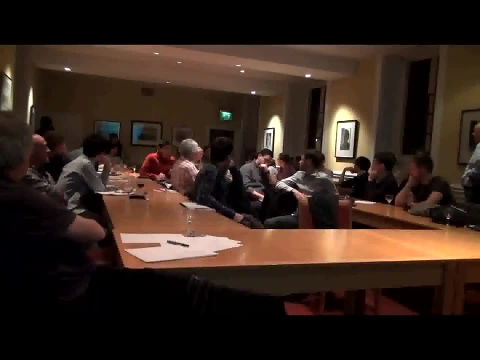 on which show that mathematically, these models don't really hold. And fine enough. I mean, if the point is to devastate their mathematics in order to perhaps show that their conclusions about the real world aren't true, fine enough. Then you have a different type of model, such as your endogenous money model. 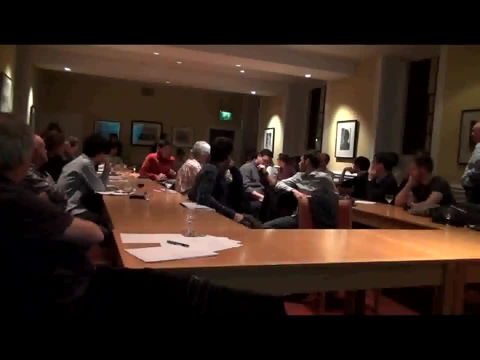 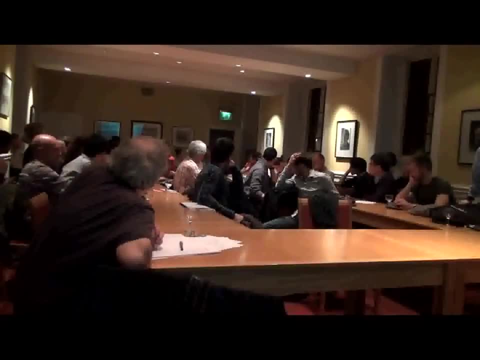 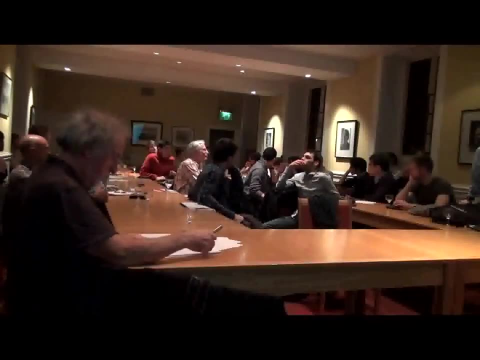 But you said it's not about predictions. It's just showing that in an endogenous money framework It is possible to increase demand by increasing debt. Yeah, So fine. But those models- I see that they actually have an anchoring in the real world. 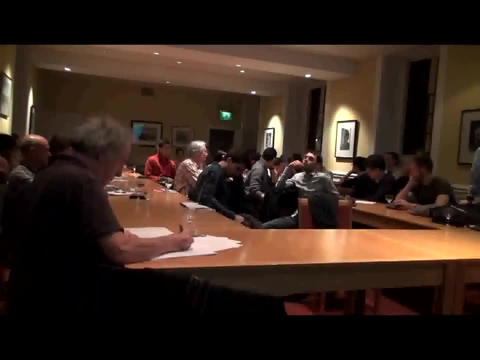 So it's basically an accounting model. That's what I want to note, Dr. Yeah, Yes, But what I'm confused by is what I see as the third type of models. when you mathematize Minsky, I mean if Minsky provided the insights that he did and then you mathematize them. 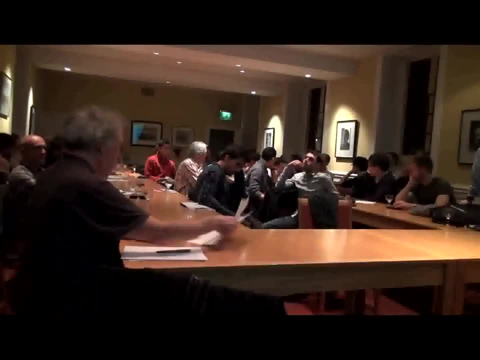 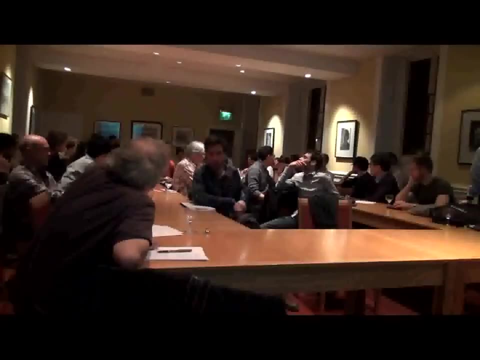 I mean to me it seemed that you said the usefulness of this was that there were these couple of things that happened in the model that I didn't see for Minsky. I mean, had you chosen different functional relationships or flight of different equations for that you could have gotten something else. 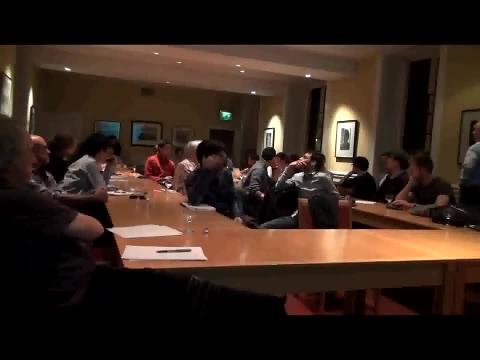 You could have also just looked at the empirical data and read someone else and got the same idea. Oh, Minsky didn't include this, So what's I mean? what is the ultimate purpose, then, of mathematizing the same insights of Minsky or Keynes? 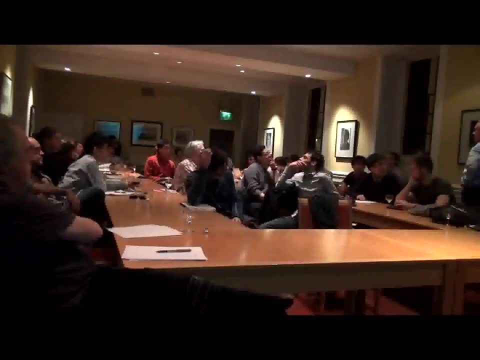 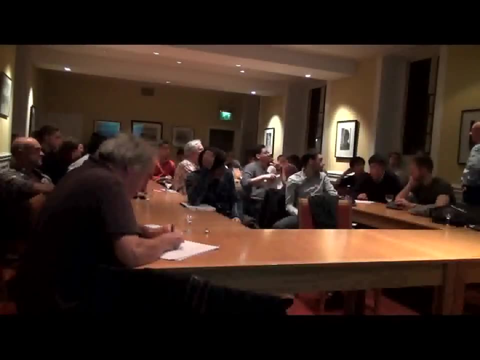 I can't quite wrap my head around that. I think mathematics is an incredibly powerful rhetorical footnote in economics which we're crippling ourselves that we don't use, And the mathematics it drives the rhetoric of economics like no other social science And you can either ignore it. 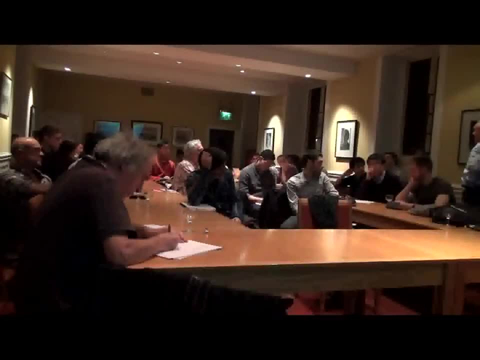 If you ignore that rhetoric, you're going to be ignored yourselves, or you can take that rhetoric over. Now, in terms of that model, could you have seen it in empirical data? No, In fact, Minsky, looking at the empirical data up to when he wrote in the 1980s, was predicting accelerated inflation, which is what happened. 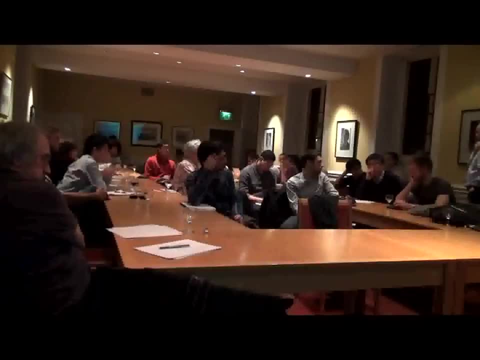 It looked like it could be happening, So that was an insight. I didn't see otherwise. And in terms of the functional forms, a simple linear Phillips curve and linear investment function give you the same cycles. They don't break down because the linear system won't have a- you know an opinion going as much up as it goes down. 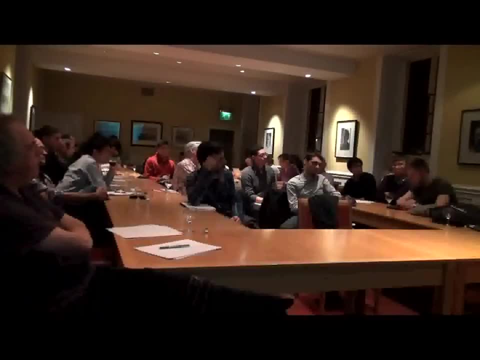 It's unrealistic. But this is independent of the mathematical forms you use, And that again was something I've only realized, not in recent, I've done it some years ago, But when I first thought that I used a nonlinear model because that was realistic, okay. 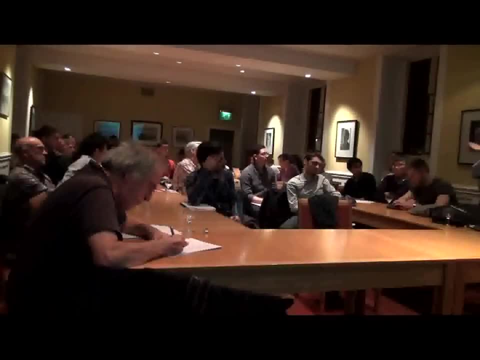 the way, as Phil Phillips himself argued. talking about the Phillips curve he said workers have it's a nonlinear reaction of factor prices to the level of output. He drew that before he did the graphing. If you look back at his system dynamics papers in 1953 and 57, he actually draws in the Phillips curve relationship before he does the empirical work for it. 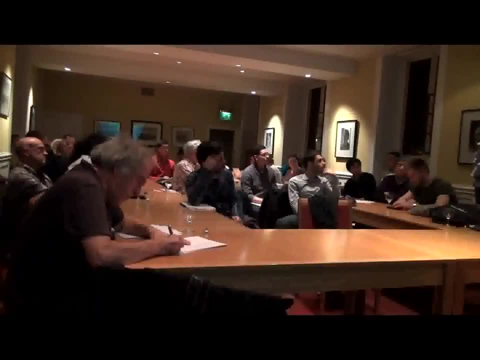 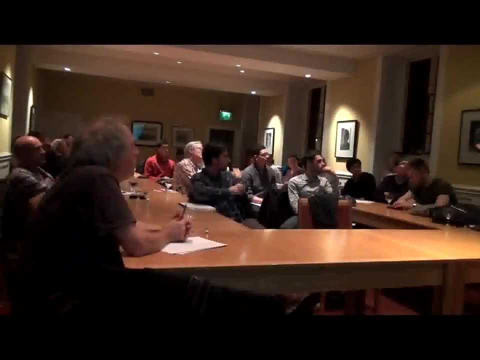 He's saying it's realistic to say that there's a nonlinear relationship. The same thing for investment. What the nonlinear functions give you is they constrain the outputs of the model to realistic values, But the actual behavior of that model comes out, even though they use linear models. 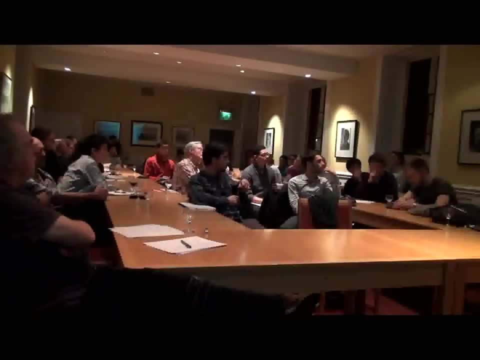 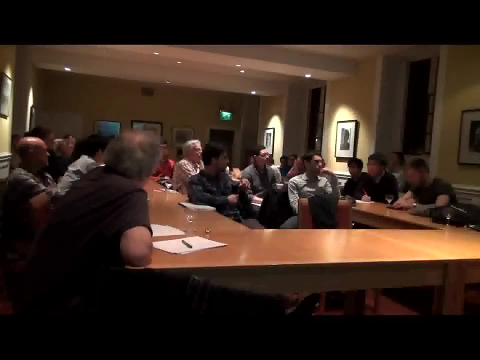 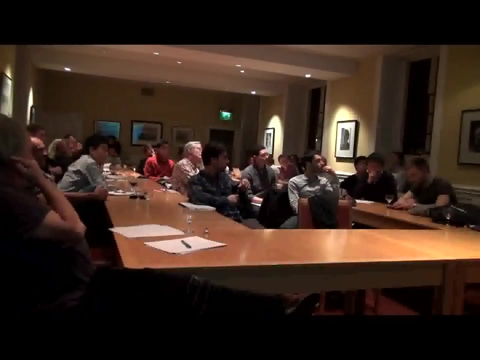 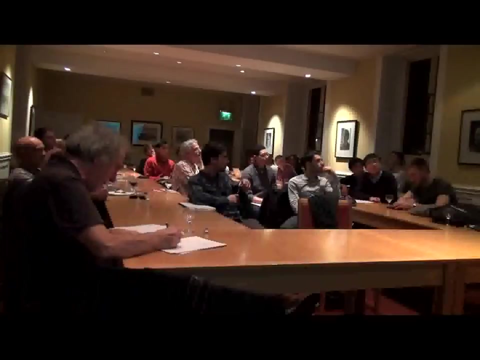 So- and that again is a surprise- It's a particular class of chaotic model. Again, that's one actually important point. I should emphasize that nonlinearity is not a case of inserting nonlinear behavior on a linear system. The nonlinearity that I built on, which is Goodwin's model, had a fundamental nonlinearity: that the wage bill is wages multiplied by labor. 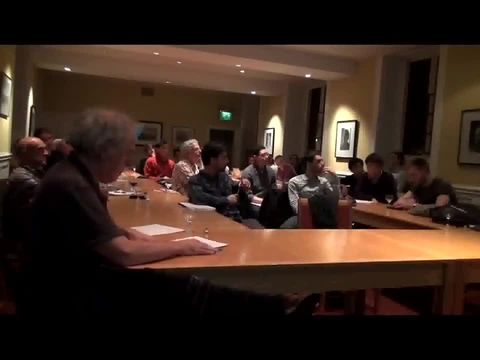 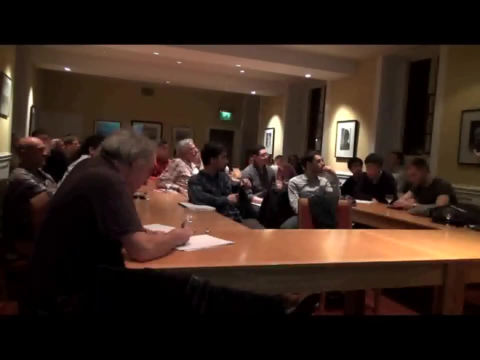 That's two variables multiplied together, semi-quadratic. That's what gives you the fundamental nonlinearity. So when you bring in nonlinear behavioral functions, they're simply saying: let's put realistic bounds on these things. Workers don't accept huge wage cuts when unemployment is gigantic. 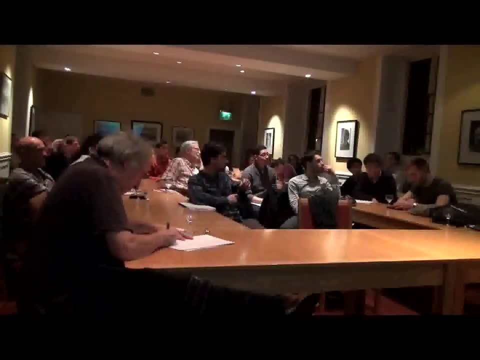 And capitalists don't smash up factories when the rate of profit is low. That's all you're doing. by having a nonlinear function. You're bringing some realism in, But the actual, true, the basic nonlinearity comes out of the interrelations of entities in the system itself. 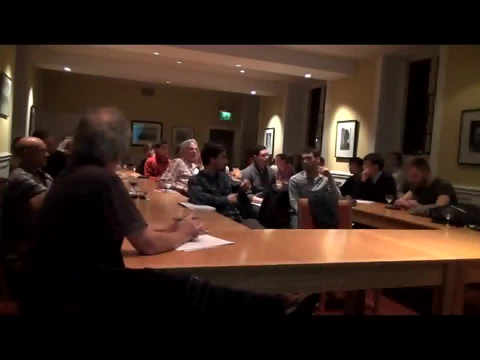 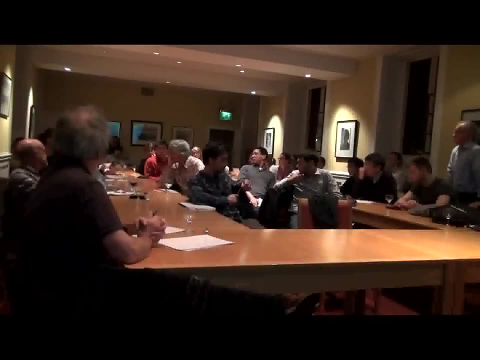 which again comes back to the points that Anderson was making. It seems at some point you are sort of making me confused between putting empirical content, sort of matching in the model in the sense of matching reality, and it being realistic. It seems to sort of use both as interchangeable. 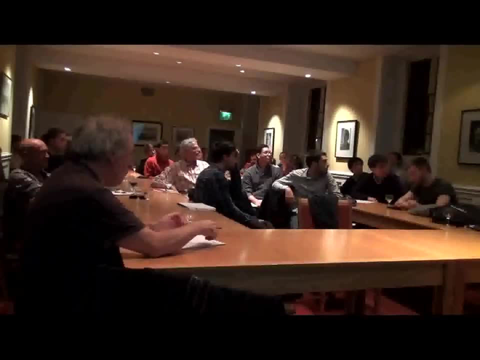 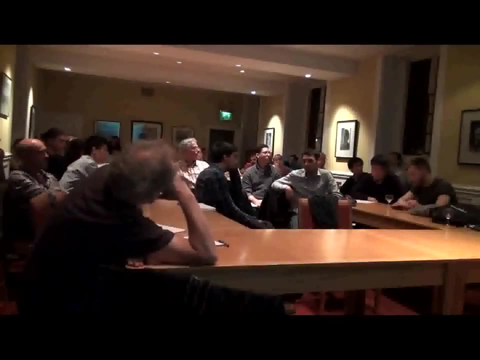 Well, maybe in a 40-minute presentation or one-hour presentation perhaps I'm trying to. when I do modeling, I'm trying to capture what I see in the real world. It means you're giving it an empirical- Yeah, there's got to be an empirical foundation to it. 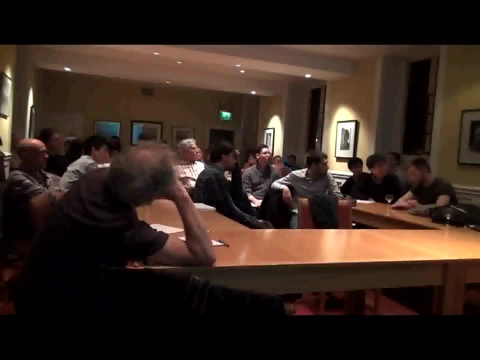 If we didn't have debt cycles, if we didn't have the Great Depression, Minsky wouldn't have come up with his model. If you look at Minsky's work, his initial inspiration was not Keynes, It was Fisher. Irving Fisher's paper was the first paper he quoted. 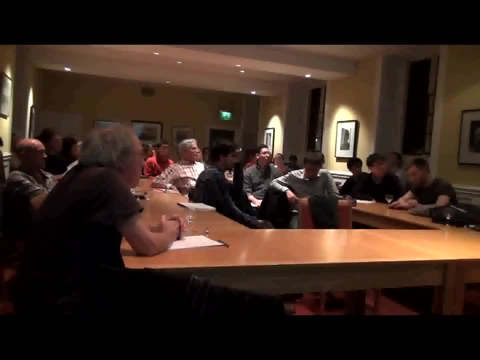 By the way, I can give one little secret: That wasn't the first real inspiration he had. The first inspiration was Das Kapital. But he could never publish that in America during the McCarthyist days without going to jail for it and certainly losing his job in the American University. 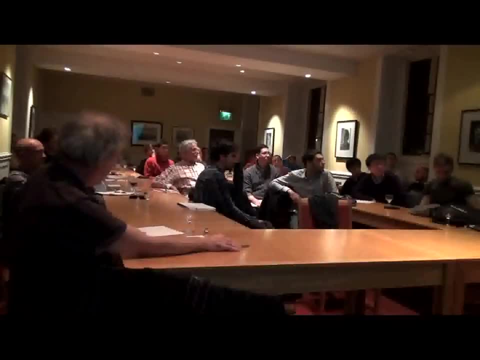 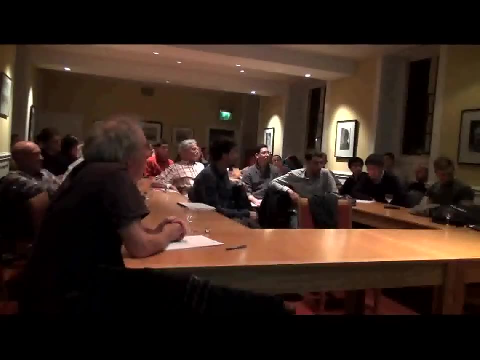 I know from his son that his first inspiration was Karl Marx. So he doesn't say that, but that's the inspiration. But certainly if the Great Depression hadn't occurred then he wouldn't have said: to model capitalism, you have to have a model that generates your Great Depression. 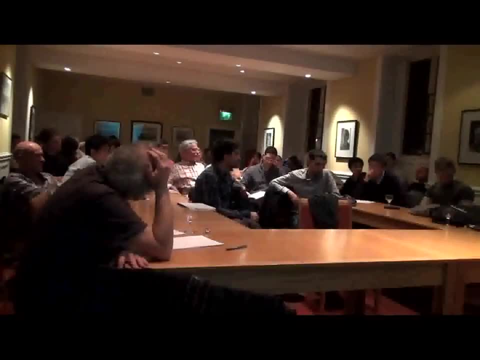 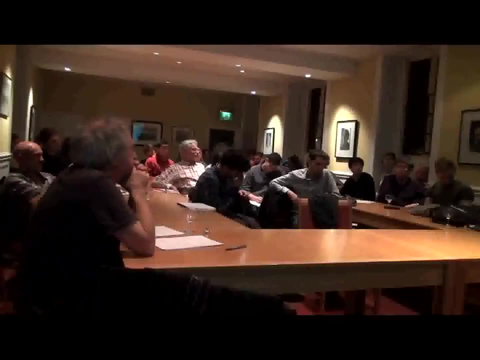 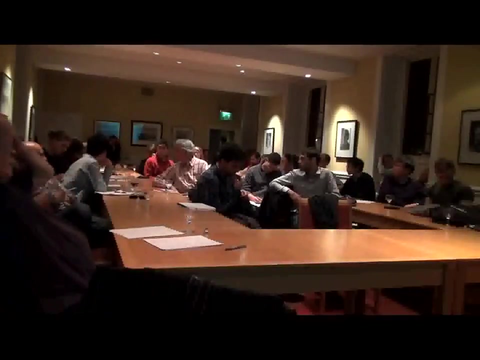 That's the true, deep insight in Minsky's work. We have to be able to explain the calamities in capitalism, and that's the last thing that I tried to do in that model which I wrote back in 1992.. Then it seems that you diverge from Tony. 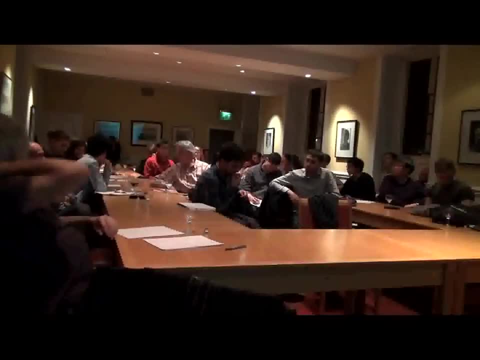 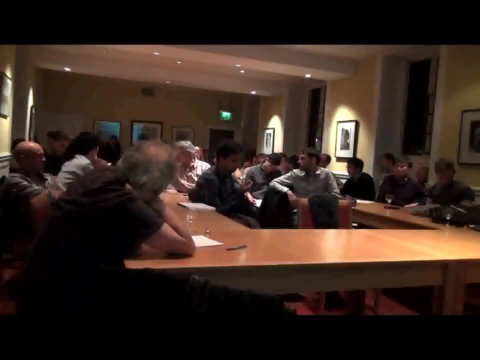 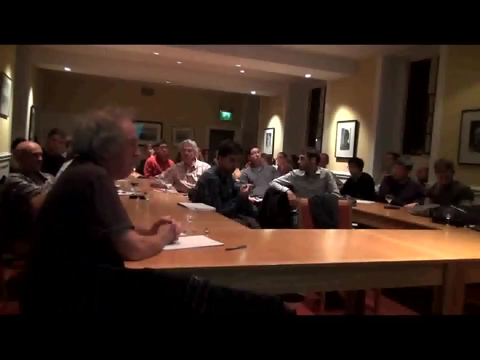 In a way, you use the term realism. You're trying to build up realistic models. I would say that, Tony, when he speaks of realism, it means he's giving it another meaning. Yours is giving an empirical context. Am I wrong on it, Tony? 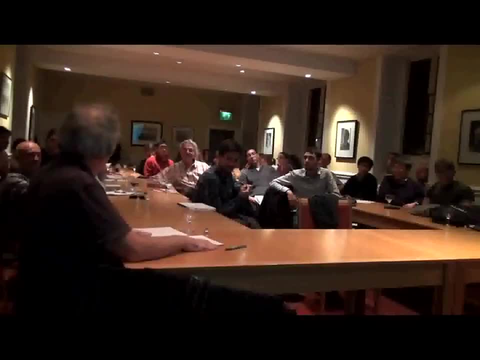 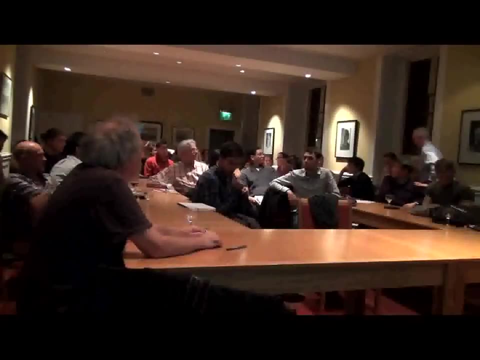 There's nothing wrong with empirical context, No, but you're going a bit beyond that, aren't you? Yes, I've seen a reason not to be realistic all the way down, Not just in a few assumptions, but we've lost the speaker. 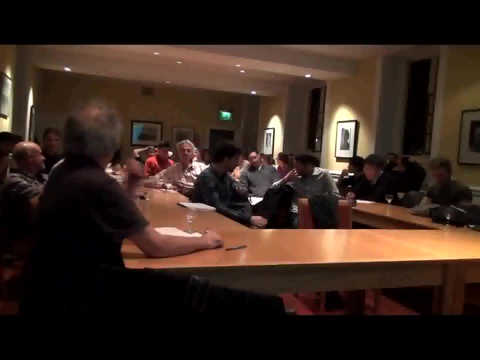 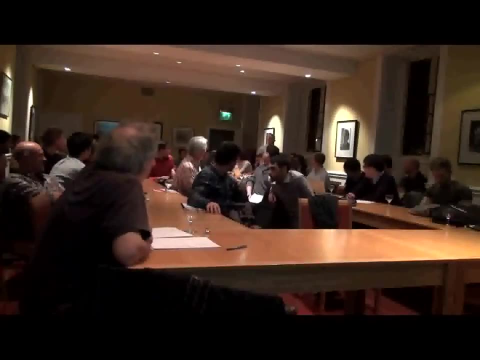 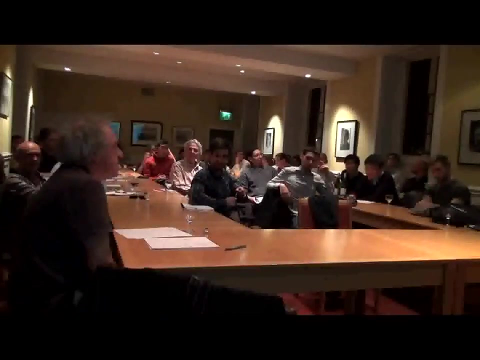 And I don't want to take over. Well, I'm happy to guess that Anybody thirsty to stand at the table. Steve, I noticed the room is quieter than normal And there could be lots of reasons for that. I'm wondering about you saying mathematics is a powerful rhetorical device. 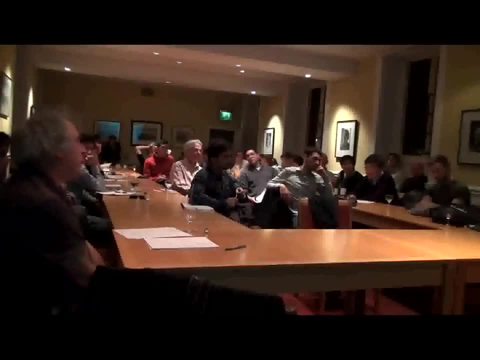 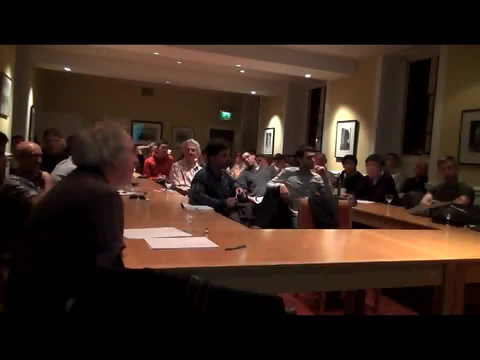 And I'm wondering what gives it its power. I mean, if you walked into a shop and disputed something with a person, would you rip out a mathematical model and try to persuade them? I mean, in what sense? in what context? how is it powerful? 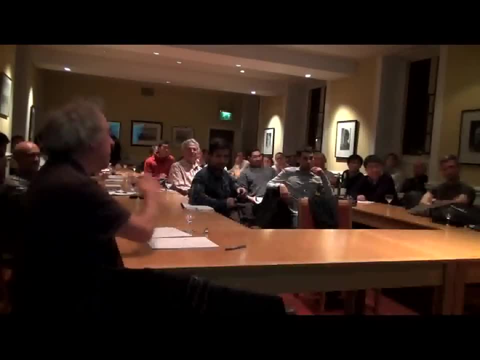 Does it shut people up? Does it tell people you're an expert, that they don't know what they're talking about? They have to really know their stuff to engage you. I think that neoclassicals use that to shut people up. 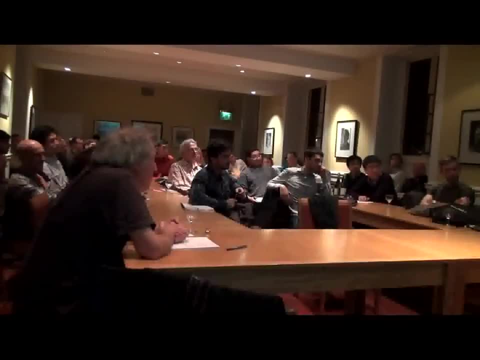 Which is one reason why I'm so glad that the physicists have got involved in economics. now It's called econophysics, Because it's a very brave and therefore, in the classic- yes, minister, sense of the word brave, A neoclassical economist tells a physicist he doesn't understand mathematics. 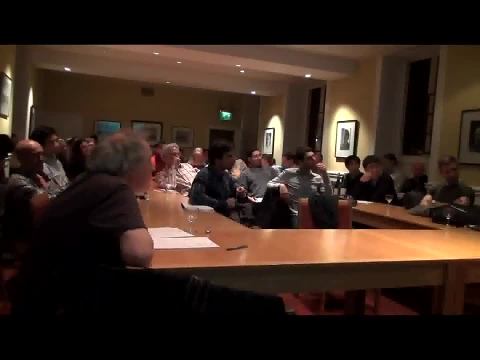 They run the news around economists, And they're getting involved now and saying this is horrifyingly bad. So in science in general, mathematics is a tool of analysis. It's you know. you're not going to convince somebody to go from Maxwellian physics. 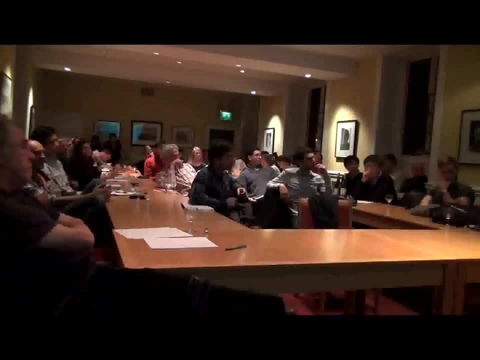 to quantum mechanics using verbal rhetoric. You've got to show a mathematical model that does it. Economics tried to borrow that. Math tried to steal that at the wrong time in the 1800s, Stole the wrong model and then ossified itself in that situation. 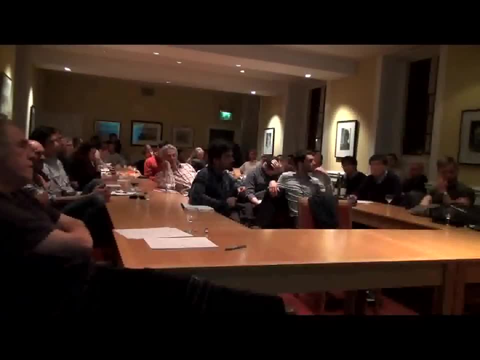 But it's still using mathematics as a form of rhetoric And if we consider our rhetoric versus their rhetoric, I think they're going to win all the time if our rhetoric doesn't include mathematics, Particularly when it comes down to models and simulations and things you can show a politician or a journalist. 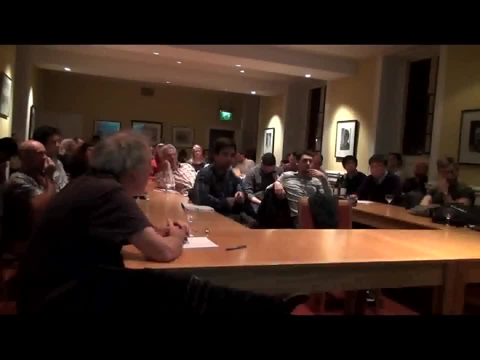 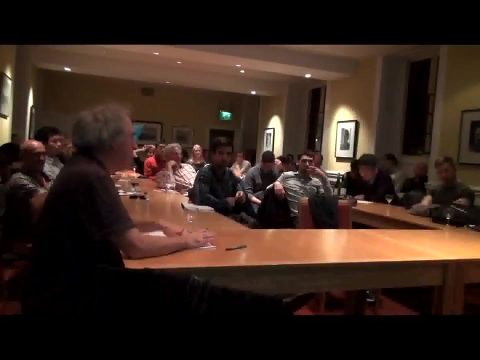 And that's because It wins the argument, Does it? I mean, by what criteria does it win the argument? They run the universities, we don't, So it's a power argument. It's a power argument. That's a good post-modernist conclusion, but it's not a realist sort of argument. 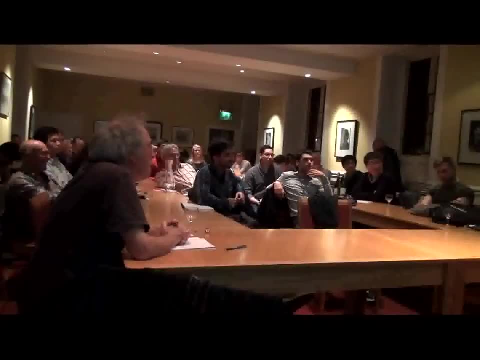 It's a realist one as well, because realistically, I want to take realistic economics, And if we see mathematics to the neoclassicals, it'll always be unrealistic mathematics that dominates economics. OK, now you're arguing for it being realistic. 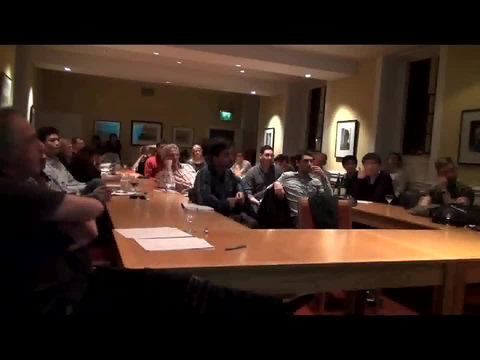 I always am. I wouldn't be bothering if it wasn't realistic Right By working in a surreal theatre instead, Or maybe living in Belgium, I would begin to wonder about Belgian-African conversation I had on Twitter over the weekend and stuff. 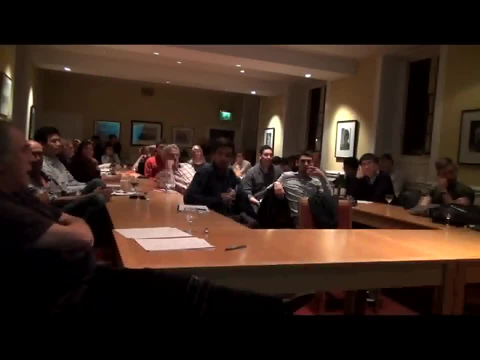 But if we explore dual models we would find a lack of realisticness or other things. Oh yeah, certainly. I mean, I've got a very simple investment response. I don't have any hysteresis built into how workers react to wage cuts. 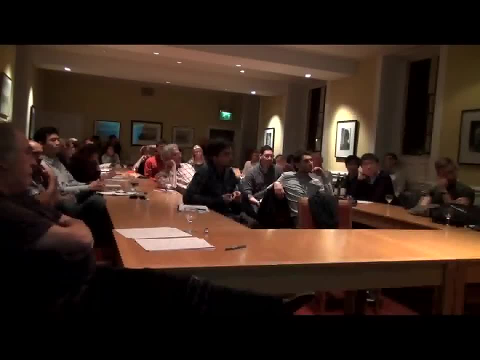 or how the government responds and so on. But with a complex systems model you can say, OK, let's now work on that particular component and bring in hysteresis and how the government responds to the level of unemployment and so on. You know that's how they used to justify their models: Scaffolding. 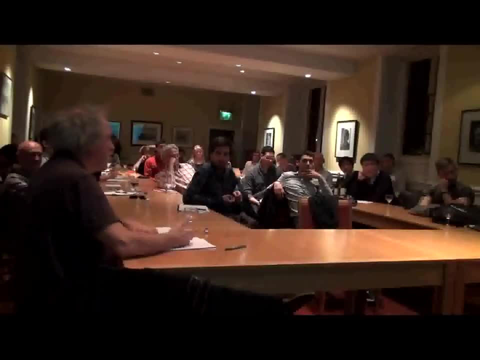 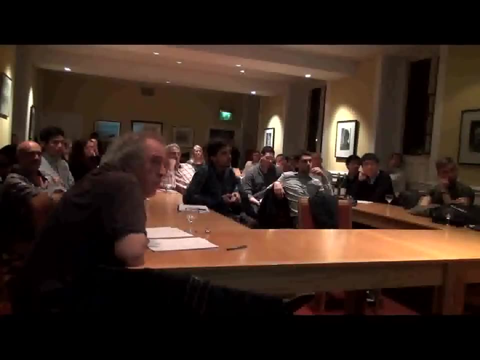 You know, OK, we've failed so far and we haven't got it fully realized yet, but we'll work on this and work on this. But I think I came a lot closer to reality with the model I showed you there than they've managed to do. 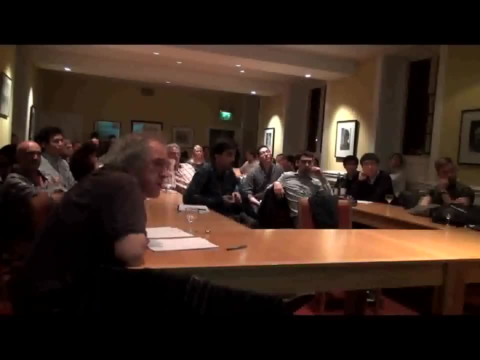 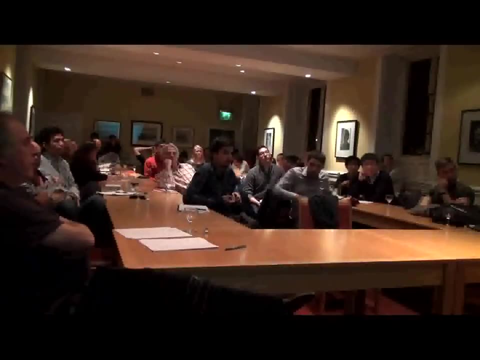 I'll just bring up my. But the reality you're getting at is you're accommodating something that you already know you want to accommodate. What do you mean? I mean you're starting from all ravens are black. No, I'm starting from capitalist: borrow money to finance investment. 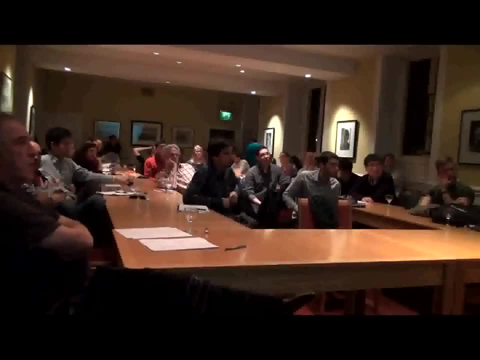 See, that's the element of realism that's left out of the model I worked with Originally. this is Richard Goodwin's model And I've corresponded with Richard a couple of times after writing his paper. There was a couple of other papers. 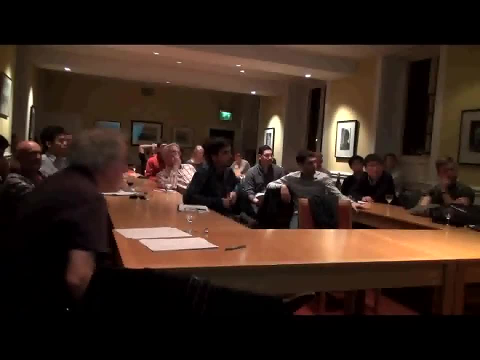 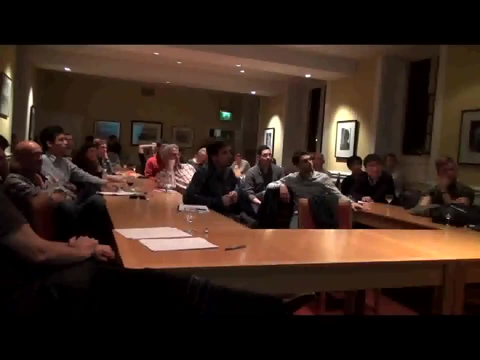 There was a couple of other papers And he tried to get me not to include debt and money in my modeling. He said he regarded debt and money as a waste of time and I shouldn't bother. OK, And I thought: well, unfortunately, realistically, I think. 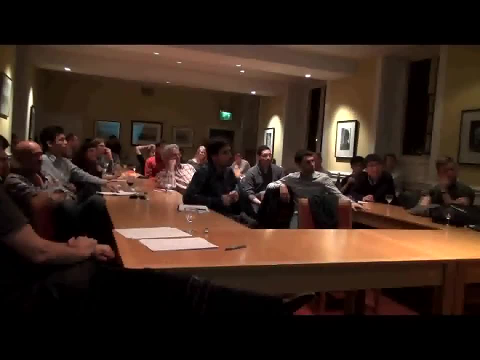 burns, borrow money to finance investment. That's a major part of the dynamics of the economy. So I took his model, which didn't have debt in it, and added debt and saw what happened. But I think, in a philosophical way, what I'm starting from is actually: 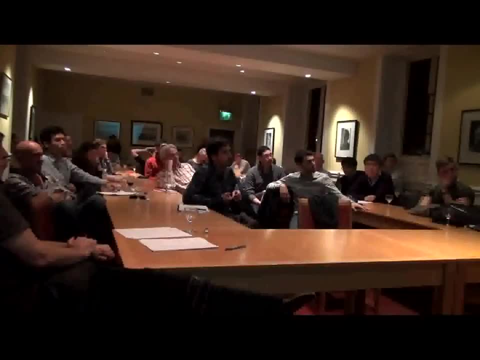 if I go back to Marx's original logic, I have a non-conventional interpretation of Marx as well, which rejects the labor theory of value. It starts from the idea that both capital and labor can produce a profit for capitalists, And you start from that perspective. 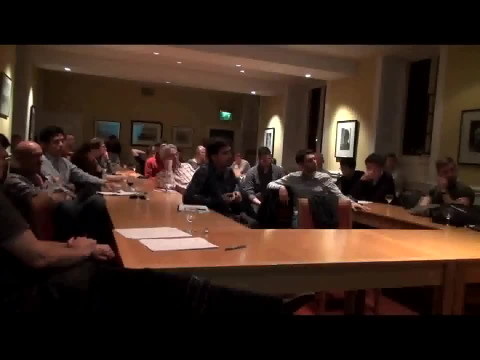 and the next level is that wages are a class struggle issue and tend to exceed the value of labor power as Marx defined it. He did that in cycles, which is what Goodwin was capturing in his 1967 paper. And then, when you go to Marx, past that, 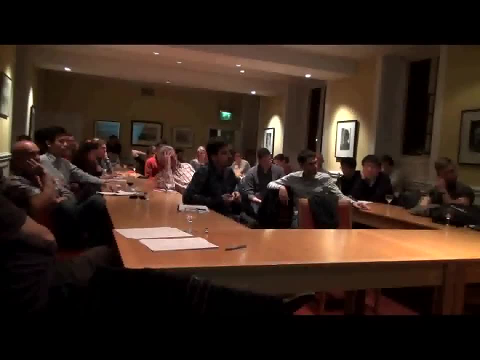 you find a role for money to have And then you have the idea of money turning up and debt finance and I've added that inside there. So I see myself as following that. That's my philosophical structure I'm building on. It's not being done in isolation or putting in bits and pieces here. 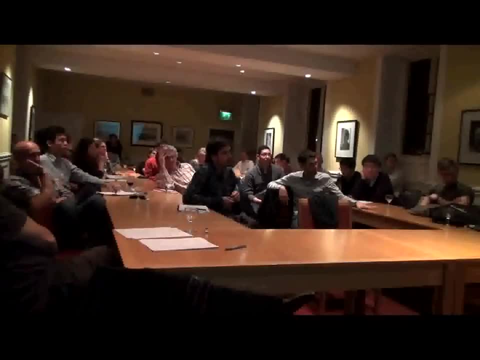 It's putting that overall vision together, but certainly not having completed it, And what I see is stuff I'm bringing in. I think would be minor perturbations rather than trying to explain a Great Depression, which doesn't happen in my model. 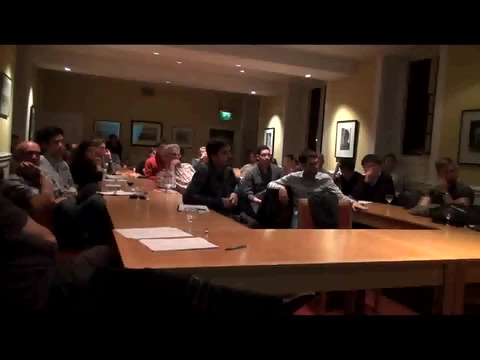 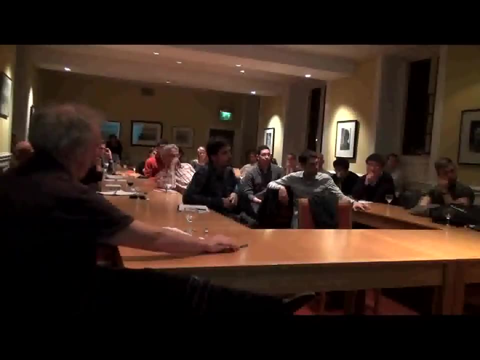 It does happen in my model. The neoclassicals are trying greater perturbation in the 20th century and 21st, So I think their stuff is an order of magnitude outside what I'm trying to do by adding I've come up with using the example of Ptolemy versus Copernicus. 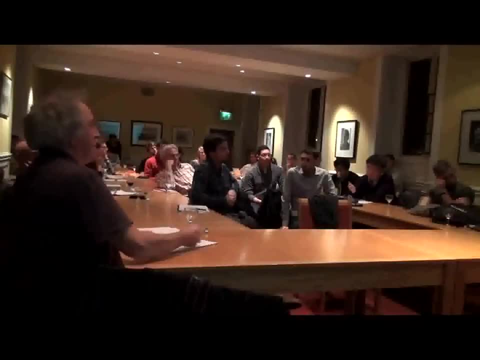 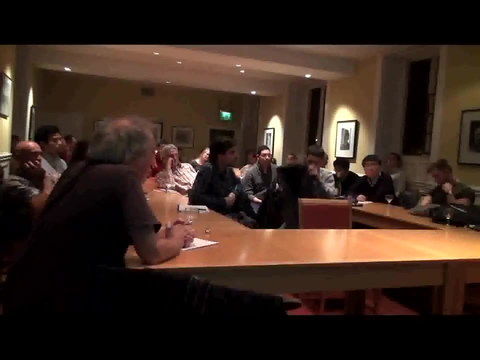 to try to really characterize the neoclassical world versus the rest. Not that I'm the first person to do that, I'm sure. But the neoclassical vision, Ptolemy's vision was: the Earth is the center of the universe. 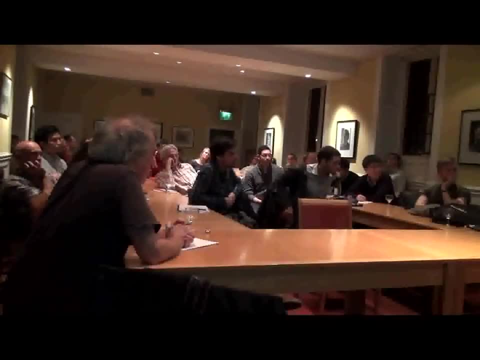 and the Sun and the Moon and the stars and the planets orbit the Earth and apparently, according to Aristotle, 55 crystalline spheres. And because that didn't explain the motion of the planets, Ptolemy added: epicycles, circles on circles. 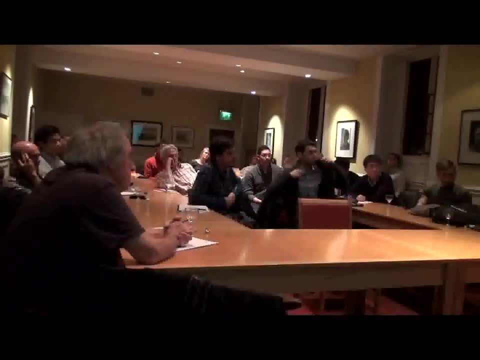 And then, with that model, circles on circles can match any motion in the heavens. It's an incredibly accurate way of describing the notion. It's a completely unrealistic model of the real world. Now then we come to Copernicus, who says the Sun's the center of the universe, as it was known then. 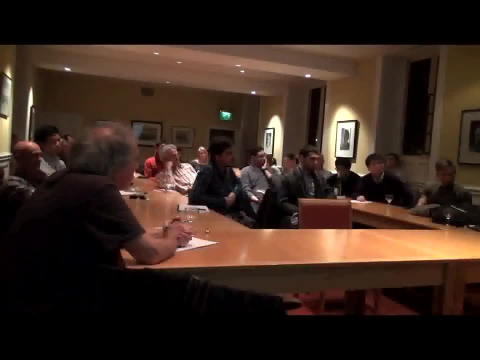 and the Earth and the planets circle, the Sun and the stars are a huge distance away, And that's the mental flip between the Ptolemy vision and the Copernicus vision. Same thing for what we're talking about. The neoclassical is an equilibrium: non-monetary systems. 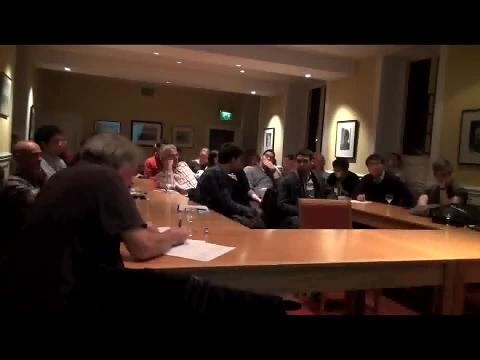 and individualistic perspectives. I'm saying we've got to go non-equilibrium monetary to model the economy and complex systems. So it's a huge shift in thinking and that's one reason they're so resistant to it. It really, for them it involves going from being Ptolemaic. 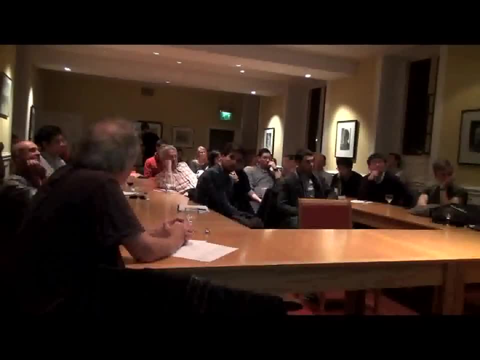 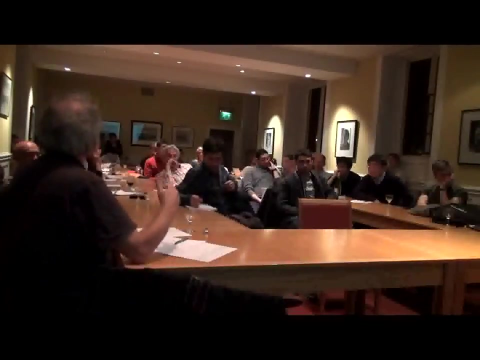 one of Ptolemy's Ptolemaeans- to Copernican astronomers, And they didn't do it, they simply died out. But astronomy also picked up those views far better than neoclassical economists have picked up the alternative. 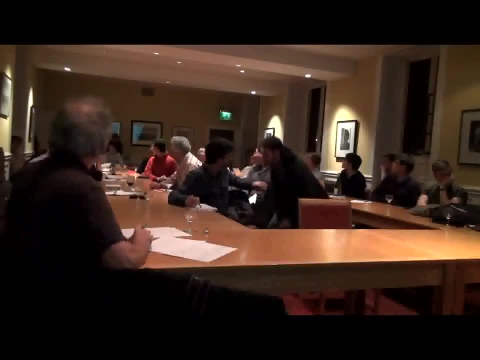 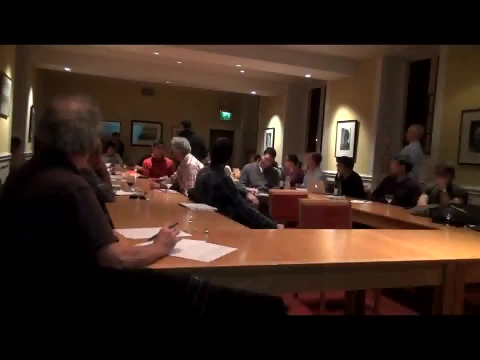 Is that Diane? Yeah, So you say that with epicycles you can find, you can just match whatever you want to match? Sorry, I don't have my hearing staff. Sorry, you're saying with epicycles they were included to match whatever they wanted to match. 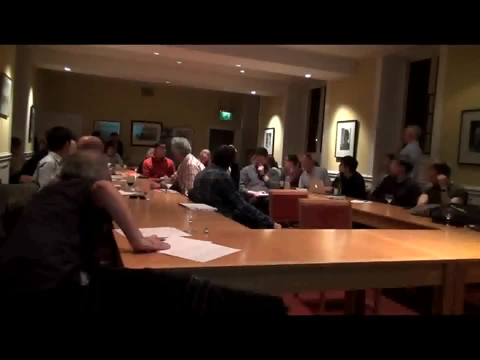 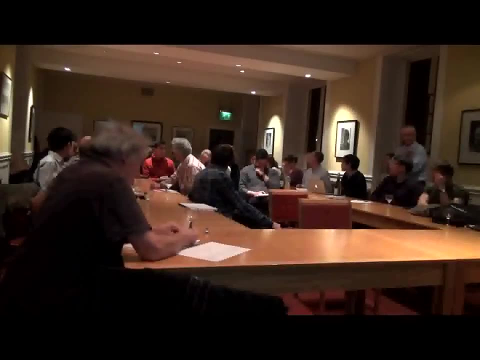 Yeah, But you can say the same about complex system simulation, because there are so many parameters and so many distributions you could be drawing from and so many complexity levels, such that you can also get them to match whatever you want to match. So how do you? I mean, 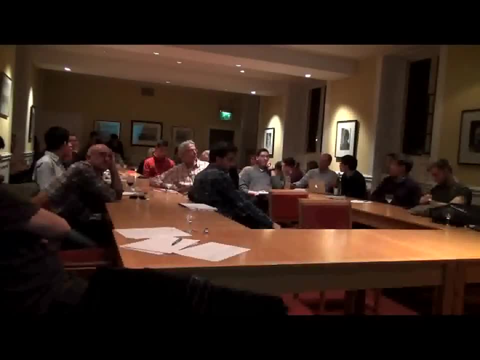 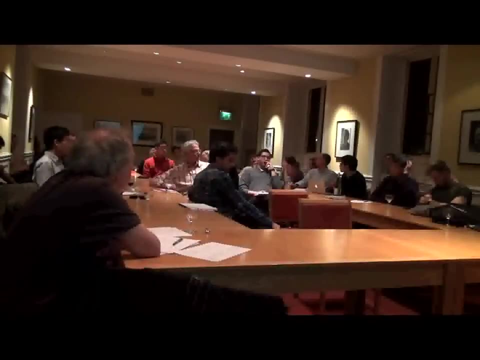 you may accept that criticism. Are we saying that? still, they're useful because they allow us to expand our imagination with respect to the possible outcomes of a given mechanism through all those possible ways. It's more than how you characterise them, because the complex system says it's the interaction. 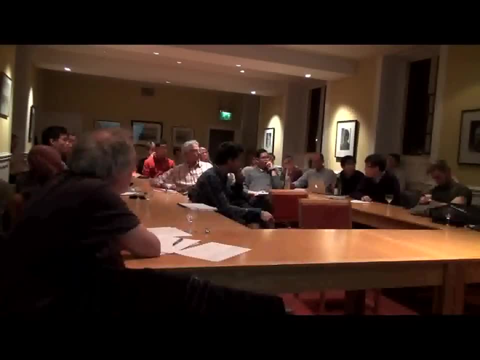 between entities that matters possibly even more than the entities themselves determining the system's behaviour. So if you simply argue that wages times labour, No, no, no, I agree that the complex systems approach is much more acceptable in terms of realism, of capturing more of the interrelatedness. 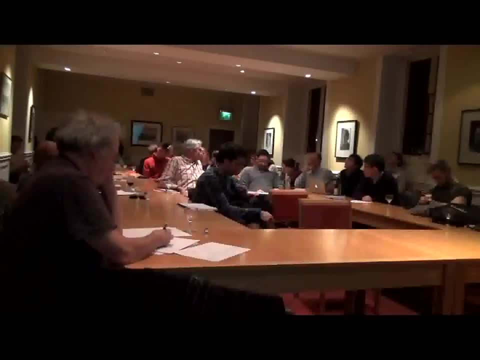 of all these human relationships that make the economy. But I'm just saying that in terms of the methodology for getting results or whatever, or input. I mean you can get these models to say whatever you want them to say. So how are they any better? 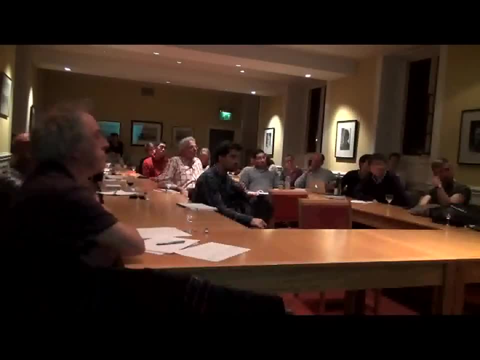 I think you have to look at more the fact that it's the structural nature of the models that determines the results. If I'm trying to find, No, I know, but No, I don't think you know. Pardon me, but I'm going to disagree there. 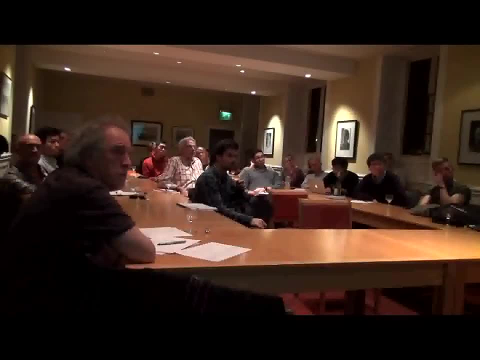 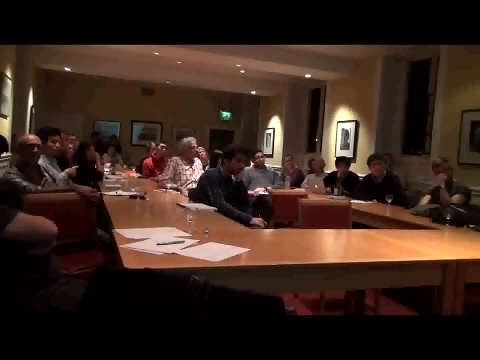 because the model I've shown you a moment ago is a non-linear model. I mean you can put whatever non-linear functions. No, I'm not. What I'm talking about is the overall character. This is a linear system. This is a model where I've got linear functions for everything. 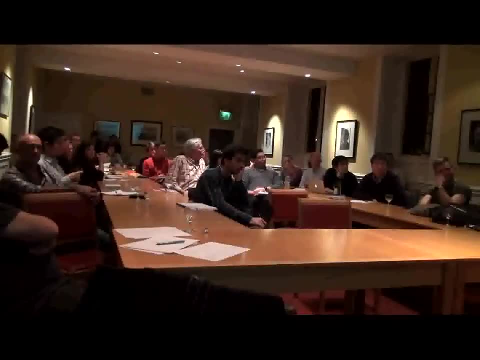 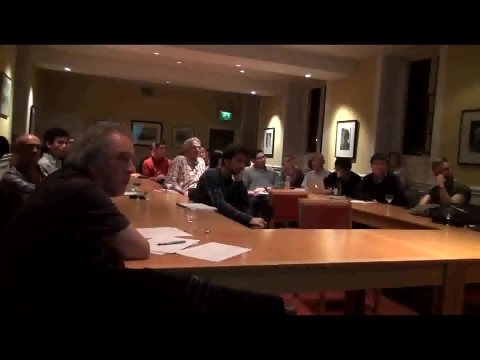 I know, I know What I'm saying. what's coming out of it is: the structure of the model determines the behaviour, more than the fitting of parameters to it. This behaviour of declining and then rising volatility is something which comes out of linear functions. OK, 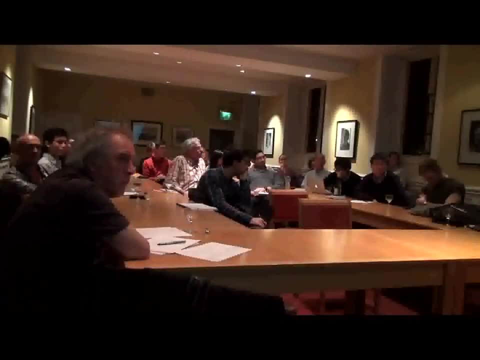 It's the structure of the model that generates that behaviour. So it's the essence, The essential. non-linearity is the important difference between this approach and the neoclassical approach, where, if you have linearity, you've got to wait in any cycles to get the results you want. 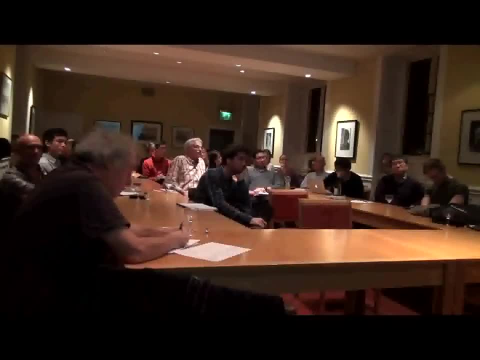 Here I'm getting the results that I didn't expect, but inverted commas I want, and now I'm going to make them more realistic. It's not a case of generating it by adding in the bits and pieces that are necessary. 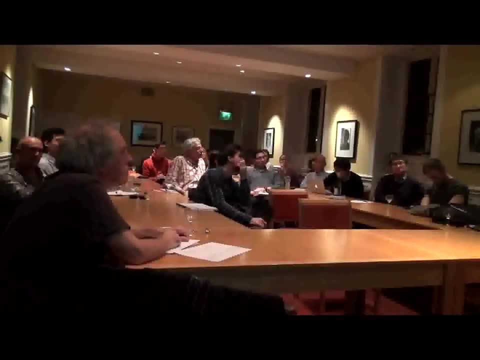 Like. I've been having conversations with some neoclassicals right now about their response to the financial crisis and they're saying: we're including banks now we've got financial frictions. It's friction That's the equivalent of epicycles in their world. OK, 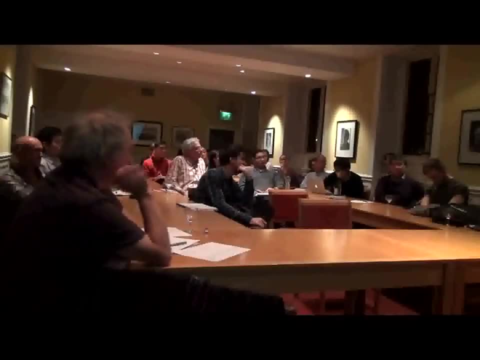 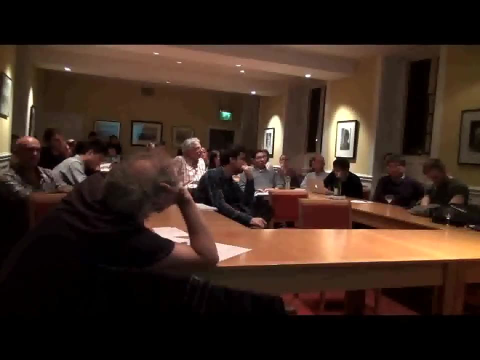 Now I'm saying it's, You've got to look at the structure, to bring the structure in With non-linearity in the structure. you have money as an essential part of your system. It's not just. You know, they are very, very different. 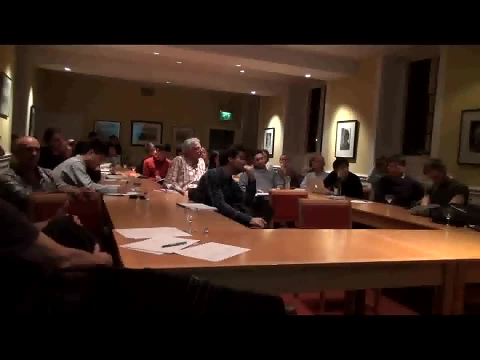 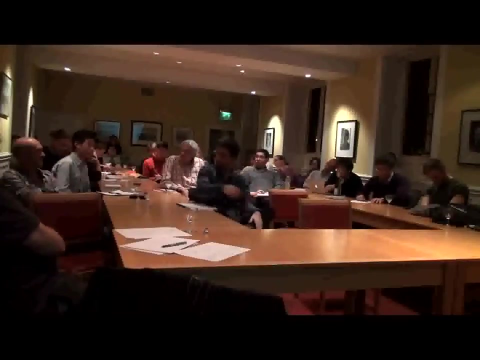 If I take you know. yes, OK, I'll change my functions a bit to get a better fit, but the characteristics come out of something. I haven't even tried to fit it to begin with. So to me, the use of mathematics, 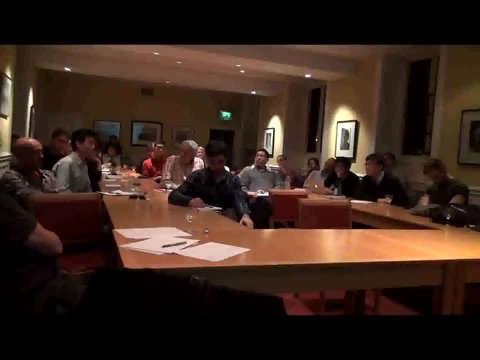 we make economics more like natural science in terms of, say, status. So will you see the models you make, as Is repeating a universal law, or do you see? Do you think it's better that it is describing? It's just an inspiration from the contest you're looking in. 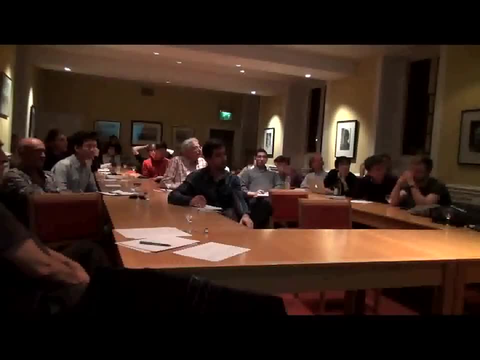 Yeah, That's a question worthy of a book. So, in terms of being more like the natural sciences, I'll say that the natural sciences try to explain and observe phenomena and evolve their understandings in that process, and we have to do the same thing. 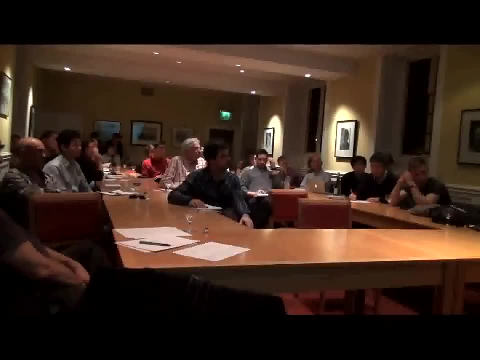 And I don't think economics has done that. It's tried to impose the vision of the world on its agenda and then tried to fit the real world to that vision, the reverse of what sciences would actually do. So I'm trying to emulate, in that sense, natural sciences. 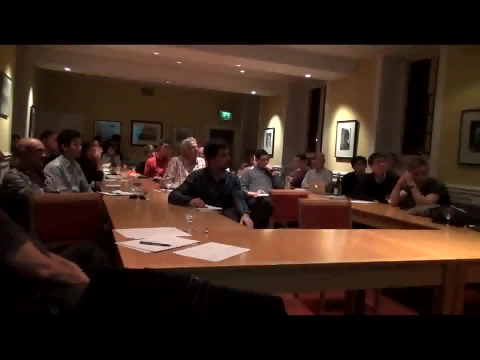 And I do want to ultimately, maybe in a couple of hundred years, have an economics that is non-ideological- It says neither left nor right is correct- is my objective. So in that sense you might see part of what I'm talking about. 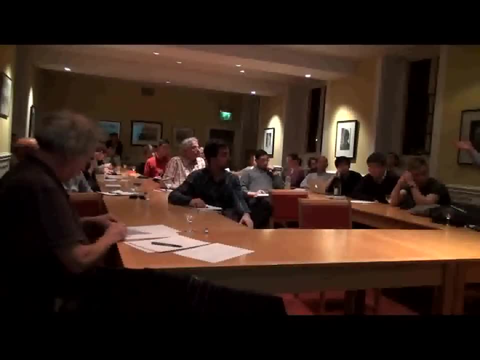 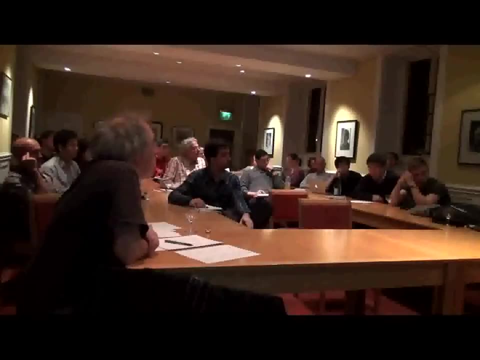 being a bit like Friedman's old positive versus normative, but without the bullshit, because his idea of positive was nonsensical. But we really have to try to describe the system accurately and this is what's the real objective of trying to bring in complex systems. 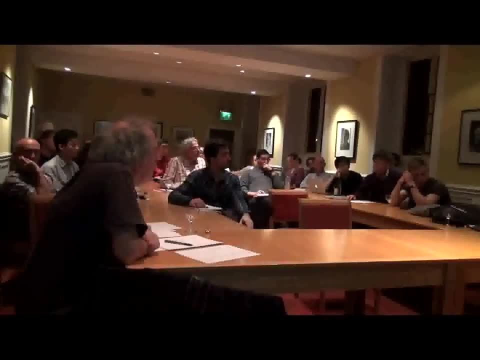 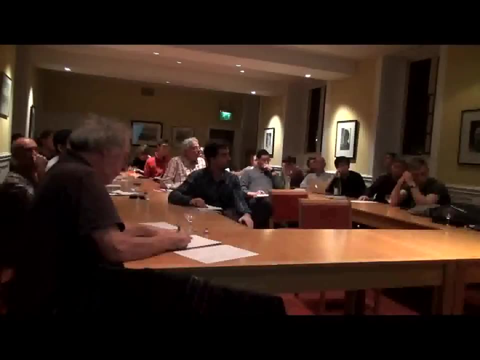 because the economy is possibly the ultimate problem. The complex system is more complex than the weather, So we have to take a complex system approach to understand it, and that's ultimately driven by the same realism that I think defines the natural sciences. Thank you. 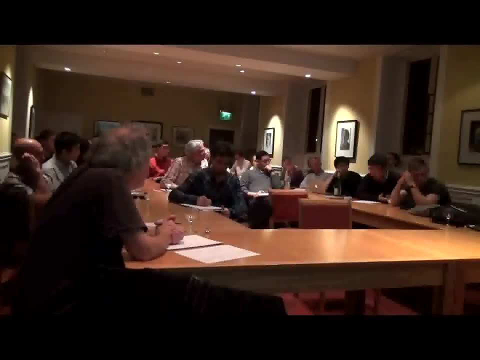 Yeah, No, I was. you know, despite being arguably one of the least mathematical economists in the world. I was almost completely agreeing with you until you said the last thing, which is that you want the economics, that you think the economics can be more ideological. 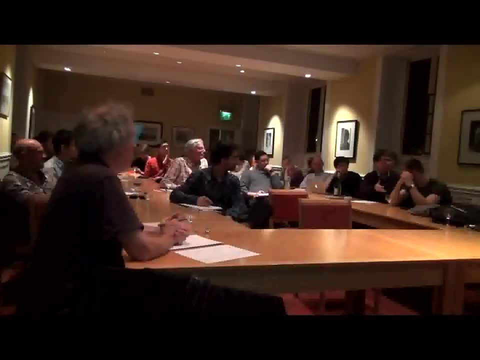 which I think is impossible. Well, I think. What is a commodity? What is a market? These are all politically determined. How can you say No? I mean, in that case I'm going to agree with you, But as much as we possibly. 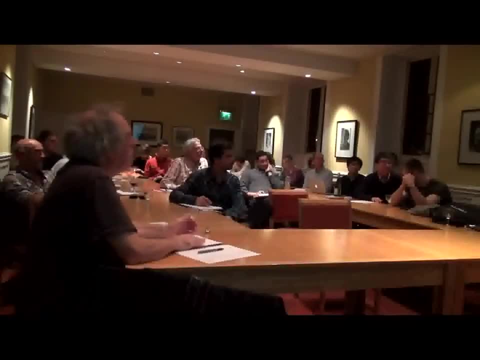 I mean defining labor as a commodity, for example, and that's one thing which, again from my position and interpretation of Marx, I see labor as both a commodity and a non-commodity, And that's again what I think. 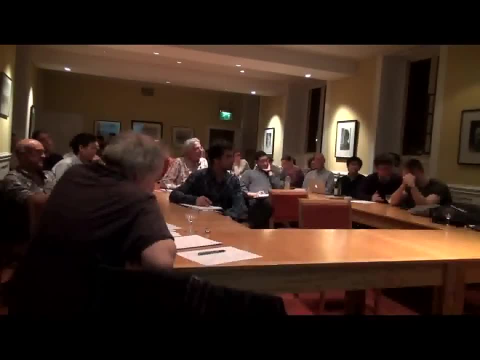 that informs how I think about building these sorts of models that you wouldn't. And Marx actually himself says this. It's quite fascinating If you look through his writings on economics. he talked about the wage and the minimum value of labor power and the wage on seven occasions in the same paragraph. 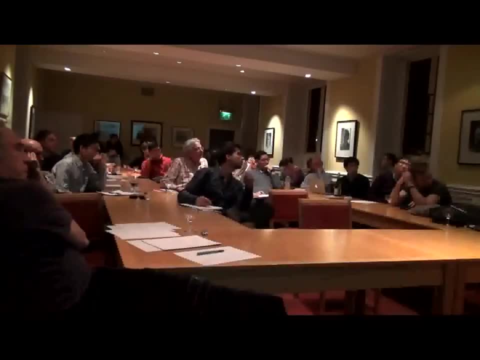 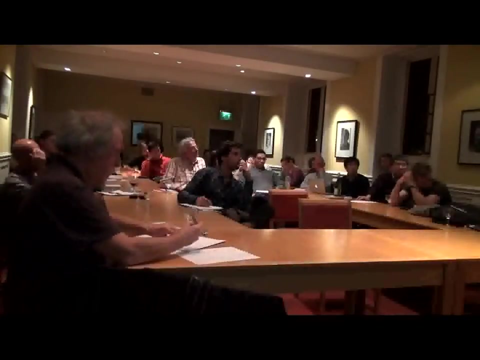 And each and every time he did, he said: the value of labor power is the minimum wage, not the actual, the minimum, which means he's seeing labor as both a commodity and a non-commodity. OK, So I take the point on that front. 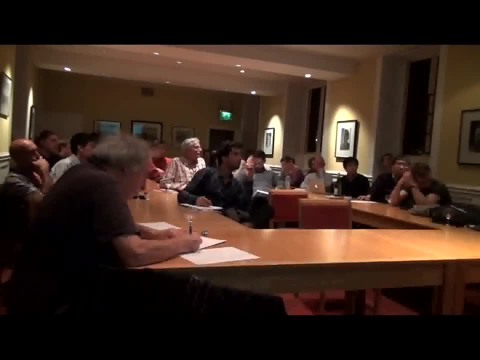 but that you will still have. politics is an essential part of economics, But to try to just build an understanding or description of capitalism that accurately produces what we actually see in capitalism, Well, the neoclassicals now I mean. I read a few actually relatively cordial fights with Tony Hicks. 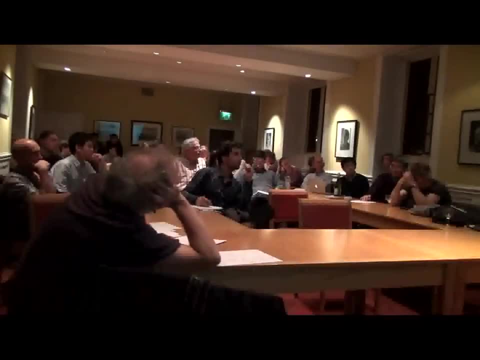 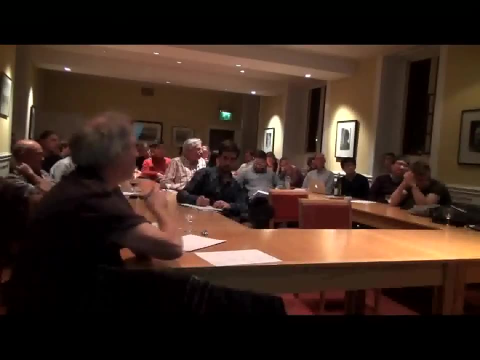 in recent moons on a I know cordial. You mean they're talking quite nicely to each other, which is a surprise, But he Yeah. but his view of non-neoclassical economics is that they are like pop talks. 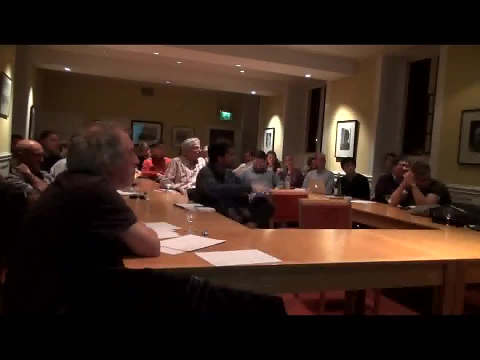 Yes, I know, I know, I know, But I think I might be. Maybe I'll change his mind. I'm not going to hold my breath, but maybe I will. But Oh, I've lost my bloody train of thought. 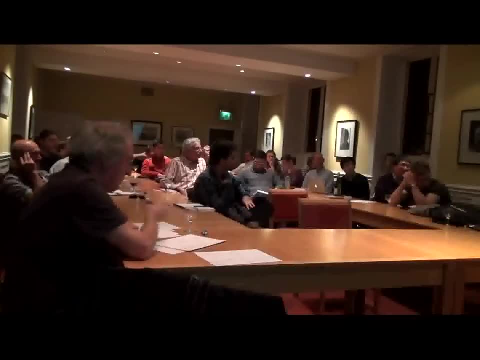 We've run out quite a bit of glasses. No, you're having a cordial debate with Tony Hicks. I've forgotten why. Oh right, OK, But Yeah, I forgot, I've lost them one. You run ideology at some stage. 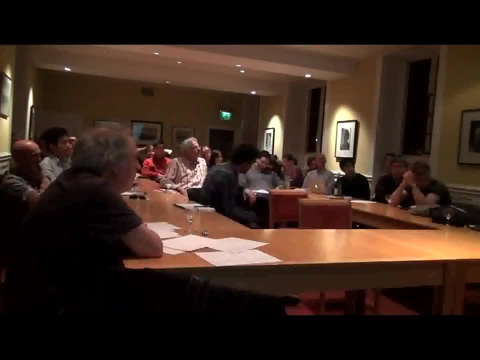 Yeah, ideology, And it's Thank you. Thanks for He's readily defending most of the time neoclassical models and rejecting anything else, but he actually admitted in a recent paper that the state-of-the-art and neoclassical DSG modelling 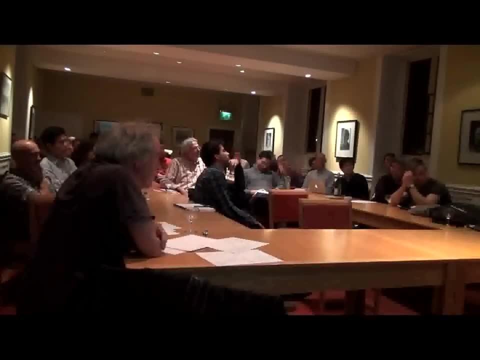 still cannot reproduce the financial crisis. OK, OK, Now that ain't a particularly good state-of-the-art, And you know that's what we need to reproduce in our models and that's the realism, and therefore the apolitical side, that I want to reach. 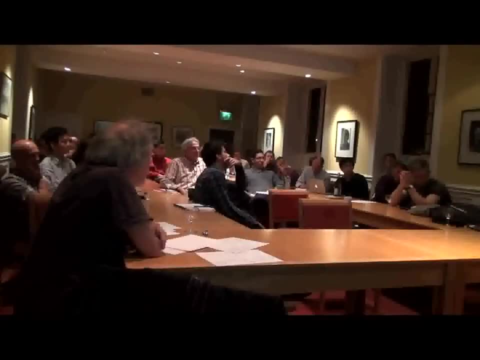 to say we have to have models that generate the sort of behaviour we see in capitalism before we can say we even have models that manipulate capitalism. That's the political. But you can reproduce anything if you don't stick to constraint of being realistic. 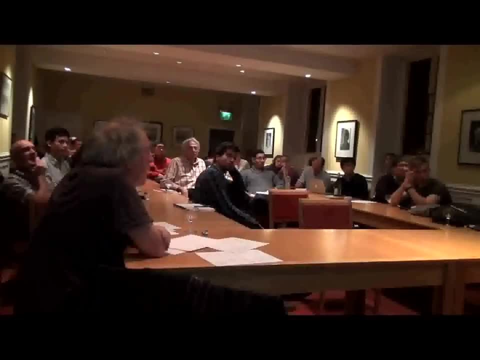 Well, they've failed to do that. Well, right, I mean, They can't reproduce a depression without being unreal. Their models are unrealistic and can't reproduce a depression. See, I guess I'm not so sure who the they are. 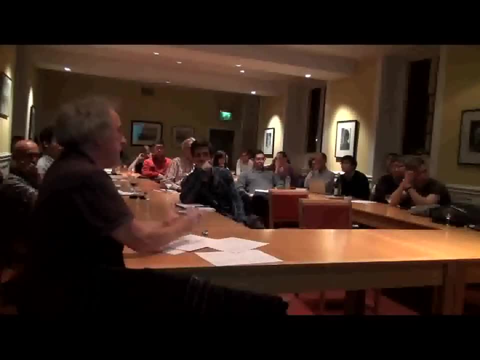 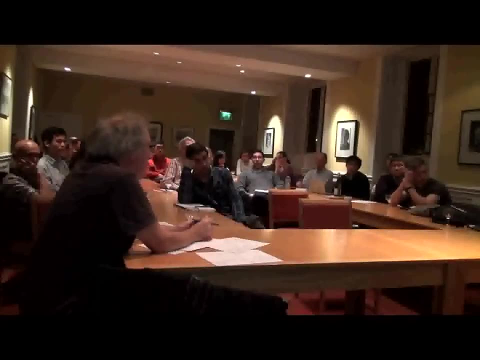 I mean you've got a conception of neoclassical, as if it's one version, one set of models or one model you've got. I mean, my experience of living amongst modelers is they can produce anything you want and the opposite of the same. 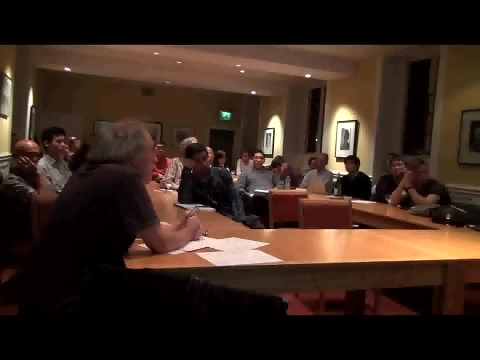 Well, in those days it was the same data set. Yeah, I, Neoclassicals, have a very particular approach. Still, logically, If you allow starting points, assumptions that are not realistic, you can generate everything like I did with brains. 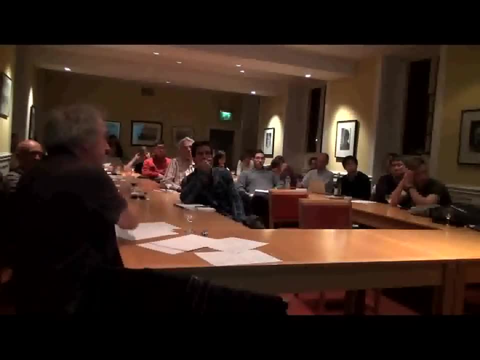 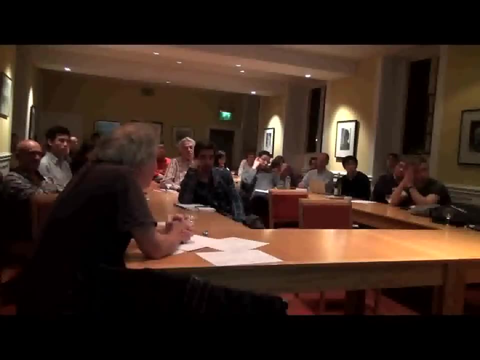 I mean, I could ask you to give me a proposition. I could generate it from unrealistic. Well, yeah, if you have unrealistic stuff you could use. you know Right. So accommodating the crisis per se after the event isn't. 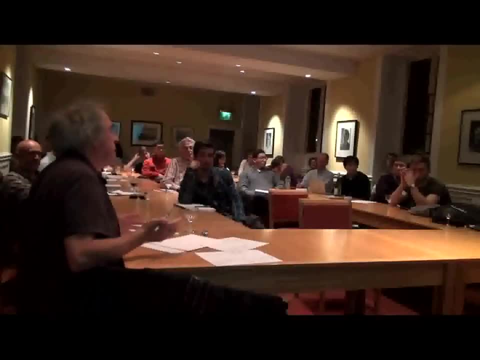 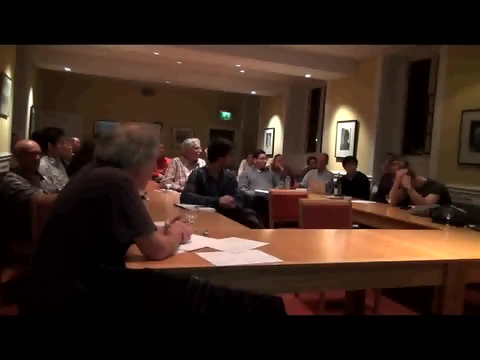 Accommodating the crisis after the event isn't such a fantastic claim, or Oh no, no, With realistic assumptions, isn't that his point? Well, that's the point. I've captured it at realistic, Very simple, realistic assumptions, captured in the process, before it happened. 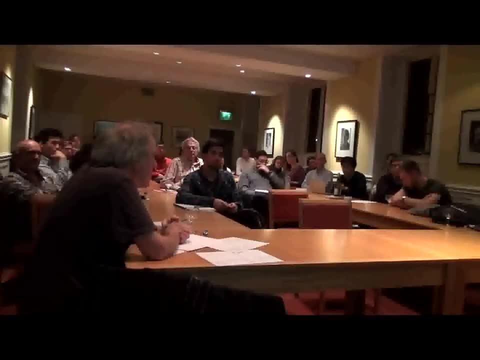 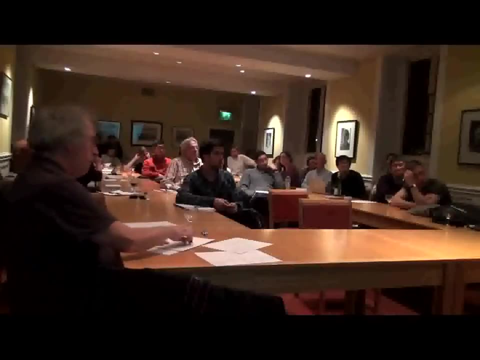 Yeah, I know I mean you've got simple assumptions and they're not all realistic. Simple assumptions which are realistic enough, and the simple assumption is that firms borrow money to finance investment. Yeah, That's the only simple assumption I added to Goodman's model. 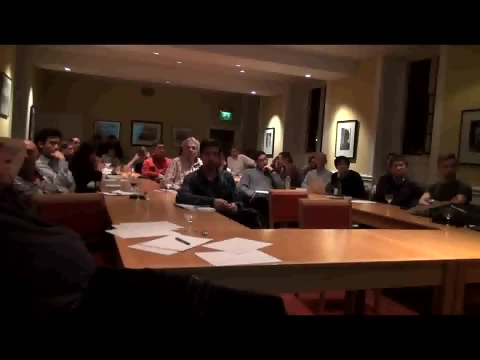 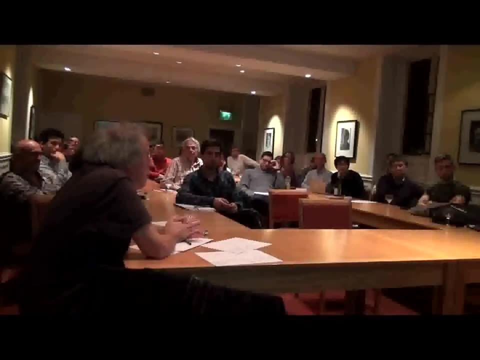 that workers demand wage rises, Yeah, but Goodman's model was Goodman's model, I mean. my problem is the assumption built in of atomism and closure, which is Closure but not atomism. Atomism I define as being reductionism. 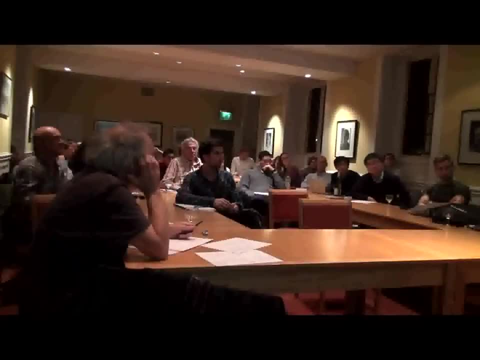 and able to produce things, Oh OK, atomistic and add up. It's not that sort of model, All right, But atomism in the sense of Keynes, under conditions X, I think that's the. I think it's different to Keynes'. 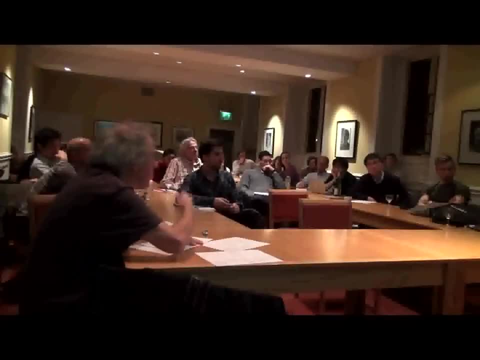 as a fiction of atomism. Well, I think the end is: Let's not turn a page before my conception of atomism Under condition X. you do want it, Organism, I mean. I don't think human beings are like that. 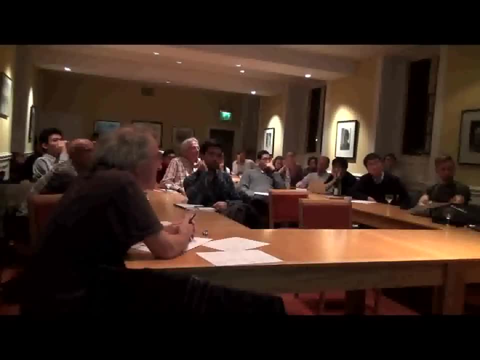 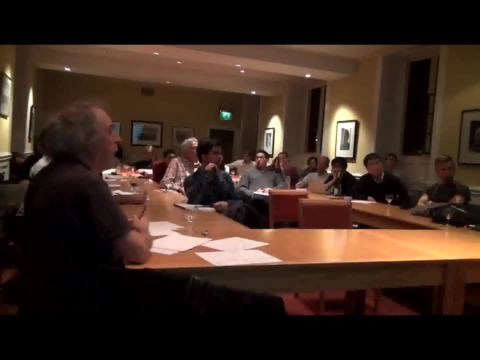 We just do not. Yeah, but if that's the case, why even do economics? I mean, if we can't find regularities, then why are we bothering doing? Why don't we do philosophy or yoga? I can answer that, but do you want to? 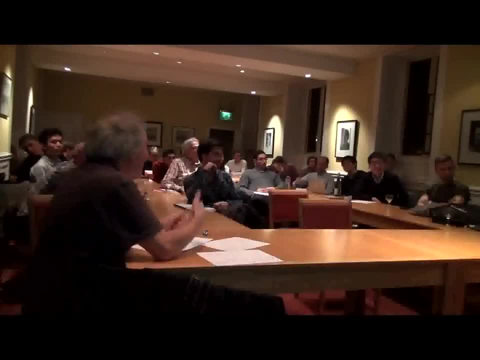 I said it all night. Well, I mean, yeah, I think there's Well to make the world a better place, But how can we make a better world? We can identify explanatory causes and get rid of bad ones, But that again involves modeling. 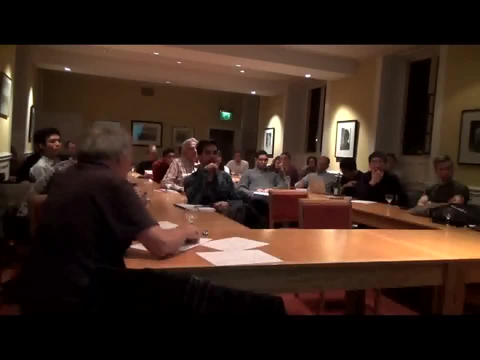 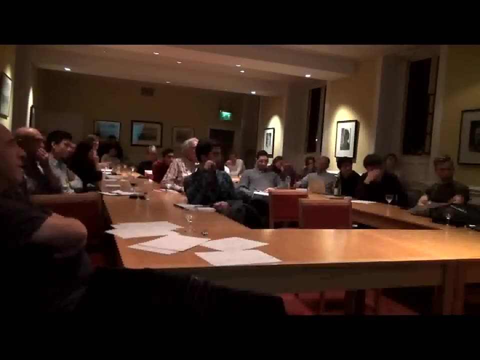 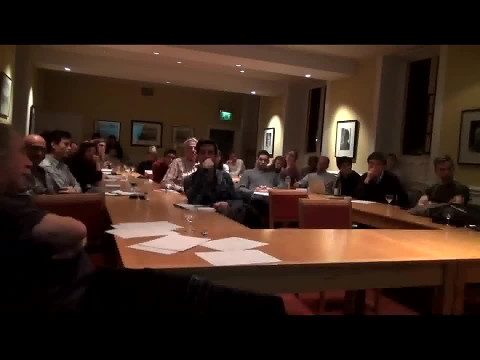 It's just that the verbal, That's your starting point. You said: if we can't do correlations, we can't do economics. You said: if we can't do correlations, is that right? No, not all correlations Or better regularities. 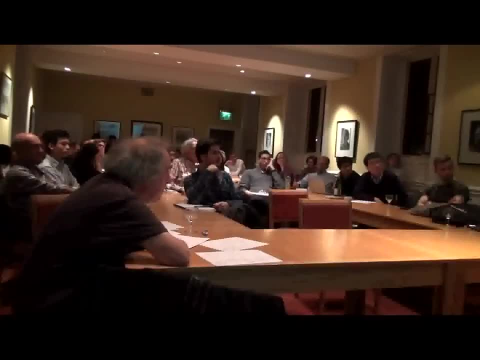 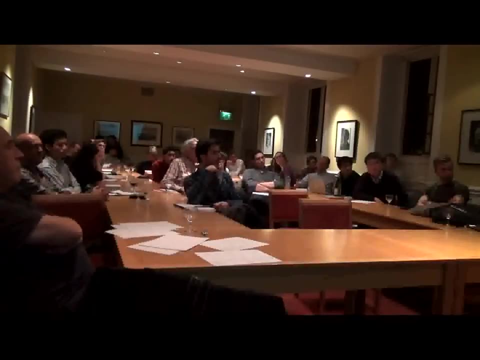 It's saying: when Marx and Keynes and Smith and Ricardo and everybody else put their propositions forward, they were putting forward verbal models, saying, given this rate of change, this will happen. And obviously they're saying: let's put them in mathematical form and see what actually emanates from that. 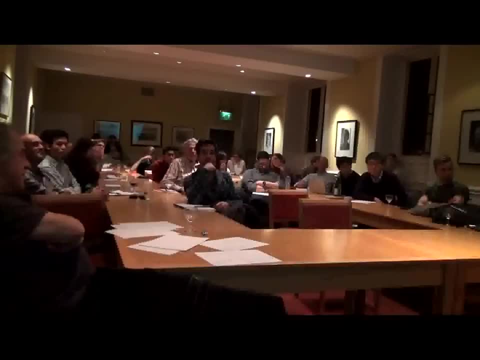 Well, they did say there's a tendency for such and such. Yeah, that's right. You can't believe in tendencies. You put a tendency in and see what happens. I saw a wonderful instance. I've forgotten the author's name. 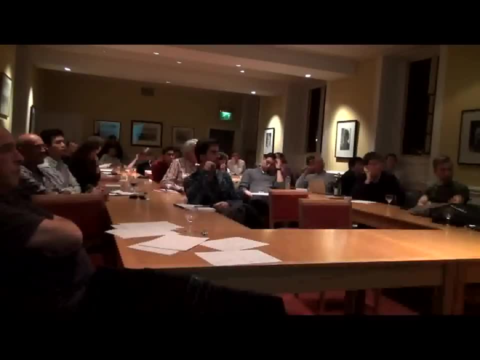 He's an English economist who specializes in religious economics as well as dynamics, And he made this proposition about Ricardo and Smith and Marx and Malthus talking in terms of verbal differential equations. So let's take the equations that Malthus had about. 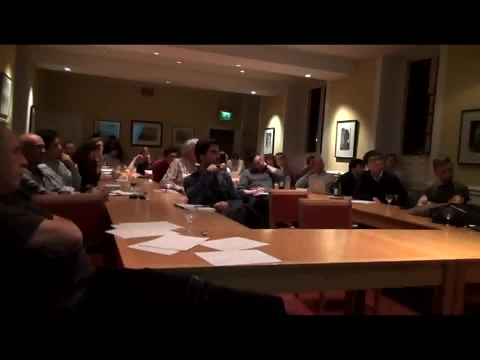 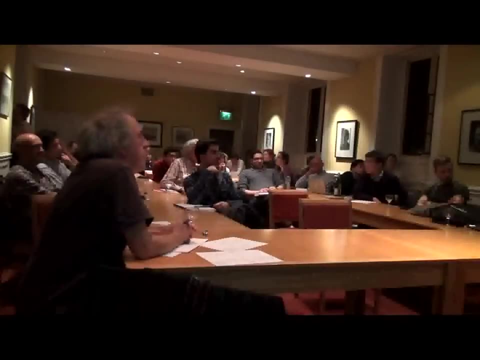 for example the iron law of wages. put that in mathematical form and see what the outcome was. And in fact that particular paper was quite intriguing. The results weren't what Malthus expected, And so we are thinking in terms of a model. 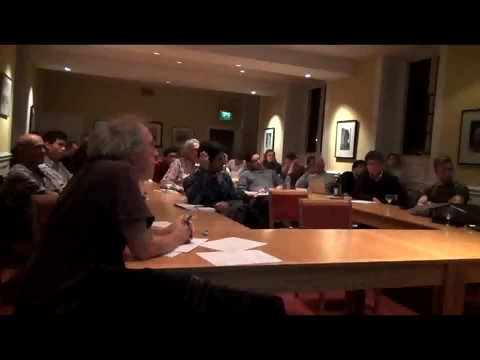 I'm just saying. mathematical models can give us further insight into our verbal models And they can actually sometimes tell us things we don't expect, like what I saw out of this model, and be contradictors. You and I are arguing over whether the certain claims of atomism 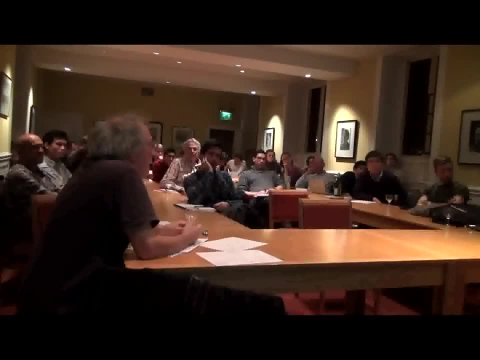 which we may not hold in common, are realistic or useful or whatever. Whatever we're debating, because I might not think on it- Do you think we can resolve what we're debating using the mathematical models? Not Good question. You'd need to be satisfied enough. 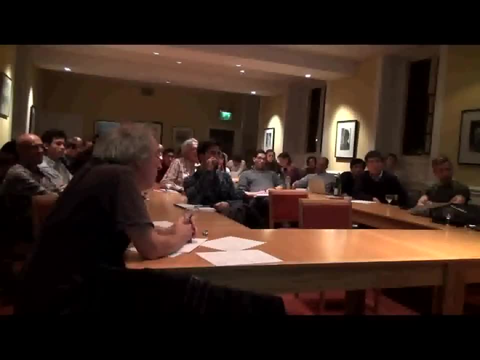 in the models, capturing enough of the real world to be able to make the improvements you were talking about a moment ago and then go to a better place. But you said to yourself: the slightest point, move it away. a little difference can send you off in a different direction. 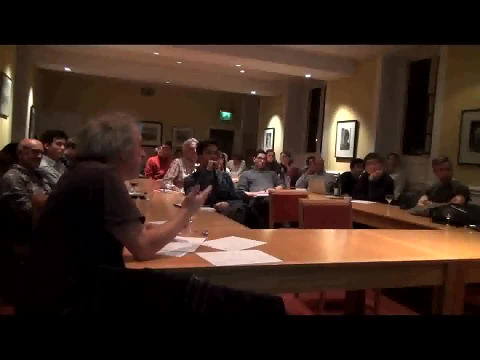 But that again comes down to this particular But I'm saying: you have this question of realistic enough and yet you allow that slight deviations from a starting point can send you off. So what about slight deviations in being realistic? Well, slight deviations. 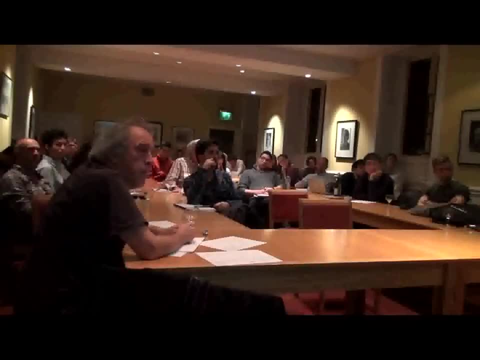 The particular model I built. there is one where there is no government sector, for example. What Minsky also talked about was saying the government plays a role of stabilising an unstable economy by working in the opposite direction. And when you feed a government into this model, 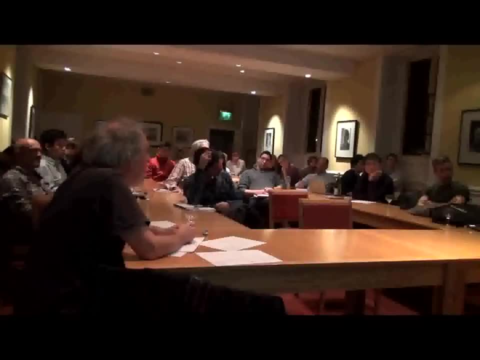 which is resolute, which actually defends a certain level of unemployment rather than accepting high and higher rates as it rises. you get a model which is cyclical but doesn't break down, and handles a wide range of parameters and actually is cyclically stable. 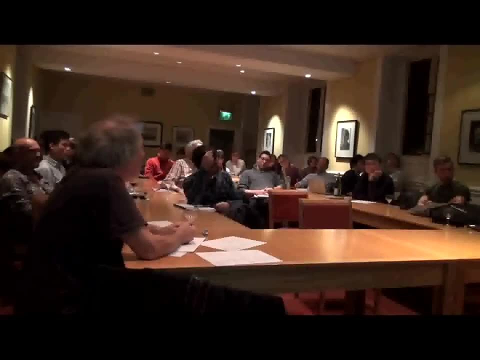 So what you then come down to saying is: what qualitative characteristics does our economy have to avoid a total collapse? And that's making qualitative statements about whether you should or shouldn't have government spending, for example, whether you should or shouldn't run a deficit. 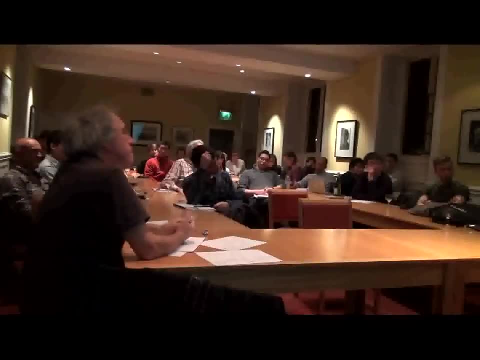 And, of course, the neoclassicals have got us believing you should have governments running surfaces. Look at the damage that has done locally. So it's that qualitative decision-making about the nature of a complex system that I want to make, rather than worrying about these tiny bits of prediction. 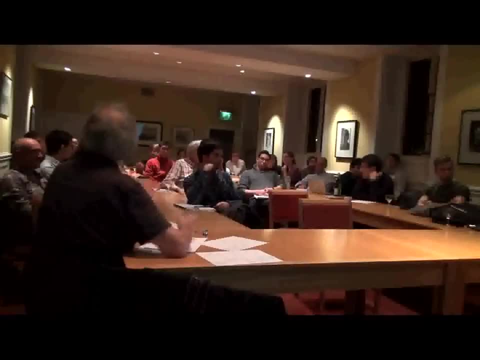 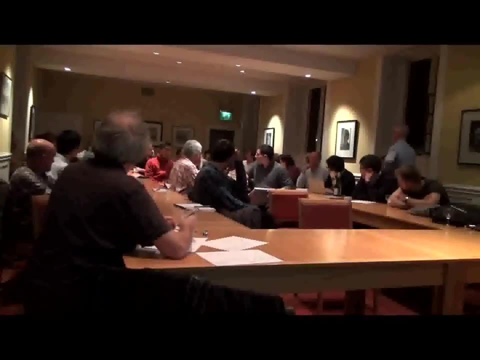 OK, Well, so much for time. Alison, Yeah, actually I thought I had a bit more to say about this than I was going to say already, but it's very striking that when economics became its kind of methodological individualist beast that it is, 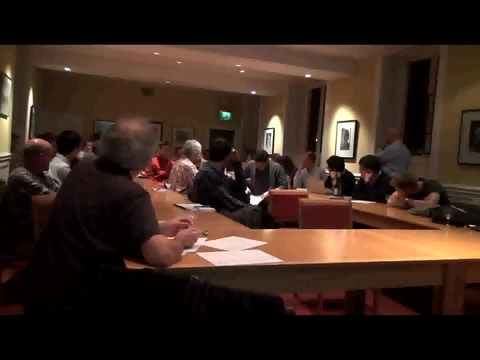 that was because it tried to copy physics right. It was the marginal revolution trying to make individuals into atoms and energy. you know, money into energy, sorry, capital into energy flows, et cetera. So it's very striking that it's now trying to get out of that mess. 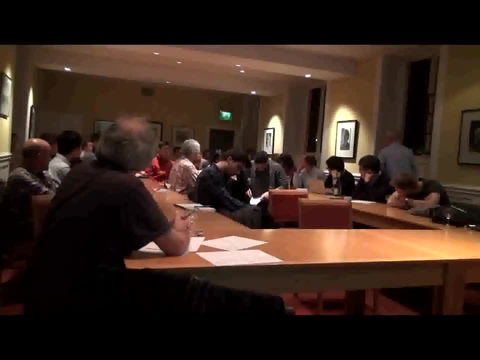 by again copying physics in a more complex system kind of parameter like your paradigm, albeit trying to catch up with physics in a sense. Are you happy to bear with whatever the consequences of that are in the sense of, Are you happy to throw out the question of? 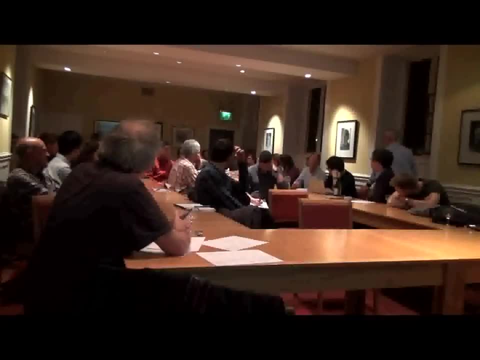 what kind of principle we want the world to be? Or is this just a two-step thing of you know, have the models get some answers and then ask the questions afterwards? Or are you happy that if the models came up with certain conclusions, that you'd be happy to throw out the political question? 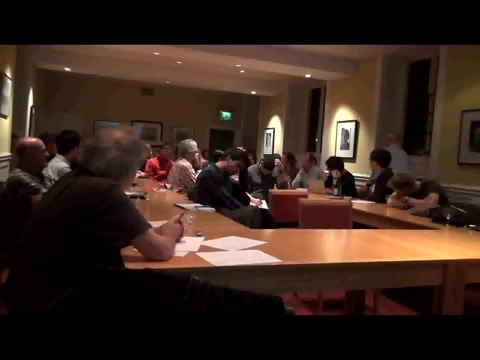 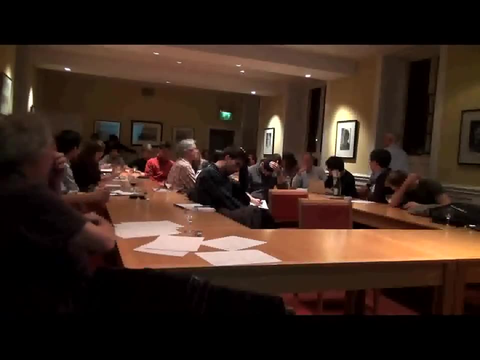 and move further away from the political economy and throw out the ideological, any ideological kind of attempts for economics altogether, Which, you know, given that you're defining the parameters of complex systems and also defining the agents of any economic policies, are perhaps 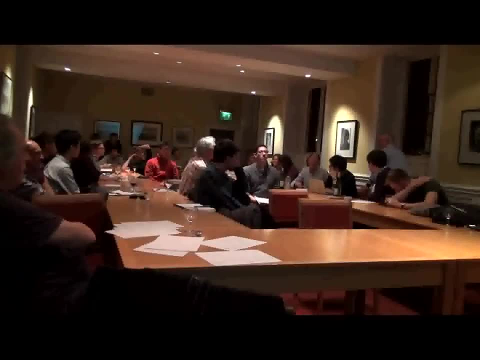 That's another book worth questioning. What I certainly I think, if you look at what neoclassical economics did, it ate the wrong. It ate badly the wrong physics at the wrong time in the development of physics. So what we got was what Phil Murawski describes as energetic. 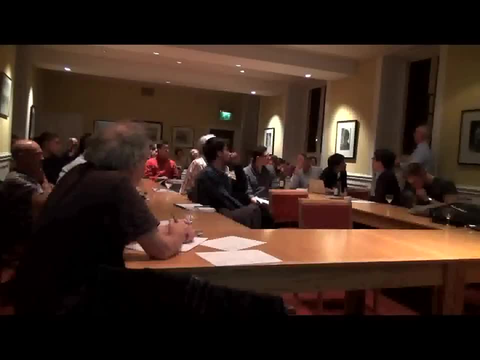 Transferred to economics, which physics itself rejected 20 years later. So we're using an out-of-date pre-thermodynamical theory as the basis of our model of the economy, Reversible processes and all sorts of nonsense like that. So I would rather say: 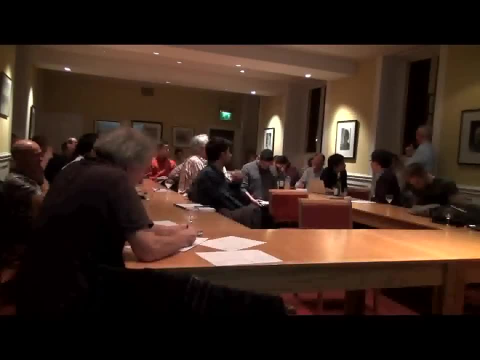 let's catch up with, say, late 19th century physics, rather than the stuff where we are in: the early 17th century stuff or late 17th century stuff. That's not what we actually did, So there is an element of saying. 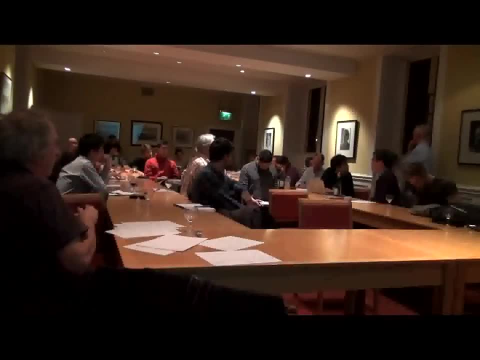 yes, we need to borrow the physics for the progress and actually know what physics is doing. in that sense, We're always going to be political and ideological because certainly, when you come down to saying we have to have a class analysis, which is what I am saying here. 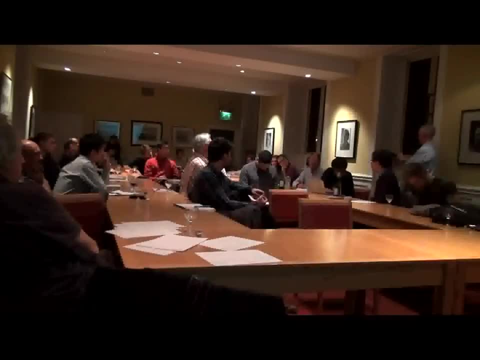 and you then get the result that learning financial capital gets too big screws the working class, which also is a result of these models. The workers actually pay for the debt even though they don't borrow it. Then you end up having a class basis. 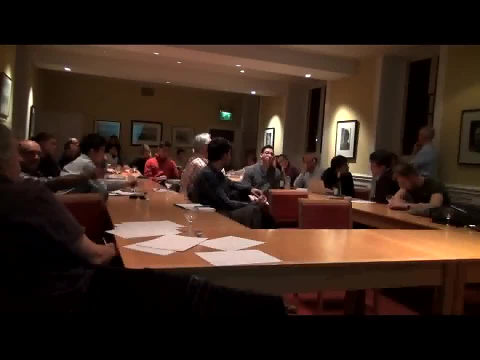 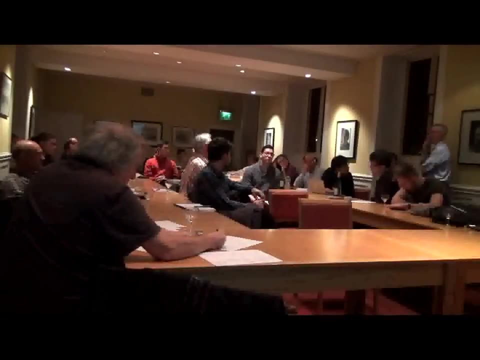 and you've got to say: well, I don't want to see the working class get screwed. I believe we should have redistribution And it becomes a political statement. Equally, I imagine- what's his name, the guy who runs Morgan Stanley? 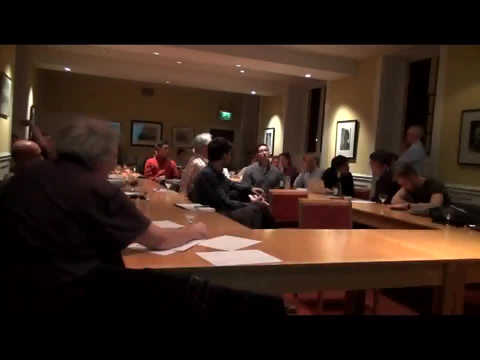 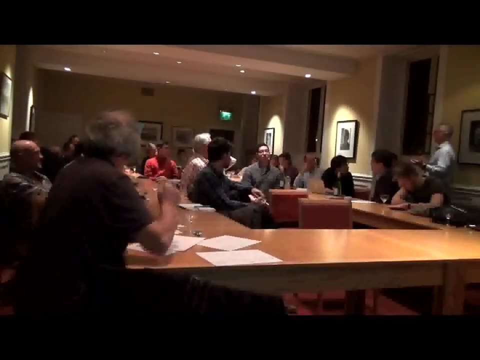 might be very happy to say: let's screw the workers. So you come down to the politics being explicit rather than hidden in the assumptions of the model. But if you think about the neoclassical model, everything is in equilibrium. Markets work perfectly without government intervention. 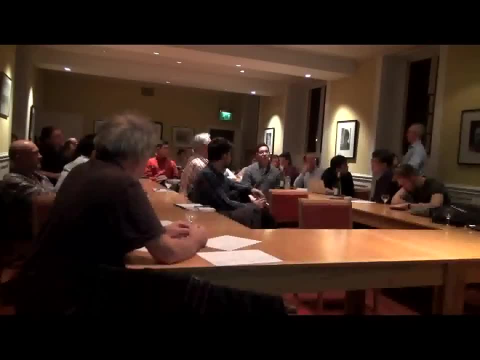 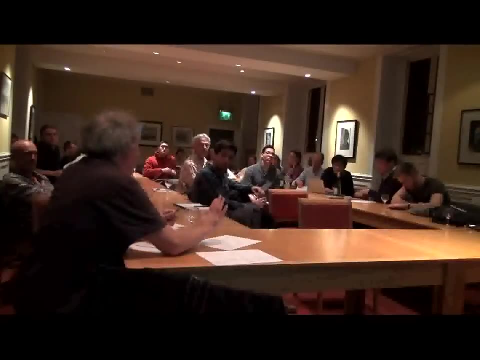 et cetera, et cetera. The ideology is buried in the assumptions itself. Or answer your question. Time has gone very fast. We're not finished quite, but perhaps, if there are any- I know there's Clive and Patrick- 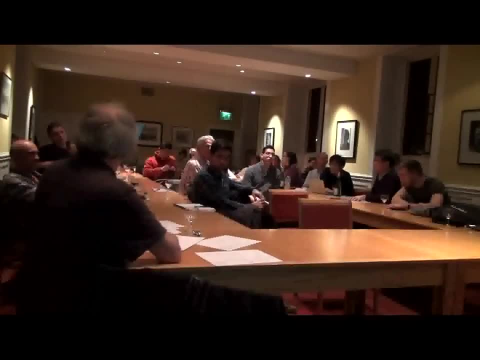 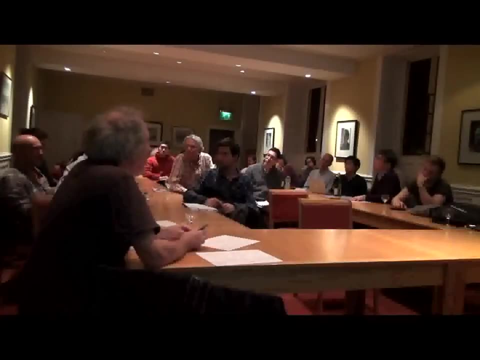 any other questions? Can you take a set of questions and then we'll come back to all of them? Yes, just to follow on from the last question, really, If it's the case that economics has got it wrong because it took the wrong bits of physics, 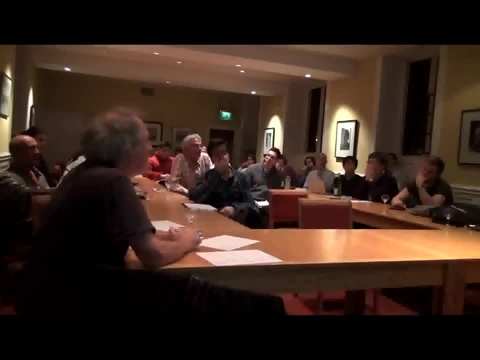 at the wrong time and came back. I think it's more the teleology that did that as well. Right, But is it is your belief, ultimately, that there's kind of no real difference between physical systems and human systems? Oh God, no. 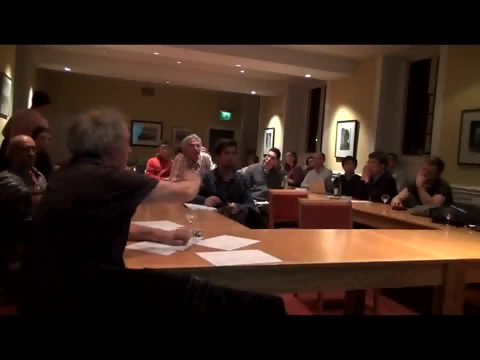 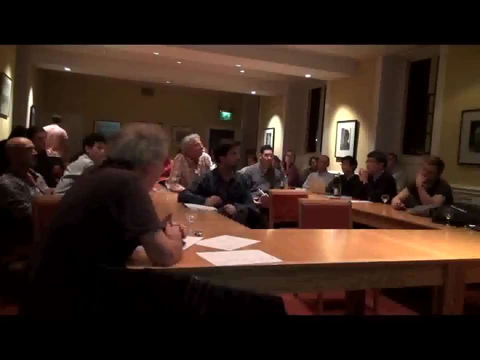 Well, in that case, what are the differences? Well, again, Give me one way: Yeah, Okay, Human decision. Yeah, yeah, Yeah, all right, Go on, Yeah, Human decision. But again I say, the human decision is constrained. 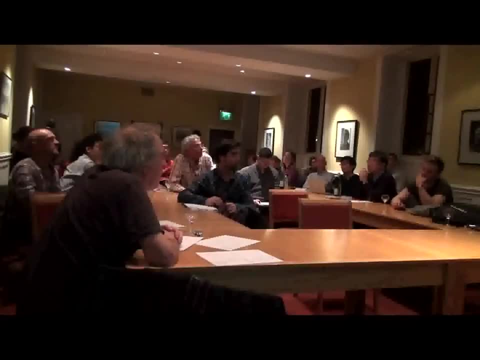 by the social systems in which we live. So I want to model the constraints and then say a human agency will mean I'll be wrong about you know where we fit inside the constraints, whether we occasionally break them, But you're still monitoring the overall constraints. 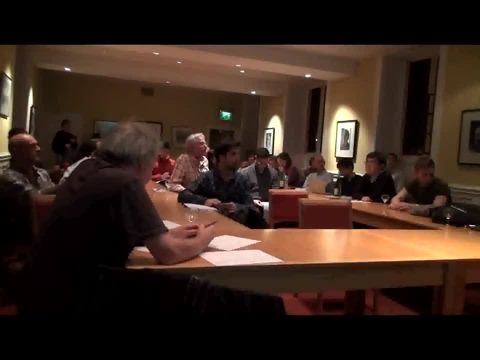 And that's where rules of thumb about behavior can actually be fairly accurate description of what people do at a collective level. But certainly you can't. you know my George Bush and the Haynes Chad's example. you know the tiniest event. 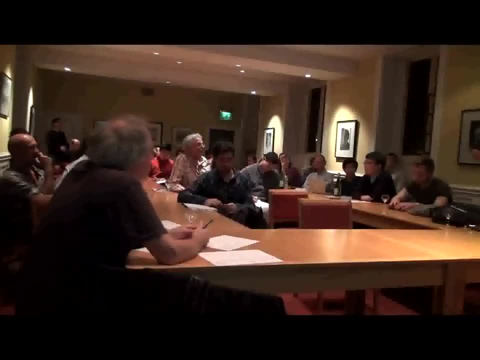 that could have made the hugest change to human history in the last 15 years. And you can't capture that, You can't pick it. you know those sorts of things can't be modeled, But you can model the overall parameters and we would have had 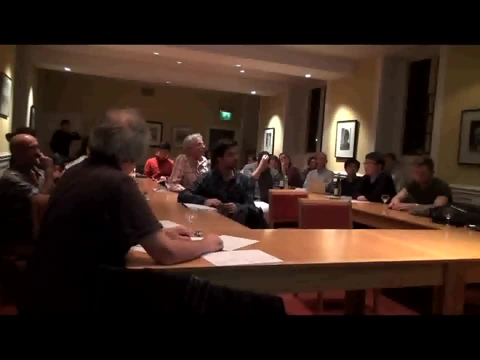 you know, the hanging chance occurred at the time of the dot-com bubble. So there's no way mathematics can model everything- No way. You've got to have modesty about it. You've got to do what you can't model and what you can't prove. 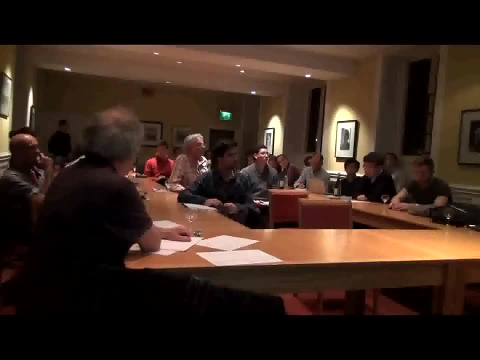 And mathematicians are aware of that. So in some ways, by being more mathematical, you're also then being more modest in your classical. So I think they can prove everything. I mean I guess, well, am I allowed to come back? 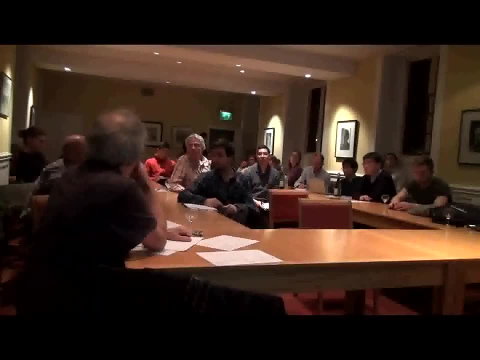 Go on quickly. The thing that bothers me about science and human systems is not so much the possibility of complexity or being very, very sensitive to starting points. It's this kind of linkage along the way, It's the way that one statement or idea 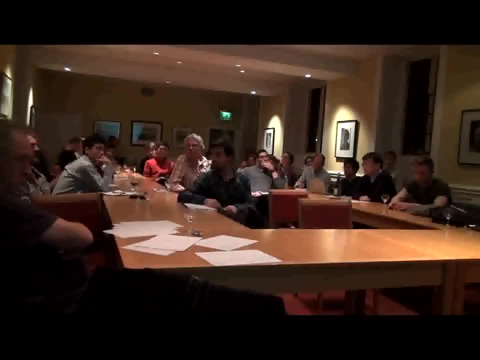 links to another or one proposition links to another one when it's open to meaning and you know getting it wrong and all this sort of stuff. But it's not clear. I mean, I still haven't got clear in my own head how maths helps us with that. 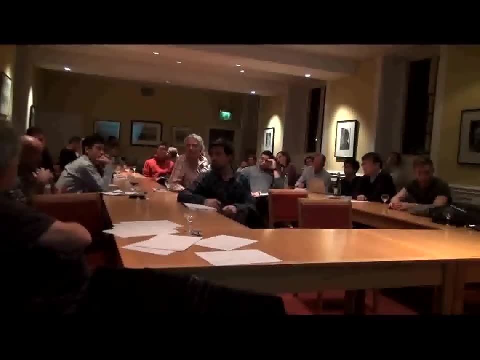 because maths helps us to link things in well, I don't know whose conception of atomistic is going on here, but you know in the sense that the link means the same thing does the same thing under the same circumstances, and you know. 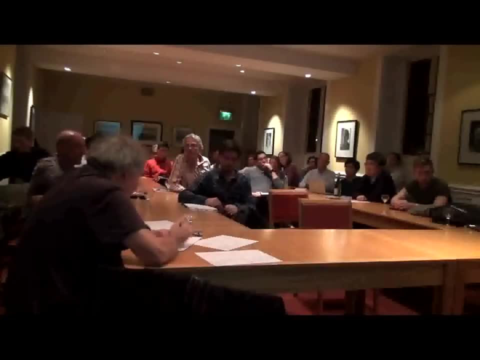 you can build an incredibly complex way of that, the way that that fires up and so on, but the basic linking from proposition to proposition sort of has to be atomistic and in physical systems. that makes sense to me, because, well, it doesn't make sense to me. 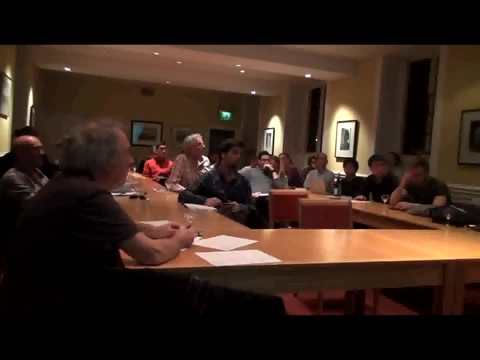 but it does seem to be the fact that there seems to be, I don't want to say the role it has in evolution. I mean, we know that evolution is a quantum mechanical process. that doesn't mean and we know we can't predict what organisms. 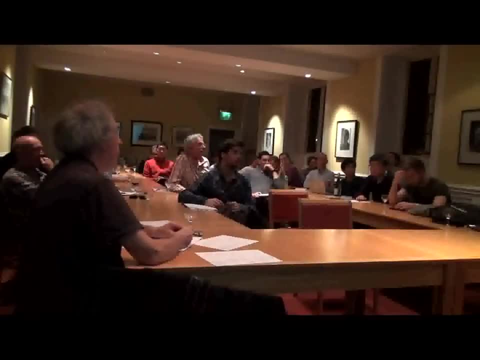 are going to happen in the future. it doesn't mean evolution didn't happen. so you tend to say no mathematical biologist is going to try to predict future organisms. but any mathematical biologist is going to say we have to capture the occurrence of occasional mass extinction events. 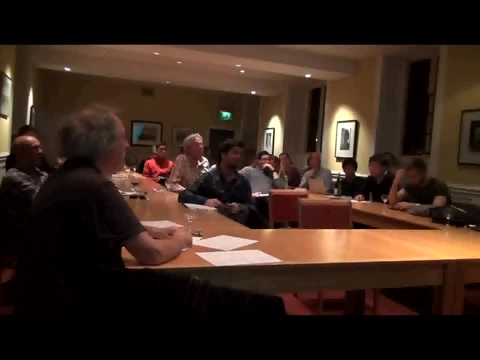 Yeah, but a lot of that mechanism seems to be extinction. You know you have to, but it's doing a qualitative description. that you're trying to do, that's generally right, but you will not reproduce exactly what has happened in the past, let alone predict. 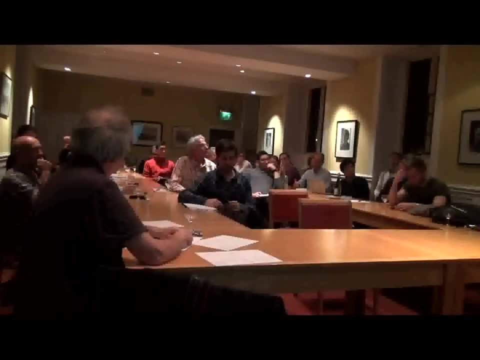 the future, but it's getting the qualitative characteristics right. and then, for example, there's an interesting work on what's called the Tracy-Wygon distribution right now, which is a model of what happens with interacting populations, and that model predicts that, if you have 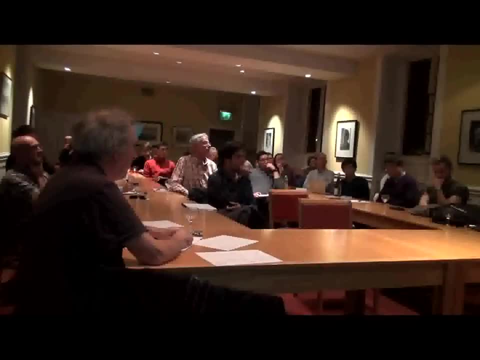 too much interaction between an isolated species and a set of islands, then what will happen is that you're going to have one population and ultimately one population will wipe out all the others. but if you have a lower level of interaction, those populations can coexist and evolve. 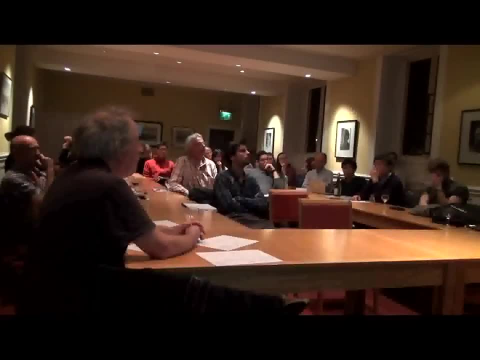 and those type of elements are what you're trying to capture in your modelling. rather than predicting what the future evolution is going to lead to, You're trying to capture what you've seen happen in the past and qualitatively describe the system and then, out of that, 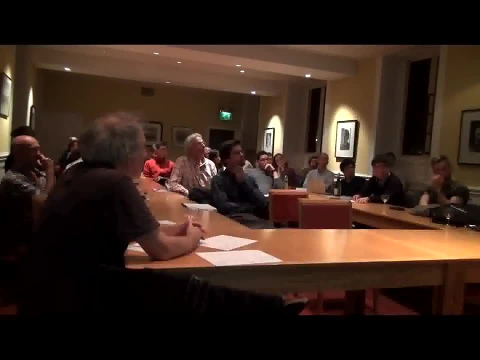 you might say if we want different populations of finches to continue surviving in the islands below a certain threshold, that sort of thing, but not saying you know that we can predict what the next finch is going to look like. Sure, I'll hop back. 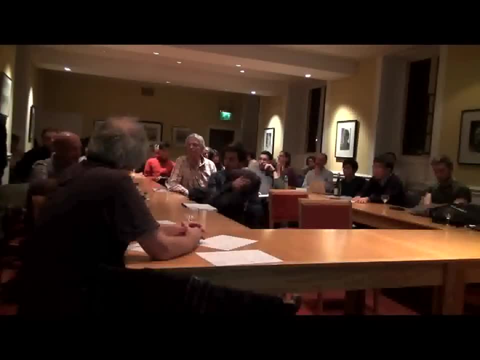 Prediction panels go, step backwards. you know, take back, move back from the prediction at the end, which you're right, then you kind of say, but how do we get to the link before the link, before the prediction? I mean this sort of link, link, link, and they're atomistic. 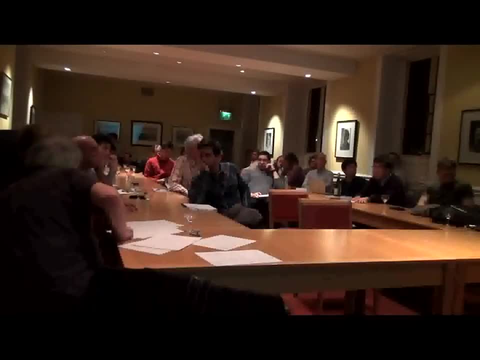 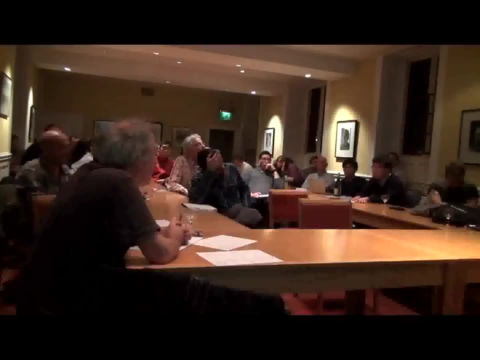 I still want to say at the end: it's organic, not atomistic. but the main thing I'm trying to explain is: why does capitalism have great depressions and is it possible to avoid them? okay, and what insights do we need? that's really as far as I need. 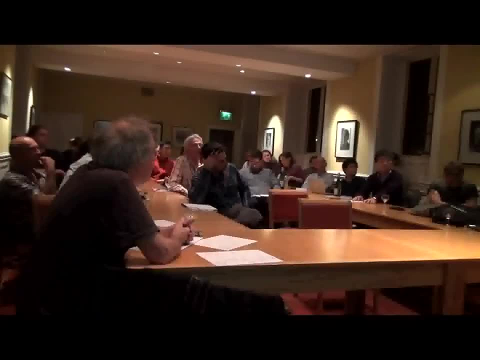 I don't want to predict what Elon Musk is going to invent tomorrow. you know I'm not trying to get. you don't need that level of precision. I simply want to get a social system which doesn't have great depressions, which doesn't lead to a miserization. 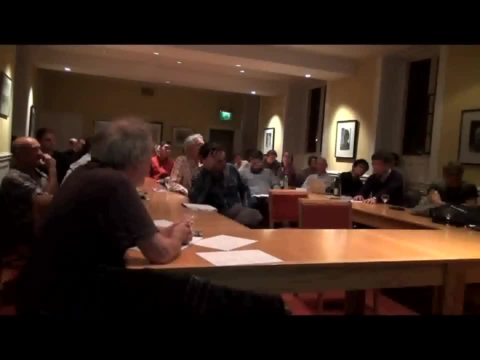 of the working class and we've got both right now. so it's really I think I'll stop there. I think I'm probably not okay. I think I mean, as always, at the end everyone's putting their hands up. I'm afraid we've come. can you stay? 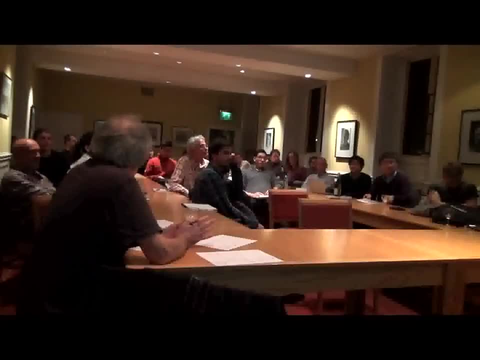 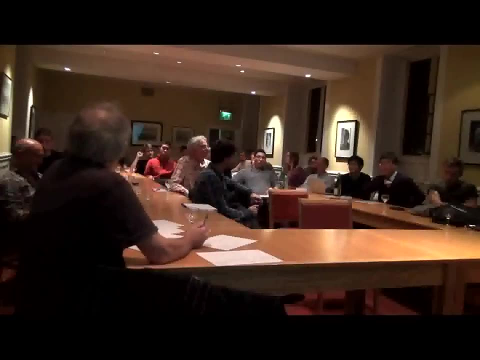 for a bit depends what time the next train is back to London. they'll only get back before too late in the morning. I'm sure everyone someone's got an app that can find you a train. well, I think I must draw it to an end because it's very kind. 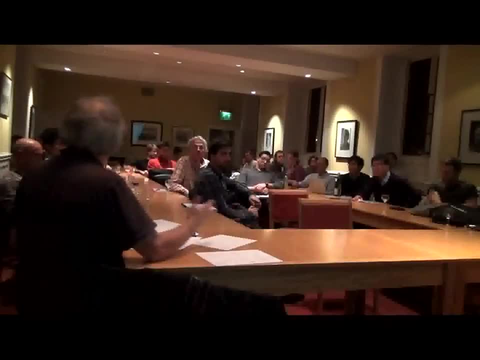 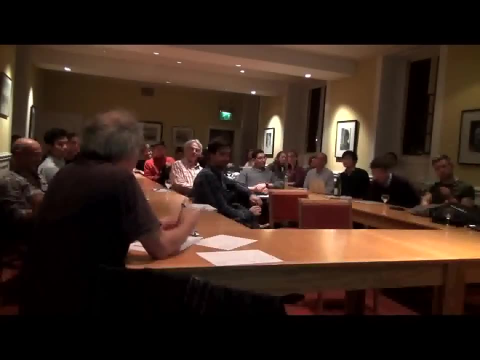 of Steve to come here and talk to us on this topic, knowing how much we would all agree with it. and in two weeks time you've got another speaker and I forgot on who it is. it's on the website, but people are welcome now to stay and if there's any, 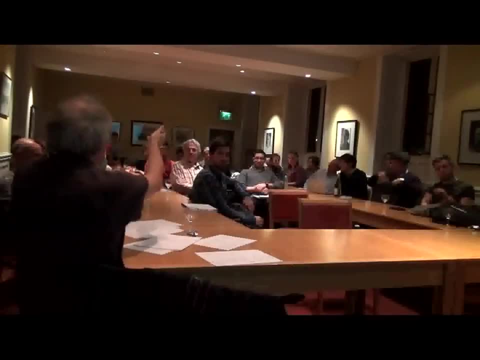 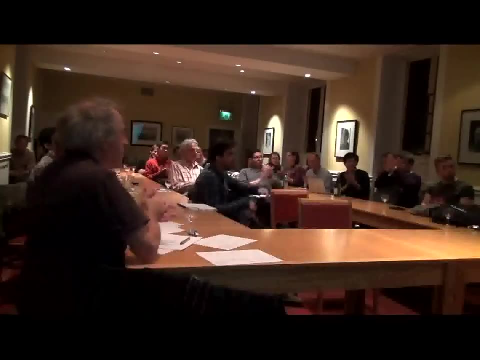 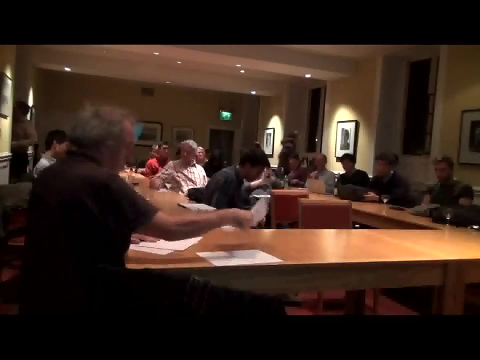 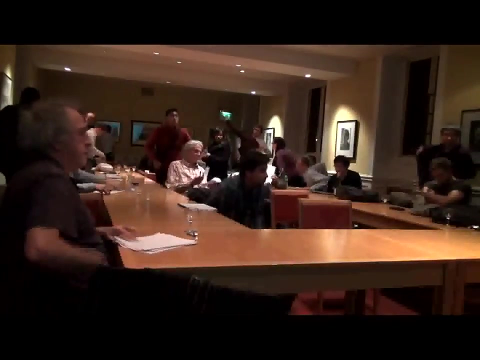 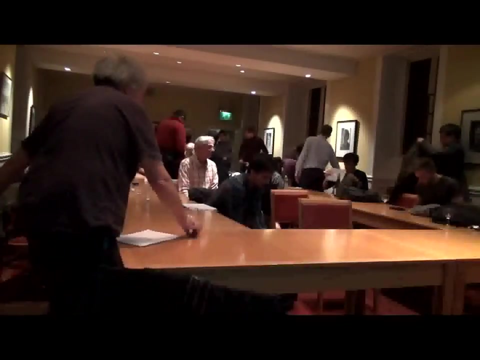 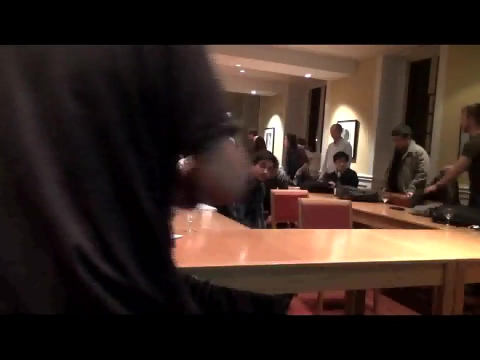 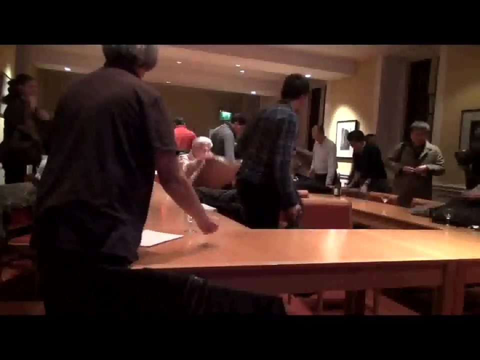 drink left at the back to drink and carry on the conversation. but let's show our appreciation to Steve for inviting you. thank you where you going, Kingsborough? thank you, that's pretty similar, Mary. Mary. Steve, I can cut through. Can I have the wire? Thanks, bro. 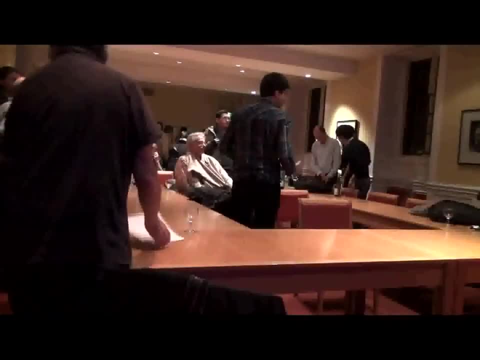 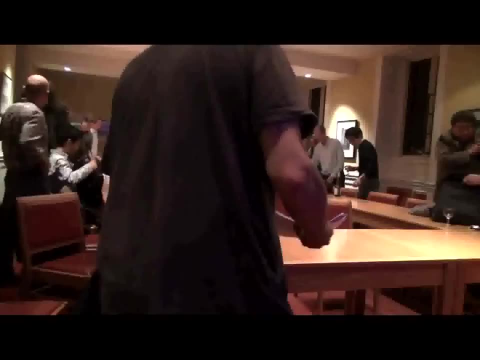 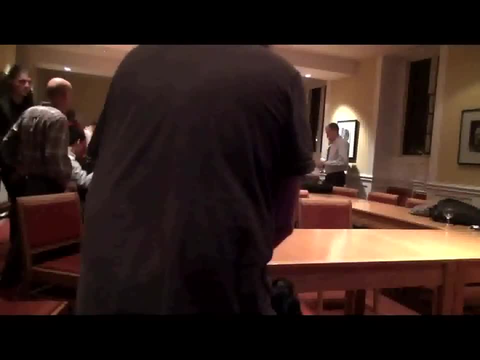 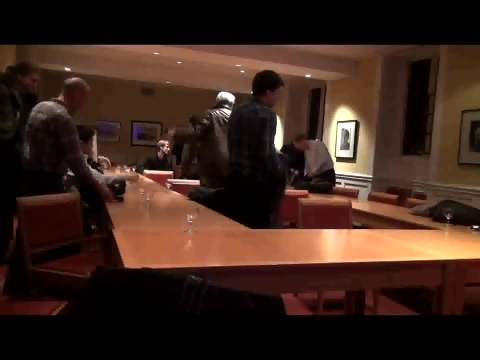 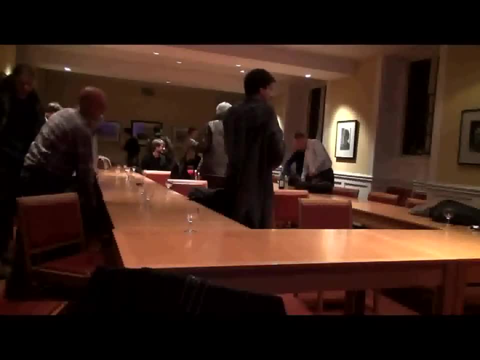 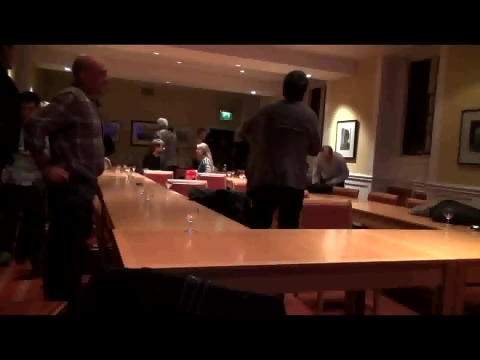 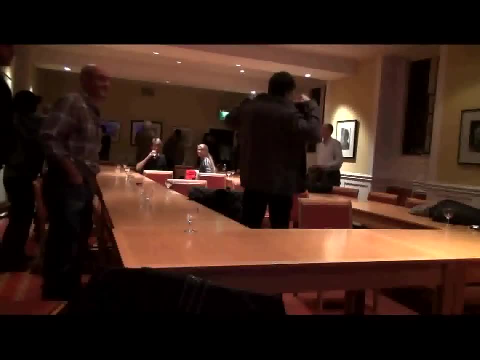 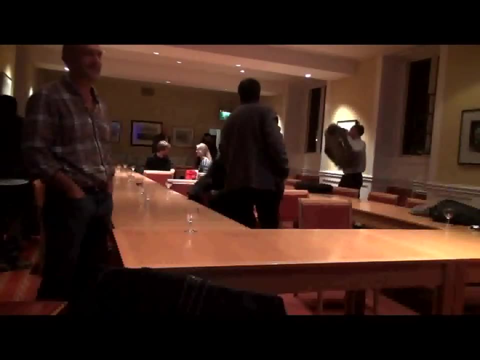 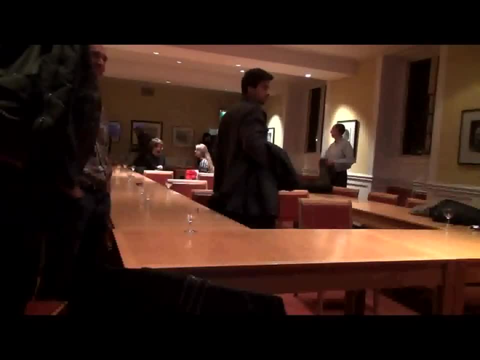 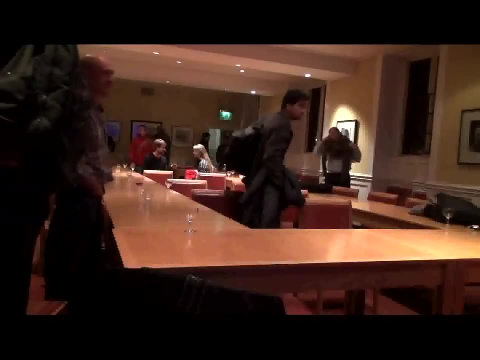 Oh yeah, I know in his final years he was quite a worthy working father to me. now, now, All the stuff I teach mathematics in, I teach mathematics in. All the stuff I teach mathematics in, I teach mathematics in. 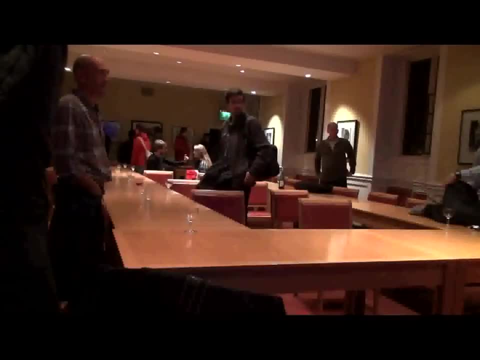 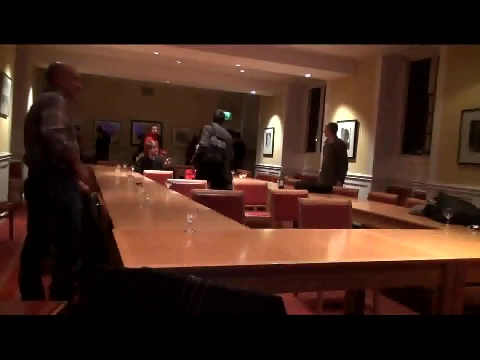 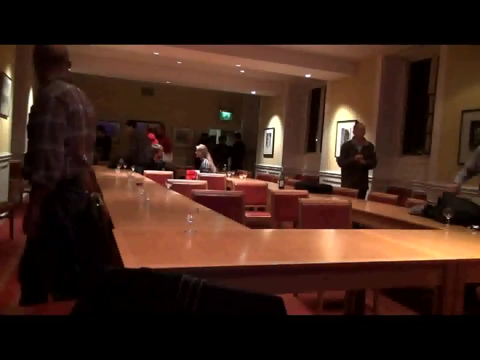 You've read his mathematical notes, haven't you? Even that has done proof of differentiation. yeah, Oh, no, I mean it's not hard. My hearing is bad, sorry, No, that's not really, No, no, I just want to know. 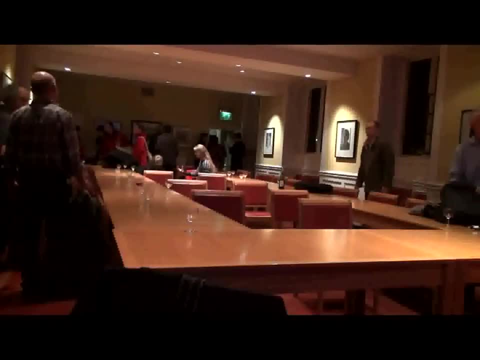 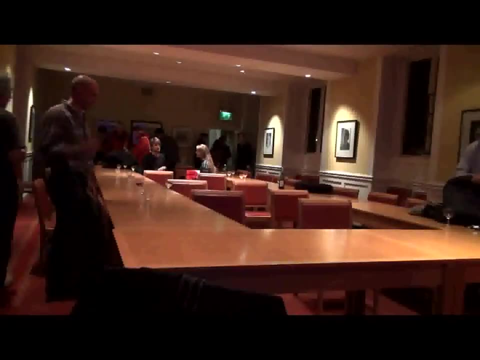 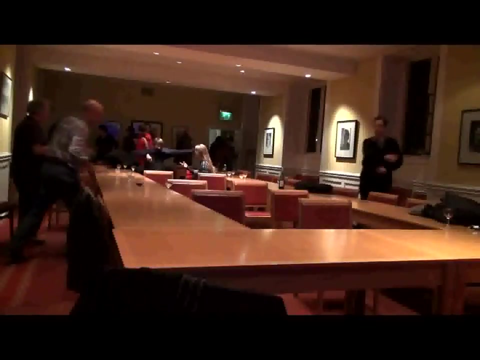 Yeah, no, no, I just want to know. Yeah, that was funny- You asked a question about economics because all the economics were there And the lawyers against him so much. how do you? It's terrifying, Yeah, Yeah. 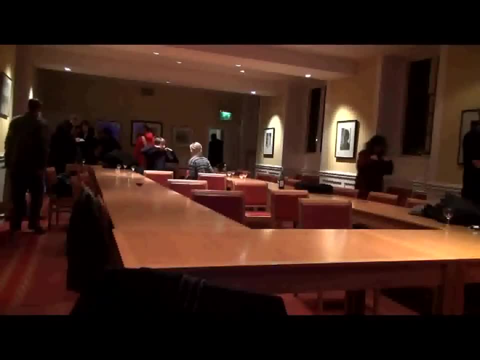 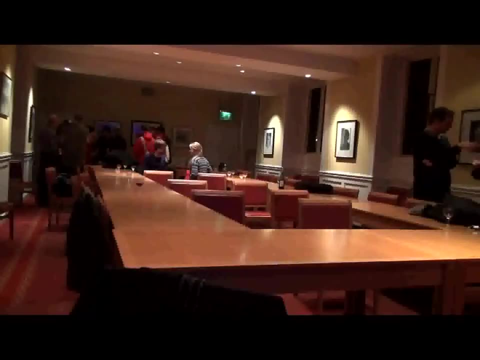 And I applied to the department of philosophy, where I was a graduate student. and I applied to the department of philosophy where I was a graduate student. I was required to get my degree at the faculty of English and I didn't get it. I was required to get my degree at the faculty of English and I wouldn't be able to do it. 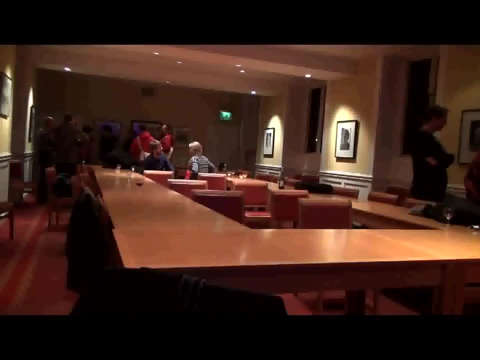 because my English wasn't so good, so I was between like math and physics, and I didn't, and I didn't even know what I was trying to learn about. Even though I got the degree, I still didn't get enough. Now, I was never old at all. 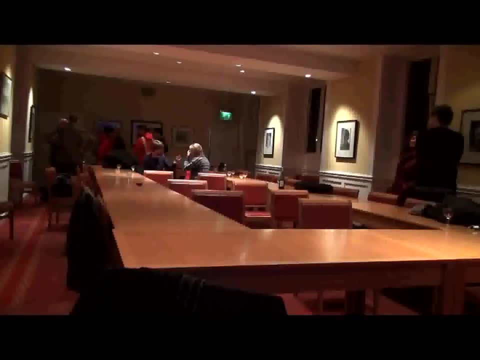 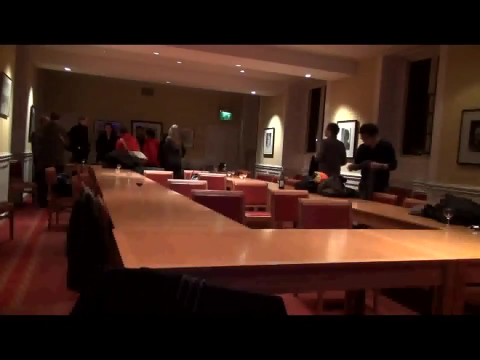 No, no, I didn't. What do you think about it? What do you think about it? Okay, Okay, I want to make sure that There's a camera running. Pardon me, Yep, yep, yep.